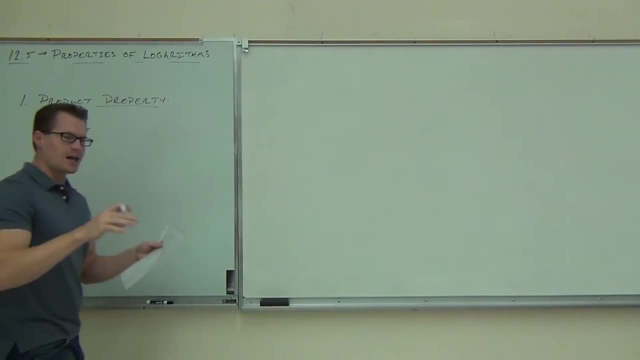 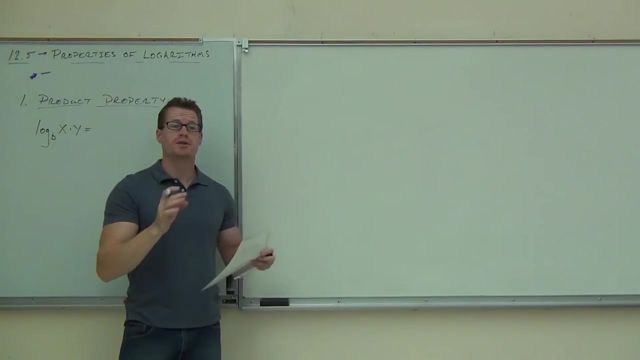 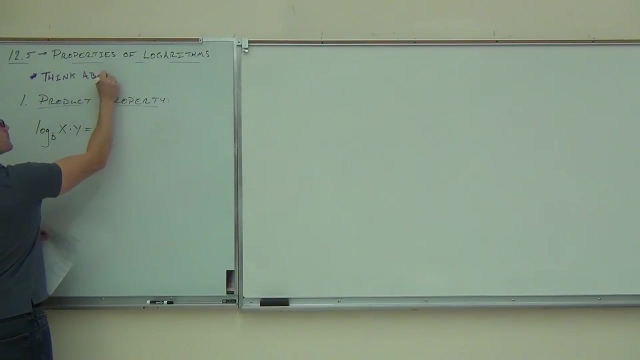 easier for you. So a little note for you: think about these like exponent rules. Are they exactly the same? No, otherwise they would just be exponents, But they're very, very similar. The first one we're going to talk about is called the product property. It says: let's. 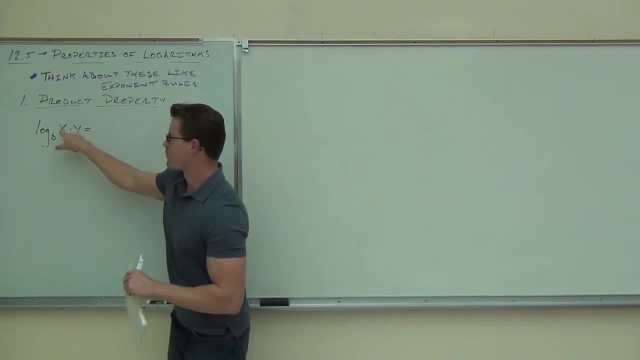 suppose you've got a logarithm and inside you have some sort of product, so things are being multiplied. Now I'm going to relate these each time to an exponent rule that you guys already covered. that's what going to make it kind of nice for you. 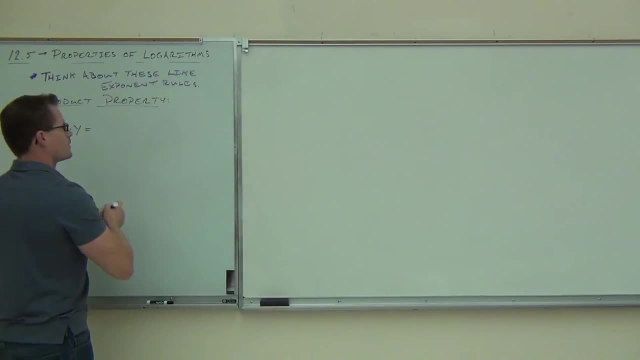 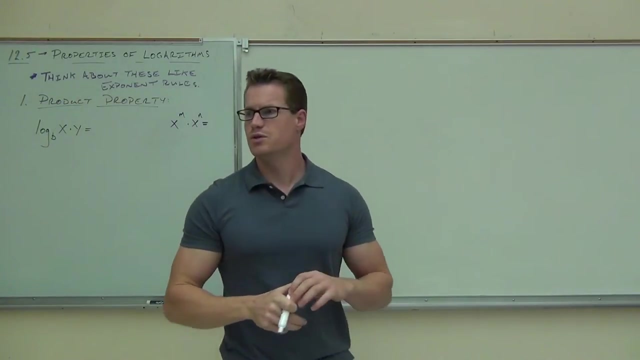 So the thing I have to relate it is, is this: What would you do if you had X to the X to the M times, X to the N? What would you do to those exponents? Would you multiply them? You would add them. 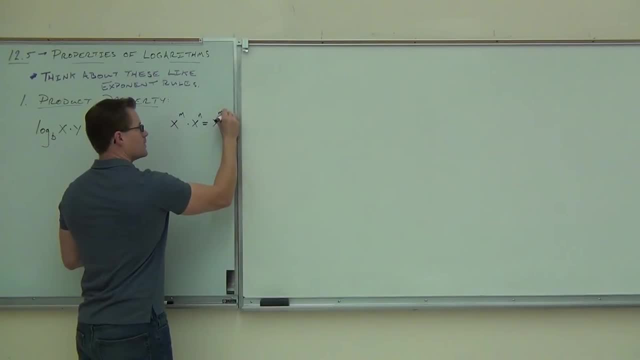 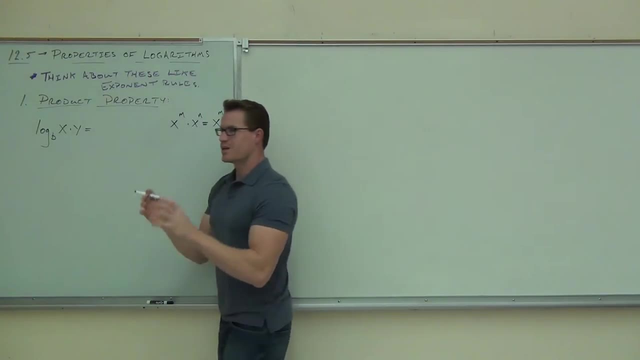 Right. So this is X to the M plus N Agree. Here's the relation between this right here and our logarithms. It works. It's a very similar situation, except, remember, we're splitting up these exponents right now, So it's going to work a little bit different than our exponents. 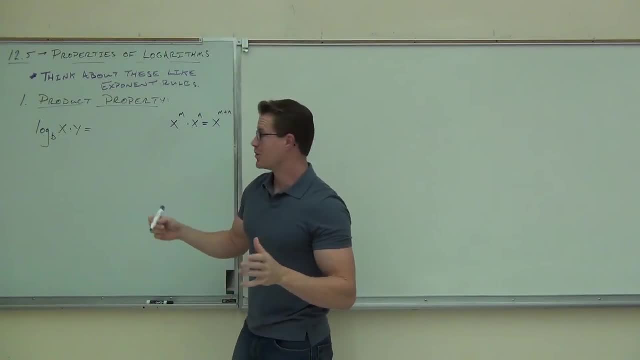 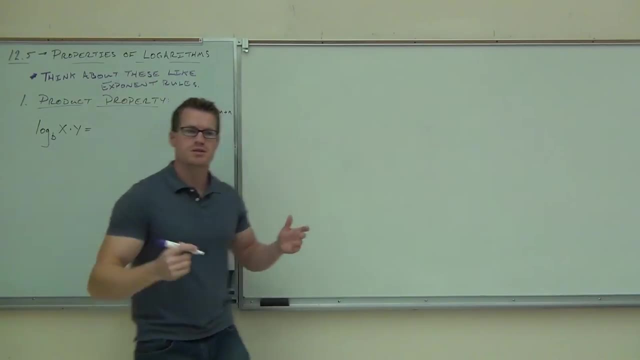 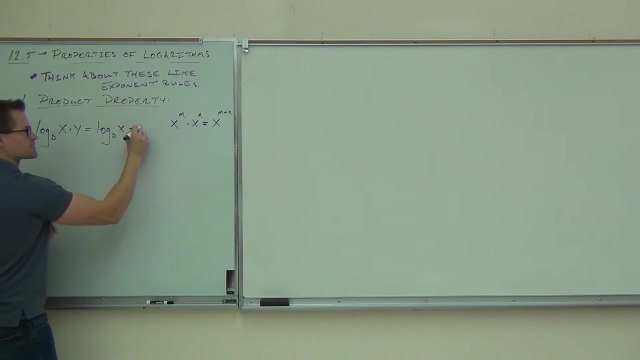 Otherwise we would just have exponents. but check this out: It's kind of cool If you have a product inside your logarithm, or in this instance, log base B of X times Y. this comes down to if we would add exponents together, we're now going to add logarithms together. 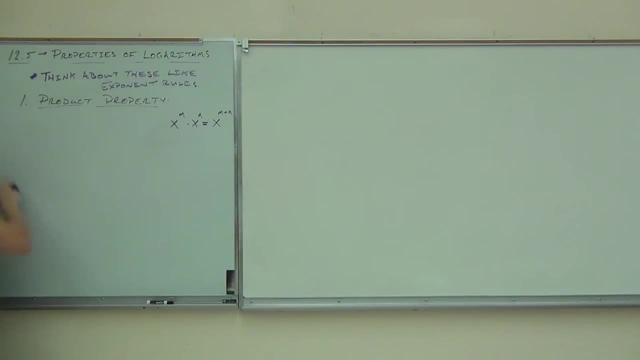 I'm going to move this a little bit lower so you can see it better. Log base B of X plus log base B of Y- That's a product rule. Is it similar to the exponent rule for you? It says if you're going to multiply common bases, you're going to add the exponents together. 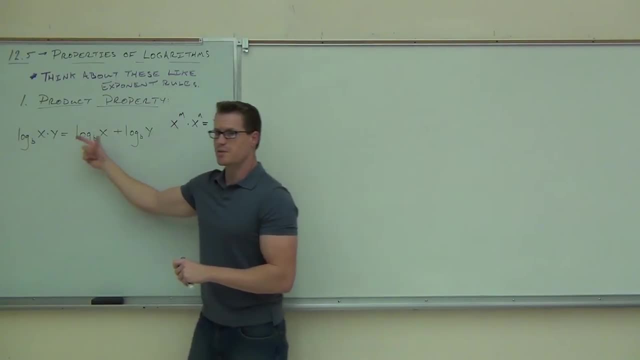 That's what this says. It says, if you're going to multiply these things, you're going to be adding those logarithms together, So you can therefore split up logarithms. You can split up logarithms. You can split up logarithms or you can combine logarithms. 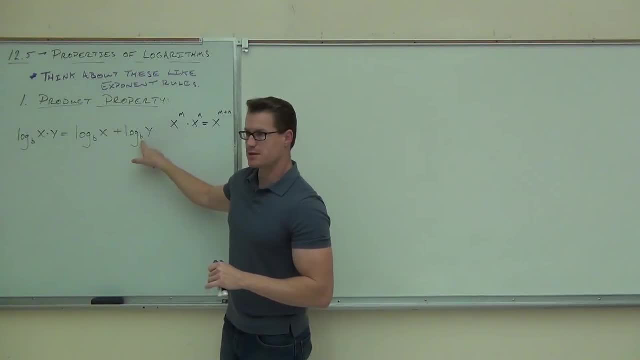 The only thing you've got to look for is if these things have a common base. They've got to have the same base because you're going to make one logarithm out of it. So these are not just one-way streets. It's not that you can always just split it up. 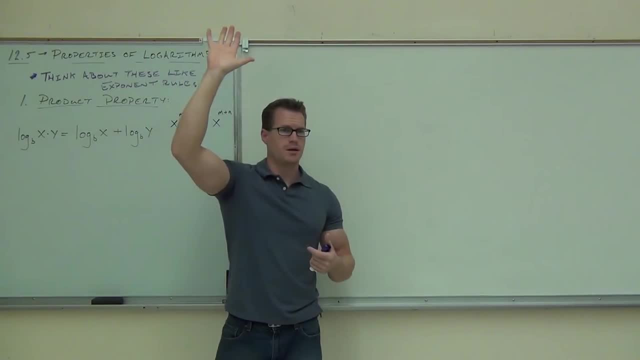 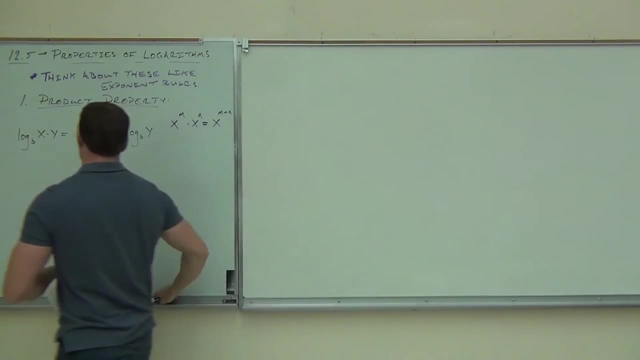 You can also put it together. How many of you feel okay with that? So if you think about them like exponent rules, it's going to at least give you a little foothold there. Now let's try a couple of examples, just to get our feet wet on this stuff. 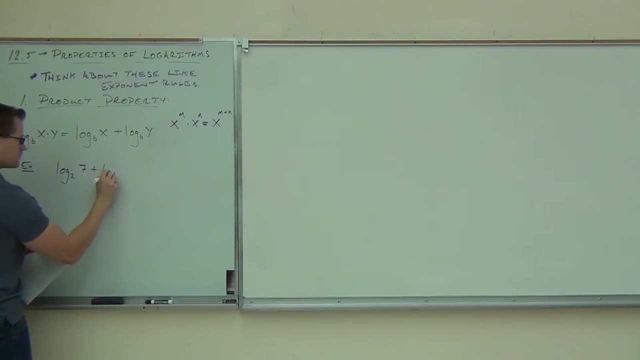 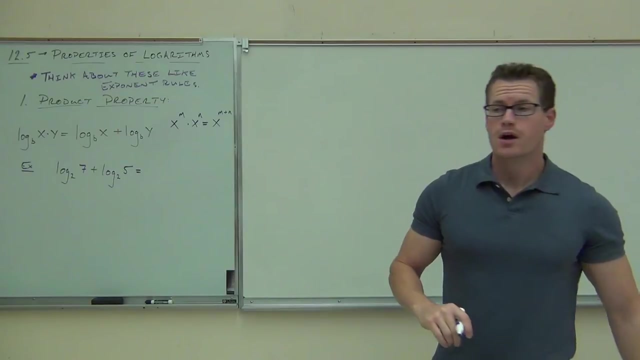 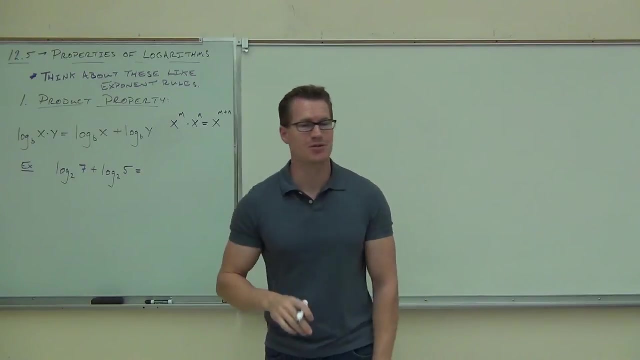 Okay, so I have log base 2 of 7 plus log base 2 of 5.. First question is: am I going to get log base 2 of 12?? No, No, They're not addable. You can't add logarithms. 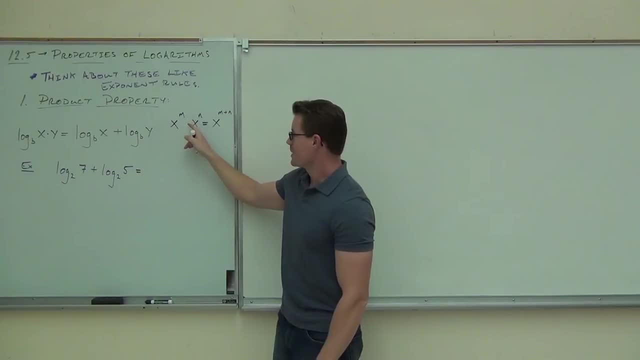 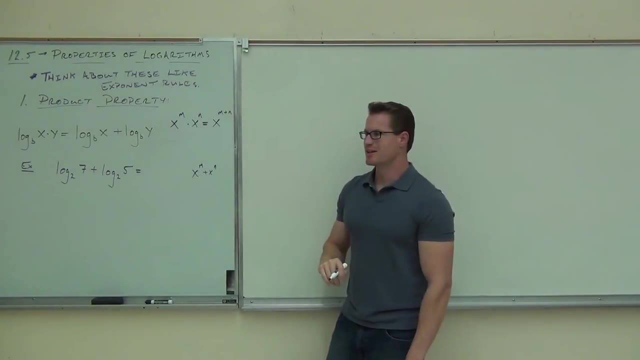 It's like doing this, You can't- just I'm sorry You can't. You can't combine those by addition, can you? You can't add those, You can add those ones. So when we're putting these things together, you don't add them. 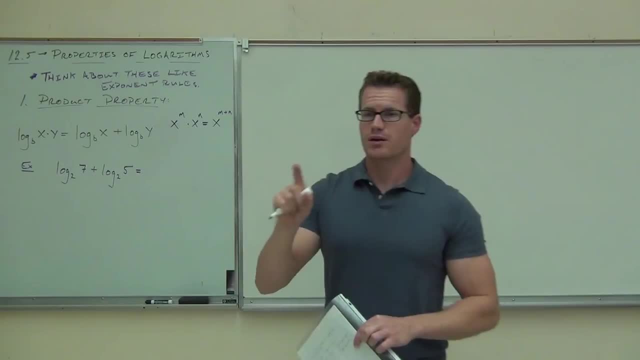 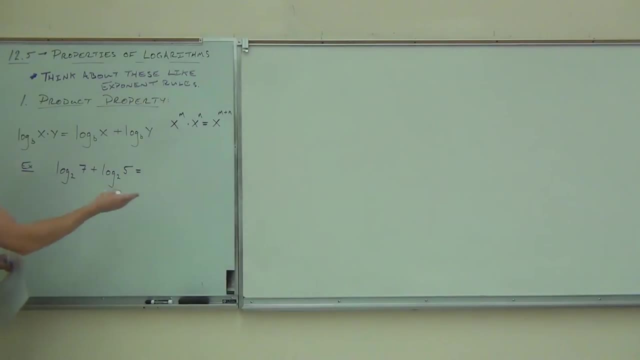 You actually multiply them. You have to use that product property Firstly, can you put them together? Do you have the same base, in other words? So that's important. You've got to check for that, Otherwise you wouldn't know what base to make your logarithm. 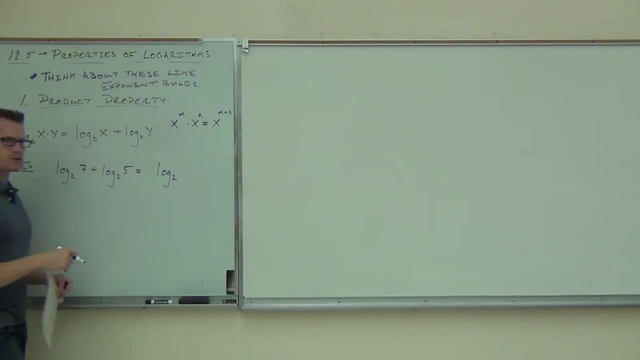 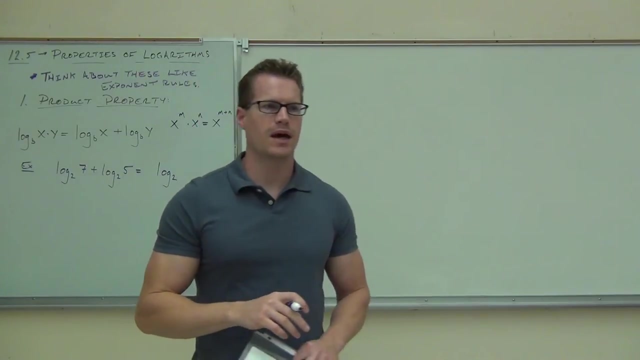 So of course we know we're going to get one logarithm out of this log base 2.. Inside that log base 2, what are we going to have? What are we going to have, Or how do you find it? Are we going to add them? 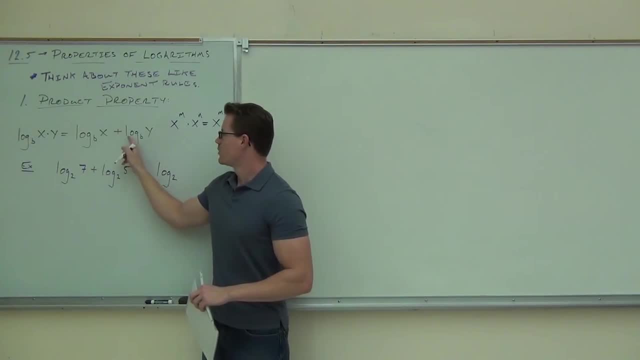 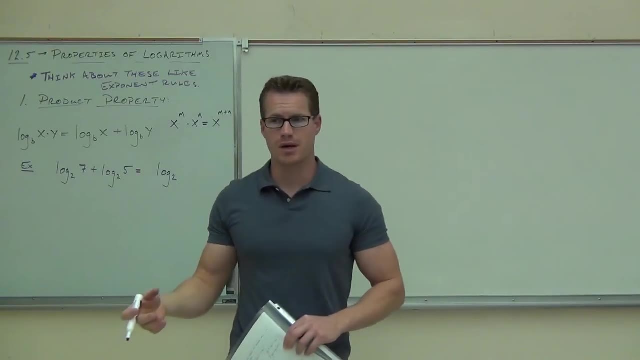 What's it say? If I'm adding these two logarithms, what do I have to do to the numbers inside? You've got to multiply them. So what the product property says is: if you're going to add two logarithms to the same base. 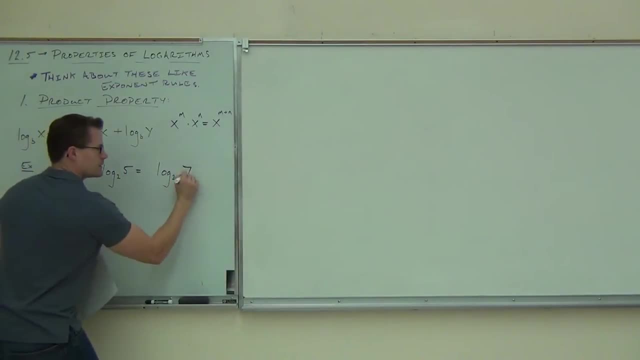 what you end up doing is multiplying the insides of your logarithms. Do you see how this property is this property? right here? It says: if you're adding logarithms, you're going to be multiplying the insides. It's kind of going this way. 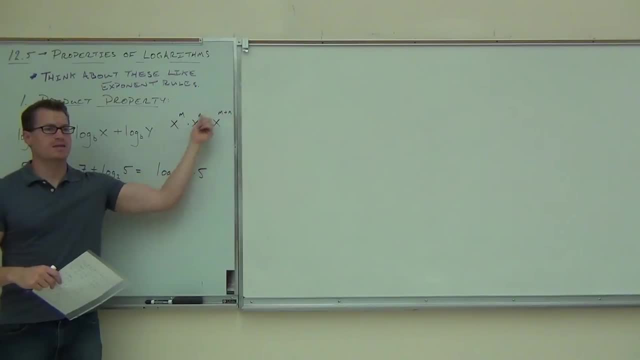 It's kind of going that way. It says if you have exponents being added together, you could split that up by a multiplication. It's possible. You can do that, You guys. okay with that one, All right, How about that? 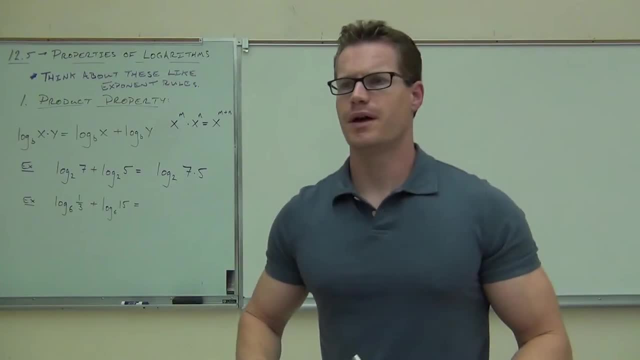 How about that? First thing? Could you combine these two logarithms? Is that possible in this case? Why Great? This is the same And we're adding together. We have a property for that. It says: if you have two logarithms of the same base being added together, all you've got. 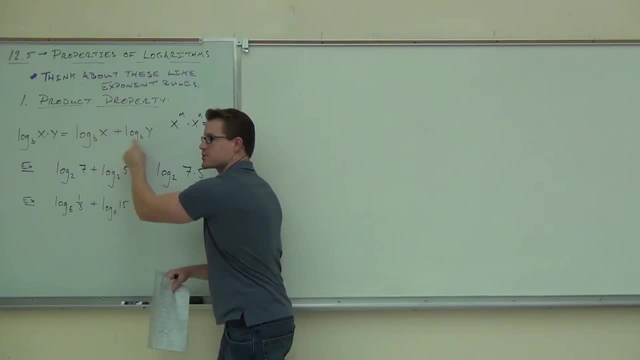 to do is look at the inside of your logarithm. there, What are you going to do? Are you going to add one third plus 15, or are you going to multiply one third times 15? One third, Sure, That's what the product property says. 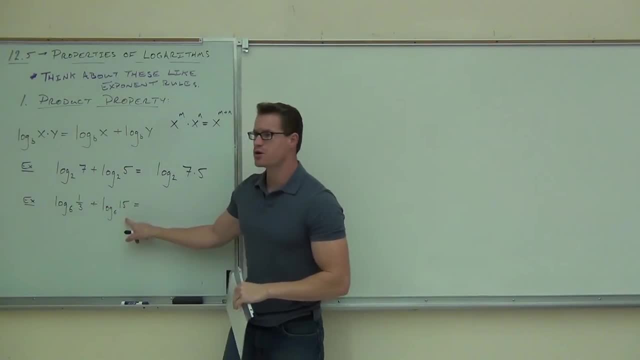 That's why it's called the product property right. It says: if you're adding two things together, you're going to be multiplying one third plus 15.. That's what the product property says. That's why it's called the product property right. 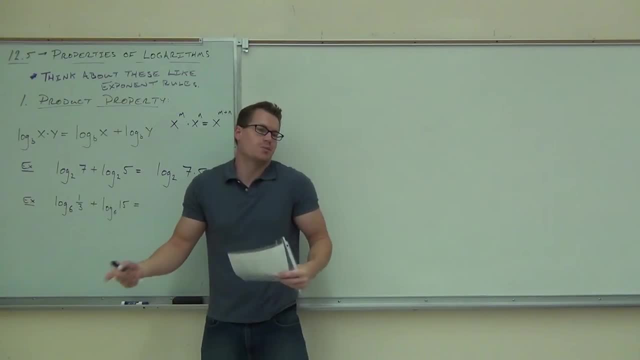 It says: if you're adding two things together, you're going to multiply the inside of those logarithms: Product plus, Product plus or plus product. The two P's go together. So tell me exactly what I'm going to write out here, please. 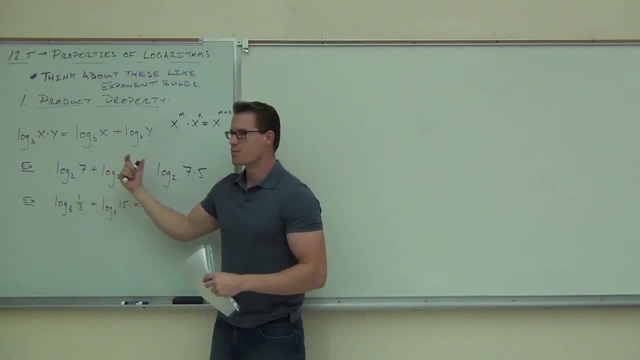 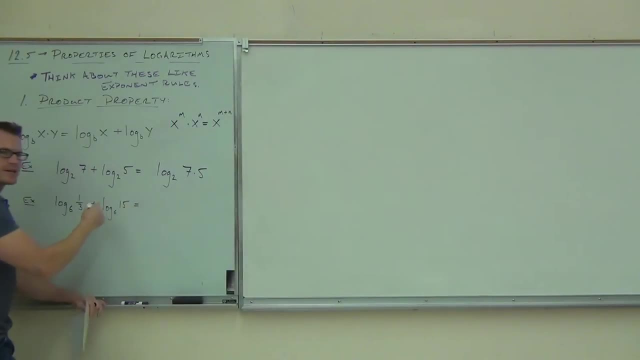 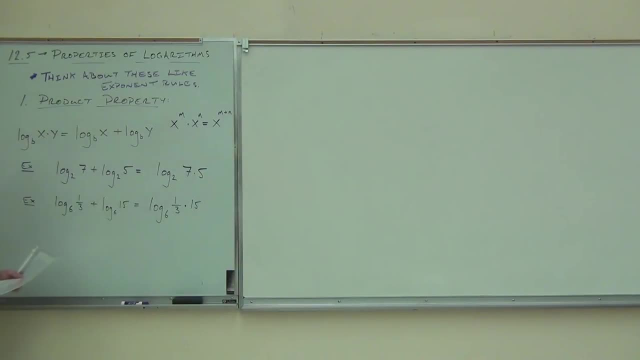 Times, Times, Times, Times. Yeah, exactly right, You simplified to five times. Yeah, you know what You could simplify If we have log base 6 of one third times 15, you can do the operation just like we did. 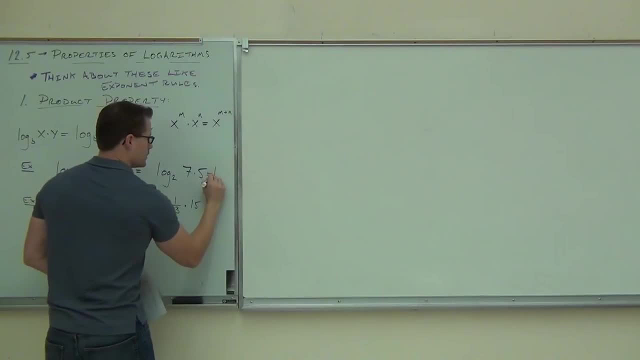 seven times 5. right here You could get log base 2 of 35. That's perfectly reasonable. What can we get here? Log base 6 of what Five? Sure, You can do the one third times of 15.. 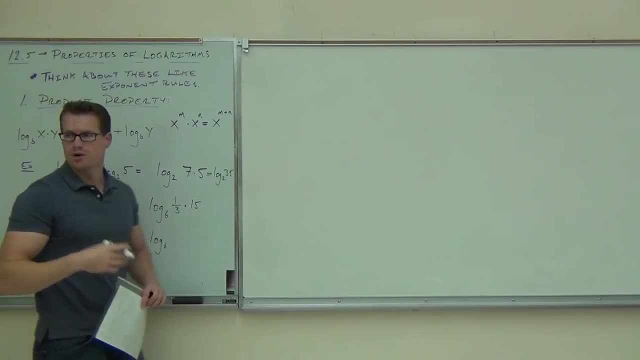 That's okay. You can do the 7 times the 5.. I'm just showing you these steps so you know where those numbers are coming from In our case. here we have our two logarithms being added together. we're gonna be multiplying the seven times the five. 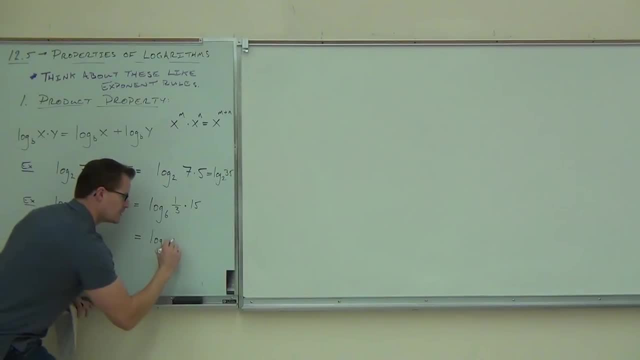 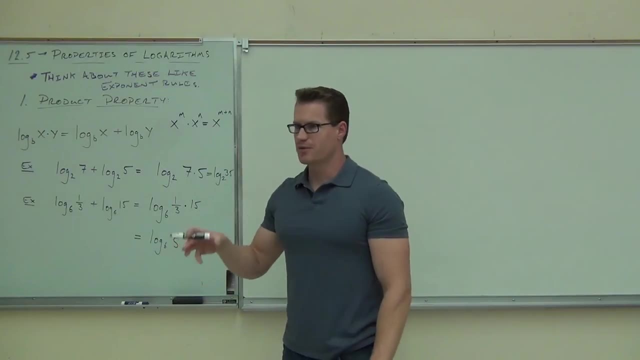 and getting 35.. We're gonna be multiplying the 1 3rd times the 15 and getting five out of that Log base. six of five. That's one way that people back in the day were able to simplify some of these problems, right. 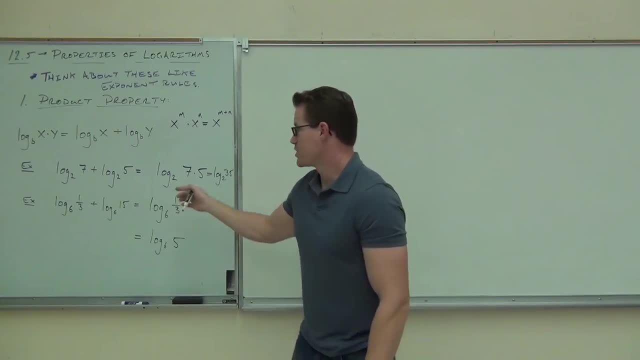 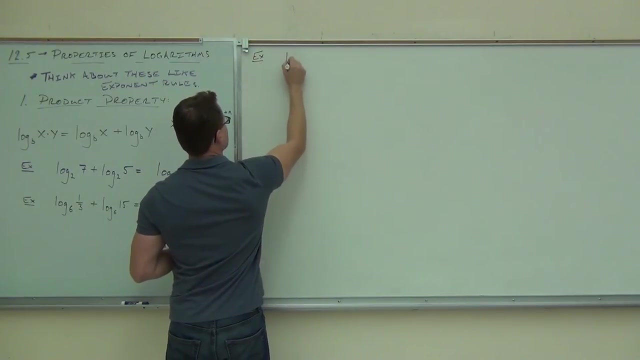 If you knew you could add logarithms together. by multiplying the insides, you change two logarithms into one logarithm. Not too bad, Too shabby. Let's try one more and then we'll continue on. All right guys, let's look at that one. 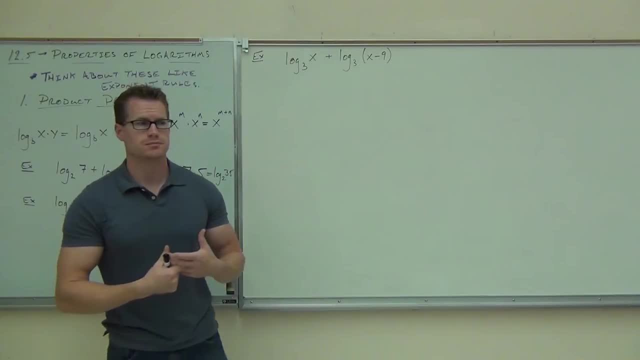 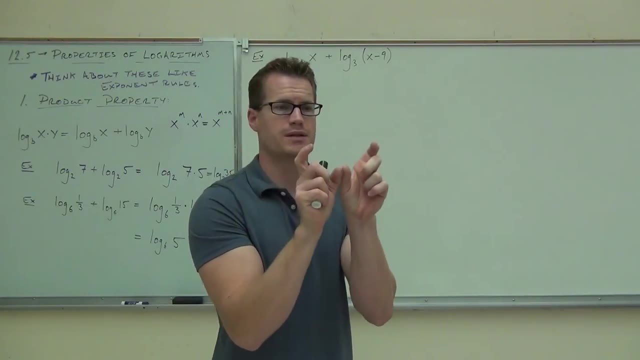 Is it possible to combine these two logarithms? What do you think? Yes, Yeah, what lets you know that again, Radix? Okay, now am I going to be adding these insides of my logarithms or multiplying the insides of my logarithms? 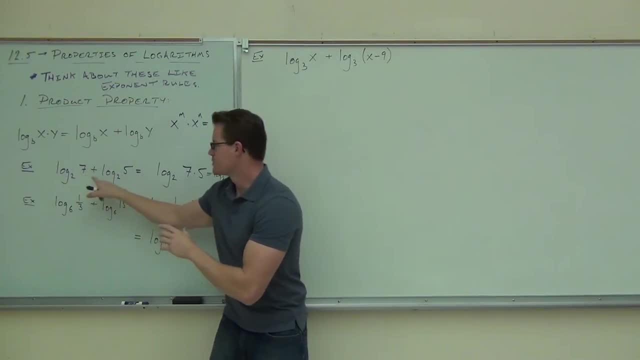 Multiplying. Just like here and here, if you ever have two logarithms of the same base and you're adding them together, you can combine them as one logarithm, provided you multiply the insides of your logs. So in our case, right here, 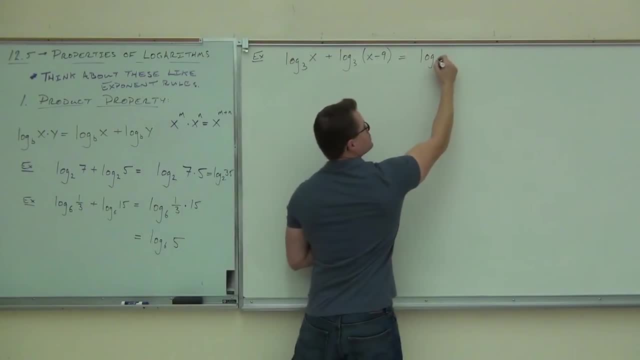 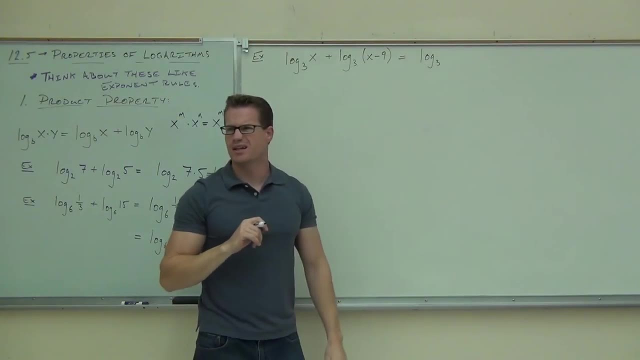 we know this is gonna be log base three. Two logarithms change to a single logarithm. We have one log base three now Only on the inside of our logarithm. we're gonna have what? What are we gonna get out of here? 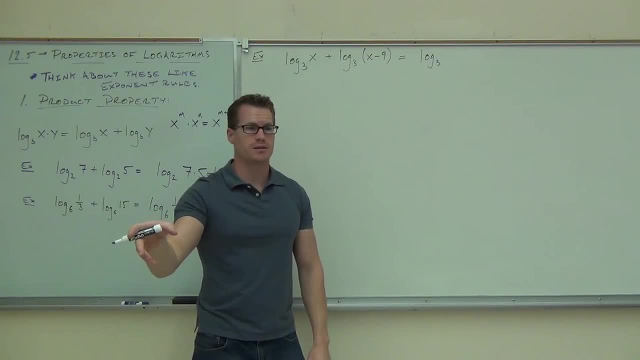 X squared minus three. Okay. how are you getting the X squared minus three? Three minus nine X, Three minus X, Okay. so I'd like you not to do that right away. Just make sure I'm seeing where this is coming from. 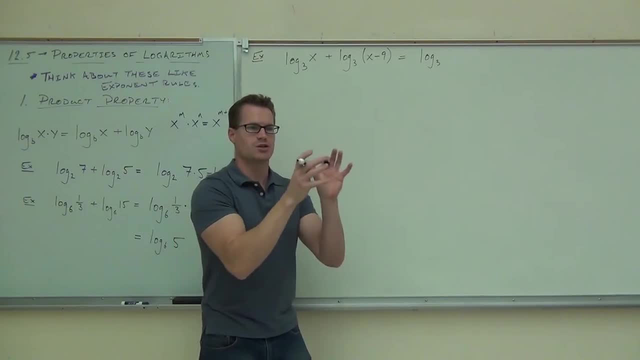 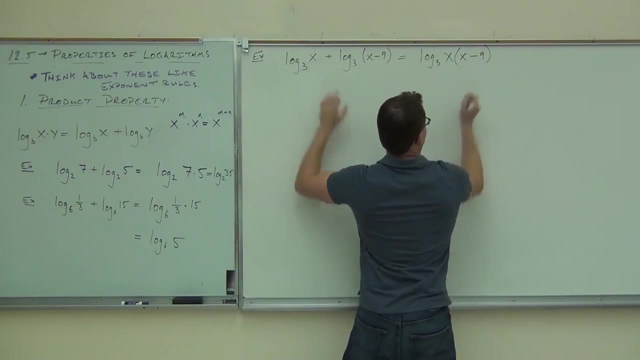 That way, in case you make a mistake on it, I'm like, ah, you don't know anything. I wanna make sure you at least get this step down. Okay, so show me this step real quick. Show me the X times X minus nine. 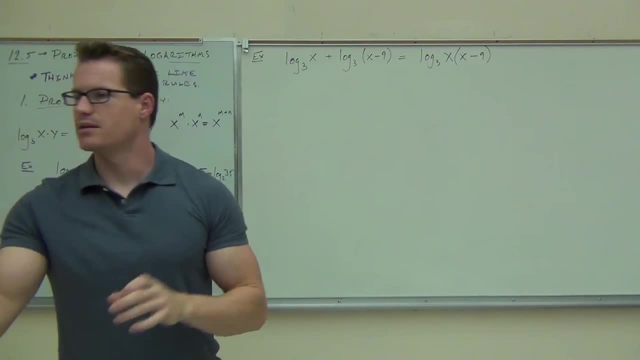 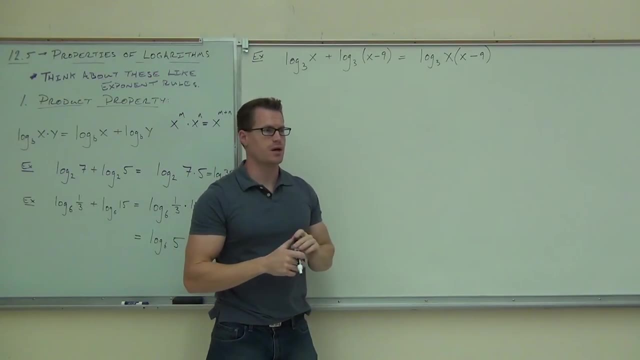 That says to me: hey, I know the product property. It says I know that I can take these two insides of my logarithms and multiply them together, since it had one log plus another log of the same base. Now you're gonna be all right with that. 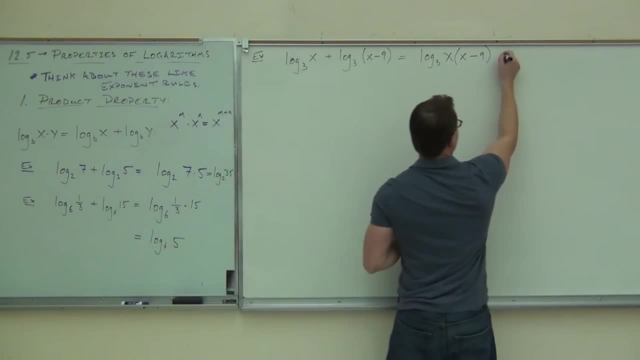 Can you distribute? Sure, of course you can, And then, of course, we'll get the X squared minus nine X. One thing I do need you to do, though: if you do distribute that, please put parentheses around this. Please put parentheses around that. 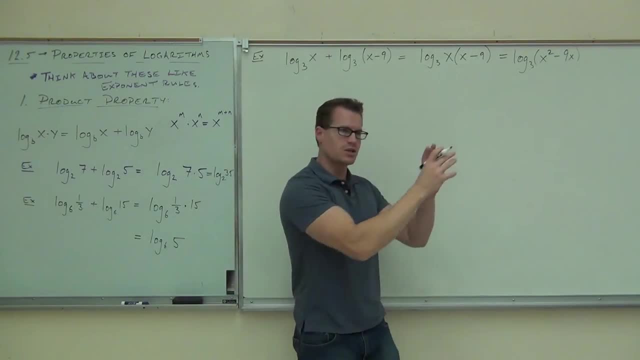 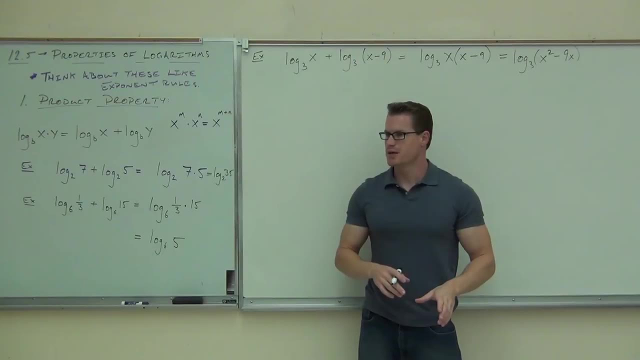 Otherwise, if you look at it, some people might think, if you write this just a little bit sloppy, that you're talking about log base three of X squared and then minus nine, X. Right, We wanna say log base three of that whole entire thing. 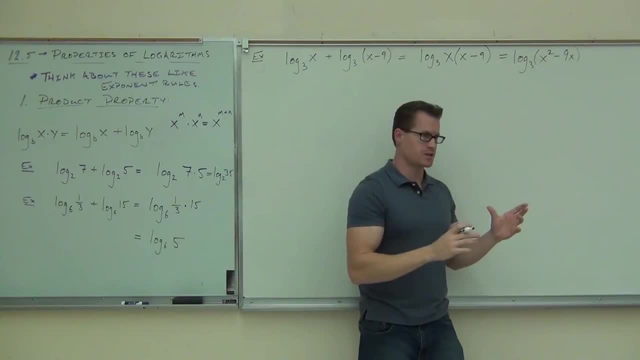 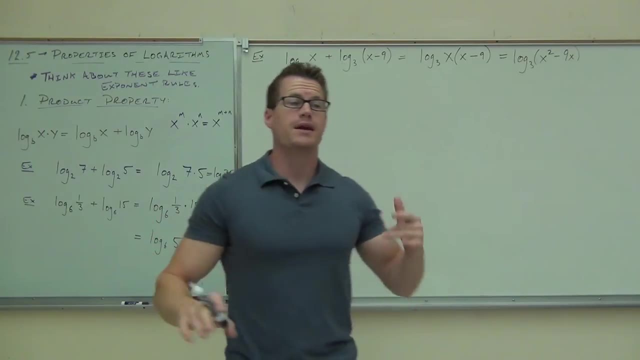 That's one expression for you. So if you do distribute it, put your parentheses there. You got it All right. Are there any questions? so far on what we're talking about? One thing I do wanna show you here real quick. Make a little note on this. 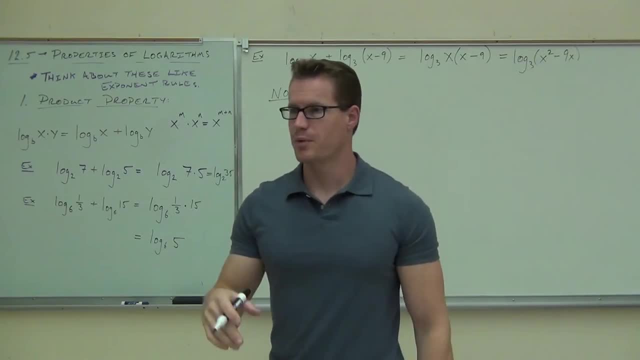 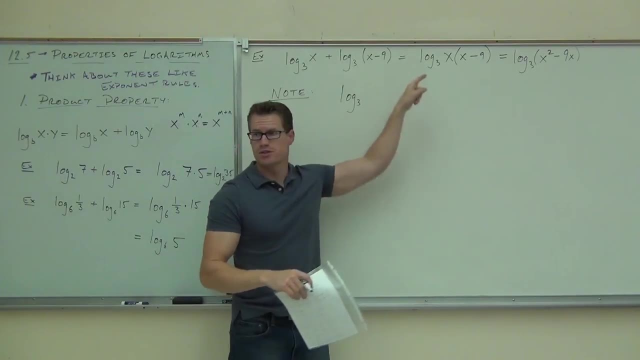 All the time this happens. This happens a lot. This happens with people that are just learning logarithms. They get this right. They know they can put things together by addition and you're not actually adding these two things right, You're multiplying those two things. 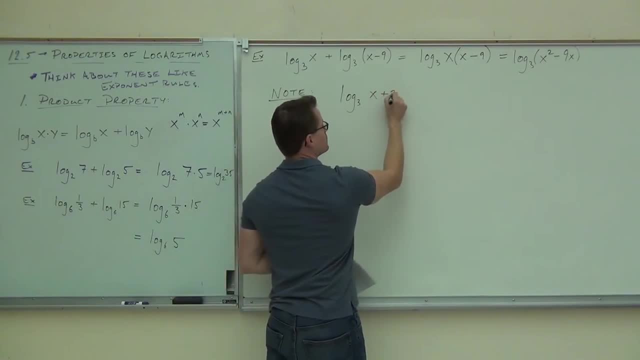 But then when they get to a problem like this, one like X plus two, log base three of X plus two, and I ask you to go the opposite way, I ask you to expand it. You know what a lot of people give me. 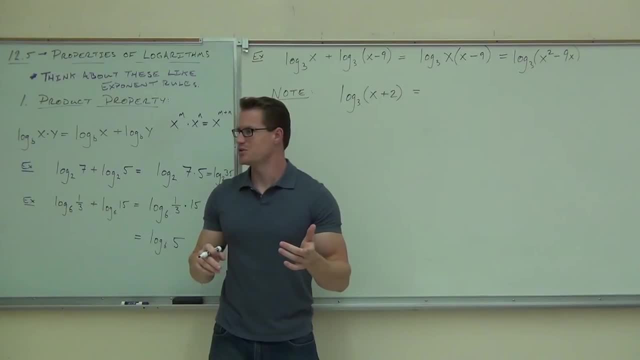 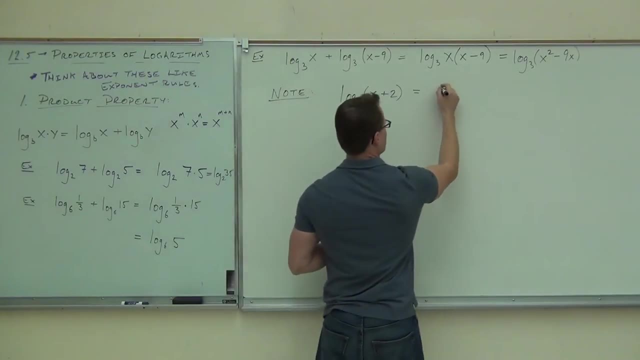 I'll bet you could tell me what they give me here. What would you think they would do there? Yeah, they give me this, They give me that. Now is it a true statement? What do you think? Does this follow the product property over here? 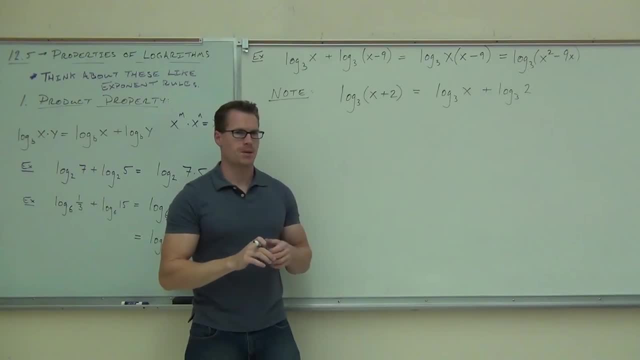 Are these two things multiplied together, Then you can't split that up. This is kinda unique, right? It's working a different way. You can't split up addition if it's within that logarithm. The only thing you can do is split a multiplication. 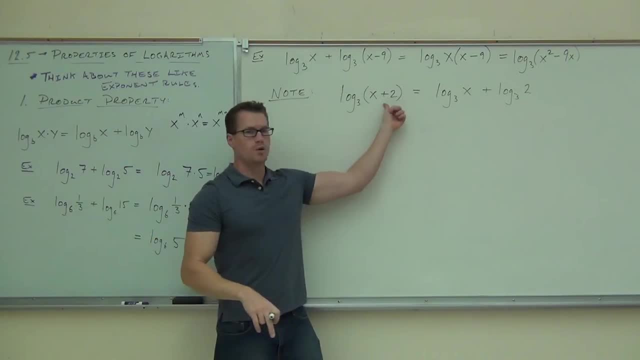 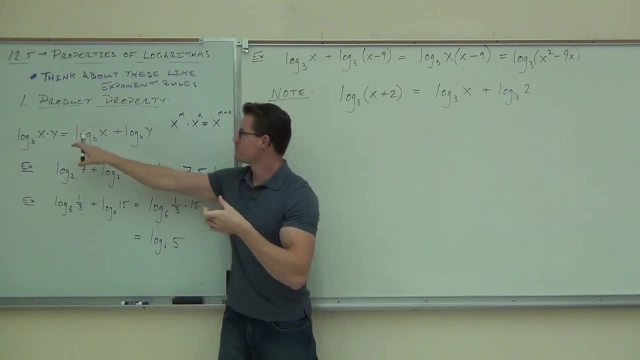 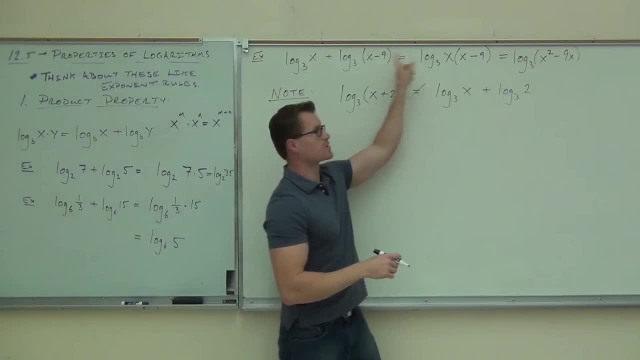 You cannot split up that addition. Can you split up multiplication, Absolutely. Can you split up multiplication this way? Sure, No problem. Can you put together addition? Yes, You can't split up addition, not if it's within the logarithm. 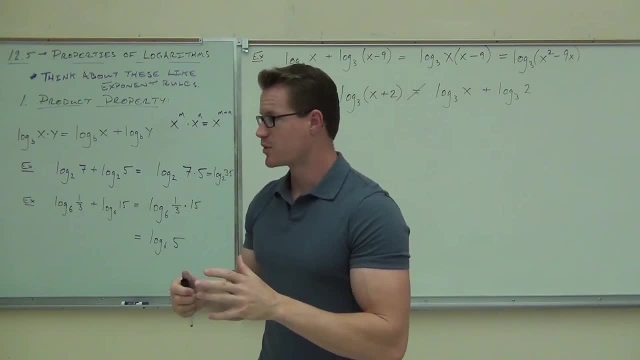 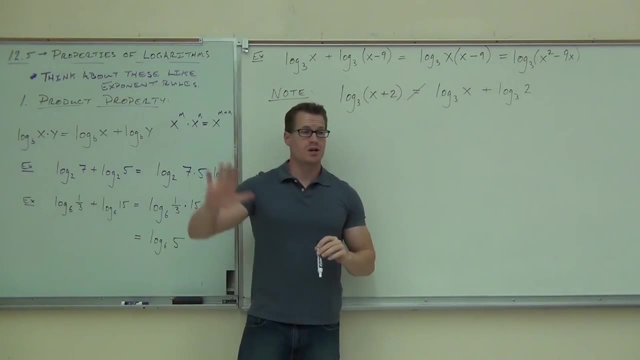 These rules- I mean, they're not too tough rules. They work very similar to exponent rules, but you really do have to memorize them, Otherwise you're gonna get down here and think that's possible. We can't do that. Would you be okay with this so far? 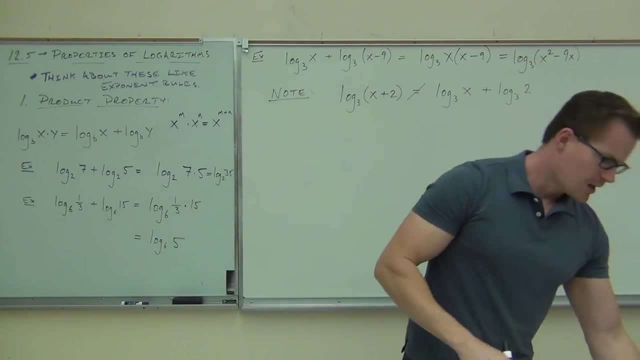 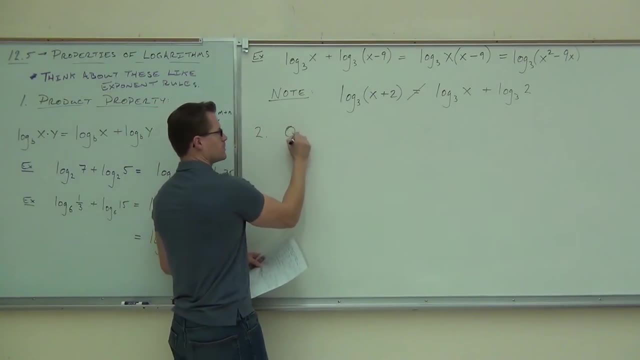 No Good, All right, Now there's two more properties we're going to talk about. The first one's called I'm sorry, the second one. the first one's this one. The second one's called the quotient rule. 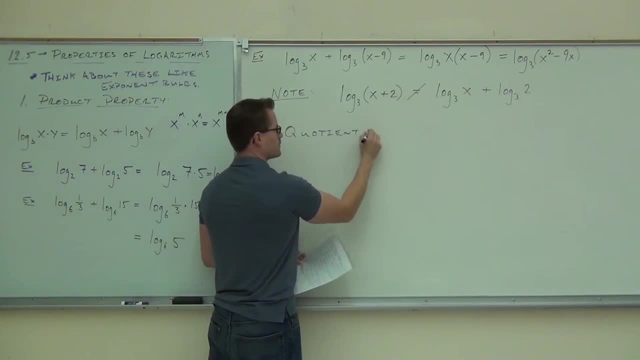 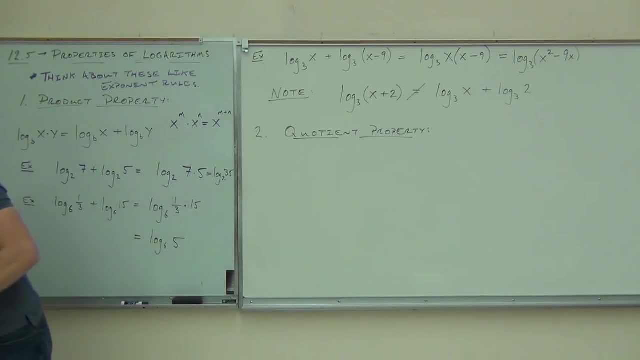 or quotient property. What's quotient mean? Division, Yeah, So instead of a product and our multiplication over, here we're going to be dealing with a quotient and some division. Hey, let me ask you a question: If we split up multiplication by addition, 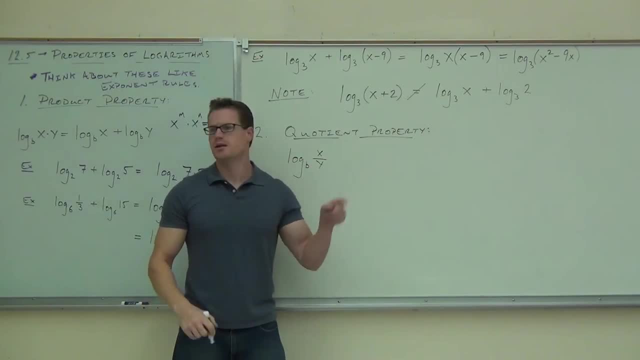 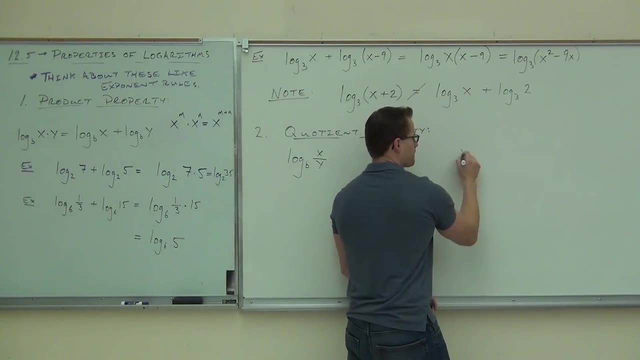 what do you suppose we're going to split up division by Subtraction? It's going to be exactly the same as your excellent rules. Remember, with your excellent rules over here, when you had something like x to the m over x to the n, what did you do with those exponents? 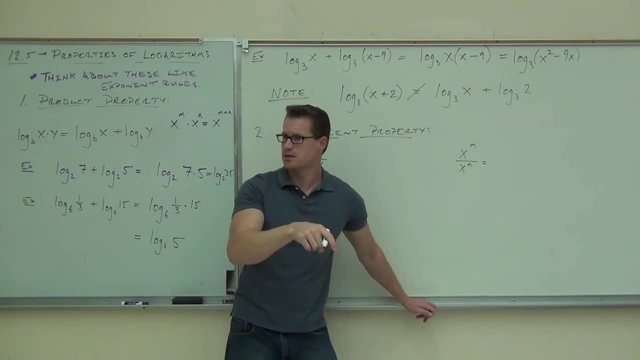 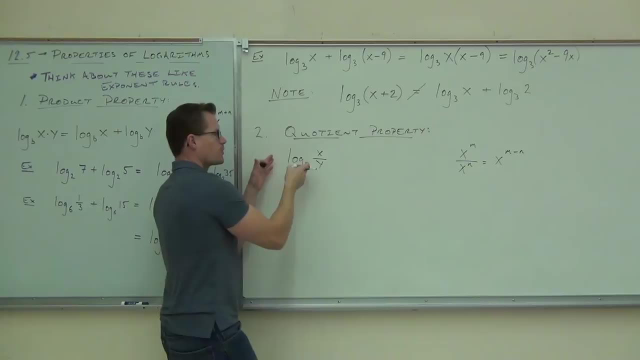 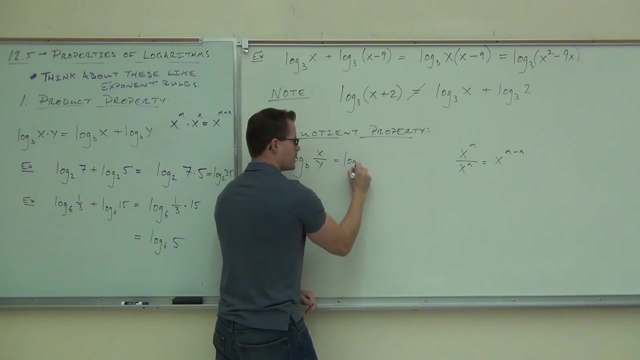 Subtraction. Sure, you subtracted x to the m minus n, didn't you? Same exact idea over here. If we have log base b of x over y. so remember this is inside of our logarithm. here we can split that up. log base b of x: That one has to come. 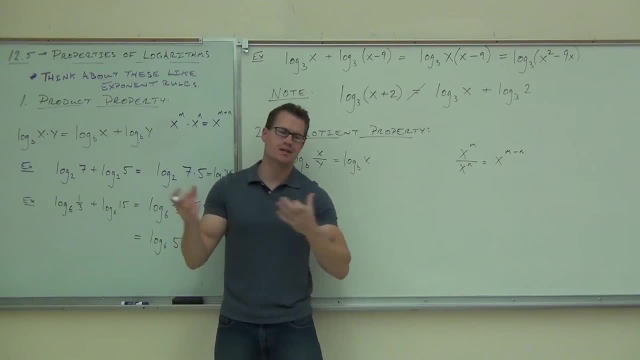 first, though The top of your fraction must come first, because, well, it's not commutative: Log of x minus log of y is different than log of y minus log of x. So, notice, we can split up one logarithm into two logarithms. 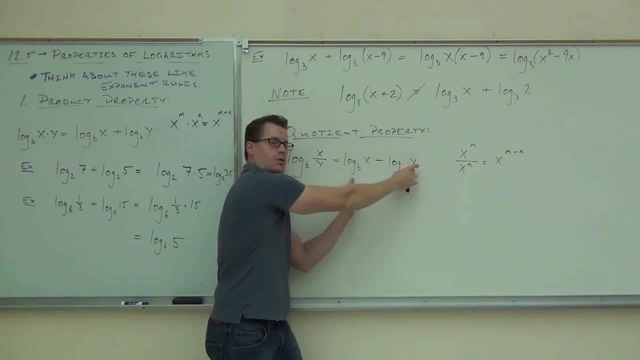 by our quotient rule or we can put this together. We can put together two logarithms into one logarithm using our quotient rule in the opposite direction. You guys all right with this one? Mm-hmm, Remember, think about my exponent rule. 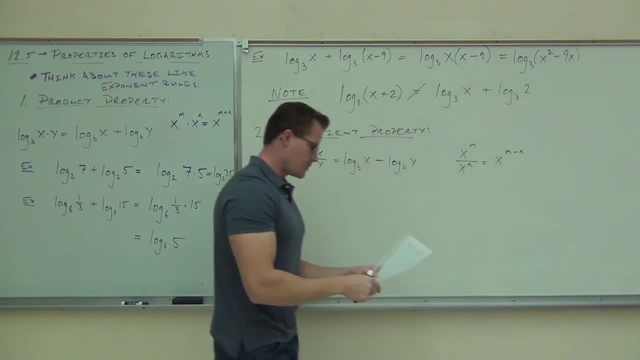 is that it really gives you a handle on what's going on here. Now let's try a couple of examples. A lot of you do some on your own and we'll move on. OK, log base 7 of 40 minus log base 7 of 8.. 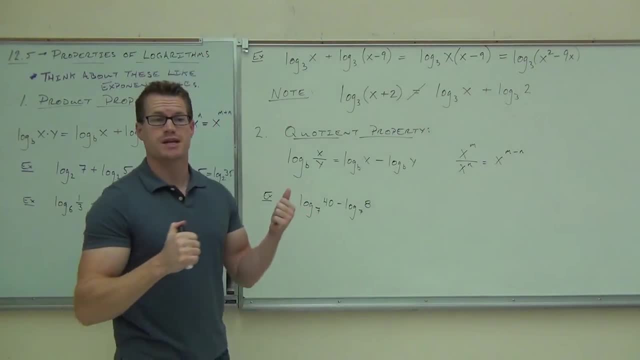 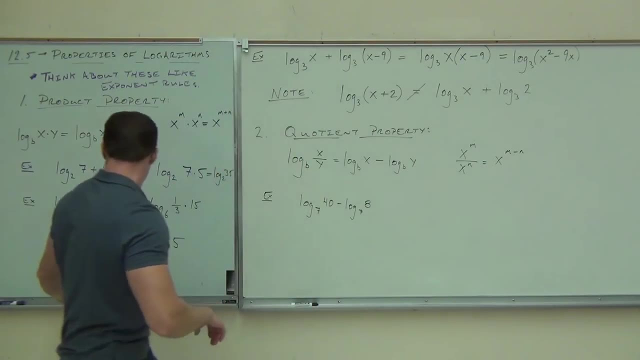 First thing, can I put those two logarithms together? Is that possible in this case? Yes, Yeah. what tells you that? again The same basis. So you've got to have those same bases. That's something to look for every single time. 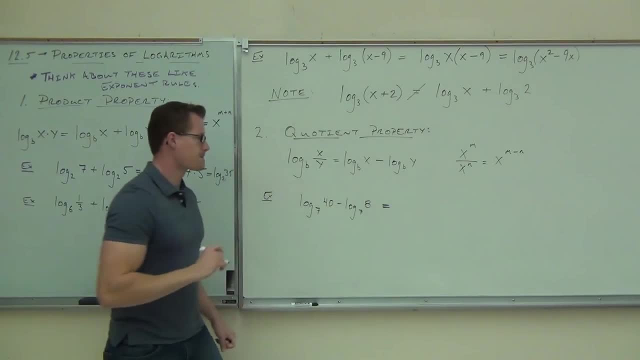 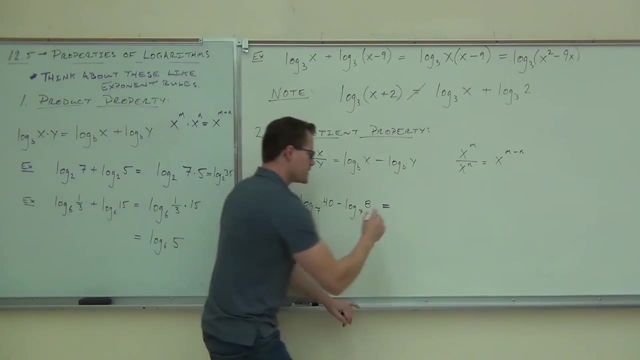 Now, when I write this out, what am I going to get? Log base 7 of 40, minus log base 7.. Log base 7 for sure. Now here's the question I need you to look up here, because this is another mistake. 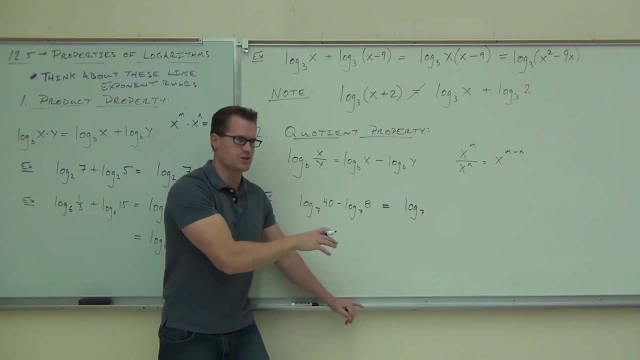 that people often give me. I'm going to show these mistakes to you, That way you don't make them. A lot of times people confuse this And they say, oh well, log base 7 of 40 minus log base 7 of 8.. 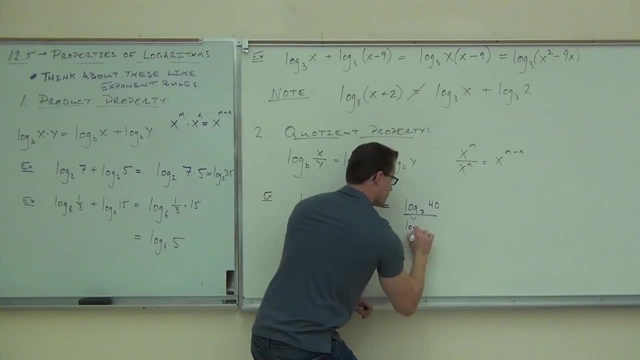 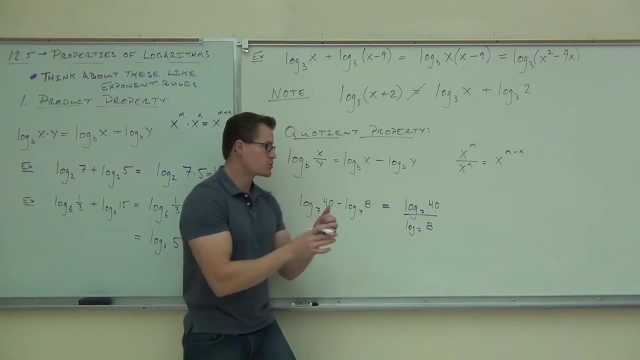 Well, that should be log base 7 of 40 over log base 7 of 8.. Do you see how they could make that mistake? When you're combining logarithms, you're changing two logarithms into one logarithm, not one logarithm. 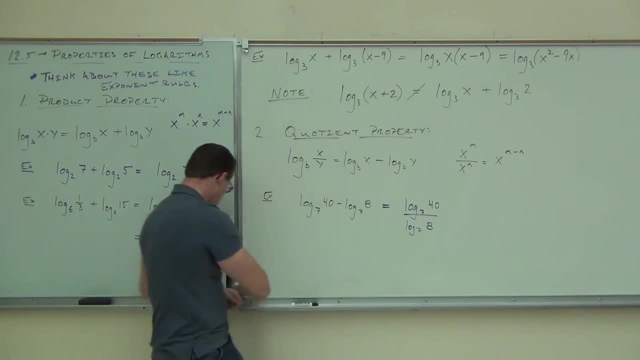 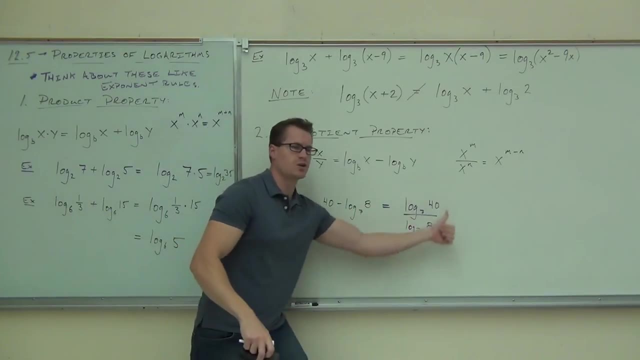 over another logarithm. You see there's not another logarithm over there. It's really combining your logarithms. It's changing two of them into one of them using that property. That's kind of nice. This is worse. You don't want to have that. 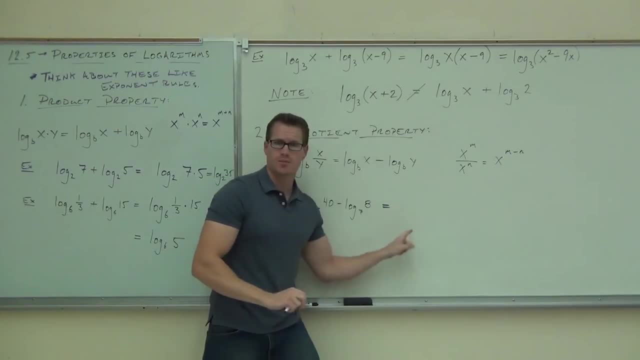 It's not simplifiable. You couldn't do anything with it. Are we going to see this in some places? Yeah, Yeah, we are, But you can't combine that at all. There's no way to put that together. Instead, we have log base 7, just one log. 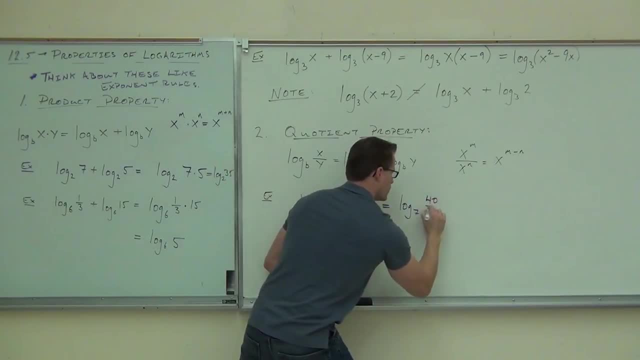 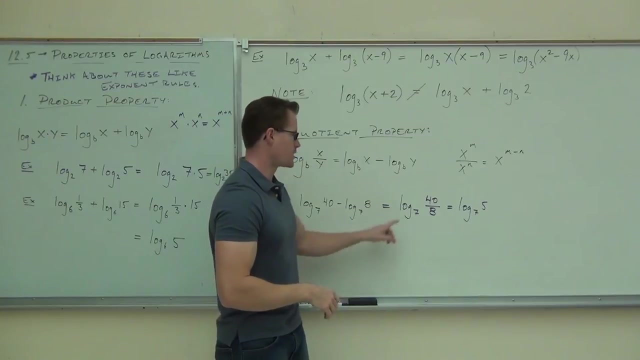 What number is going to go on the top 40. Sure, And can you simplify it? Yeah, we can Question. Order matters, right, Order definitely matters. Order definitely matters. The top number, our numerator, is our first logarithm. 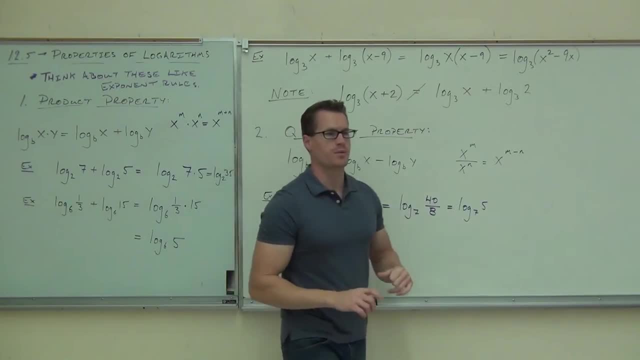 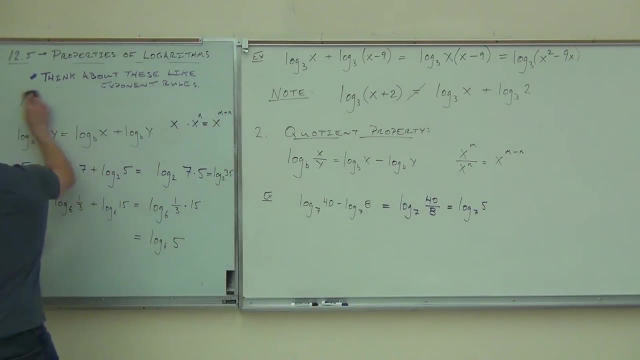 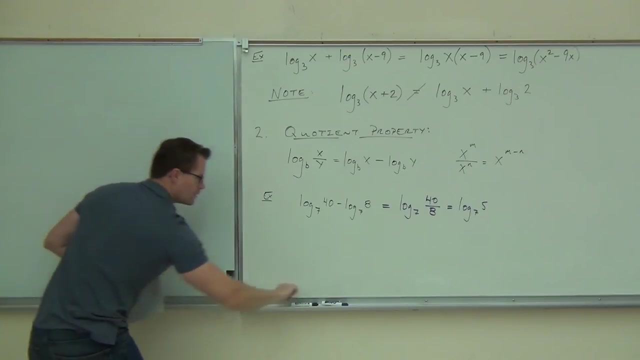 The second number, our second logarithm, is our bottom number, that denominator. Yeah, order definitely matters. Good question, Let's do a couple more here. Let's do log base 9.. Log base 9 of x minus log base 9 of 5.. 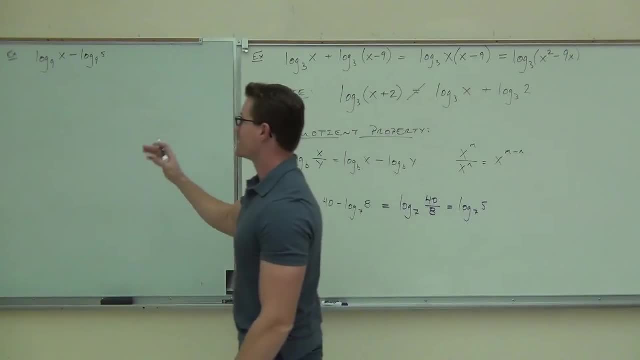 Now, clearly, we've got a couple of logarithms that have the same base. We have 9 and 9.. That's great. We're going to go ahead and we're going to combine these. Are we going to be multiplying, subtracting, dividing? 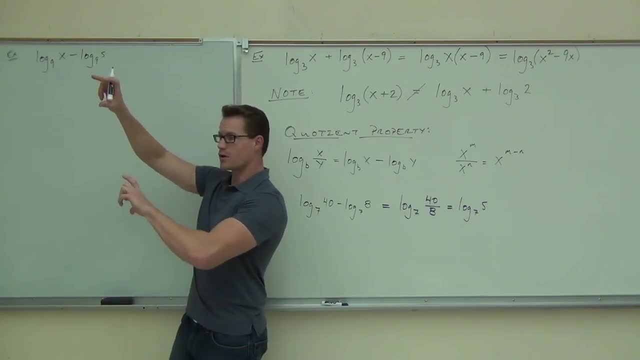 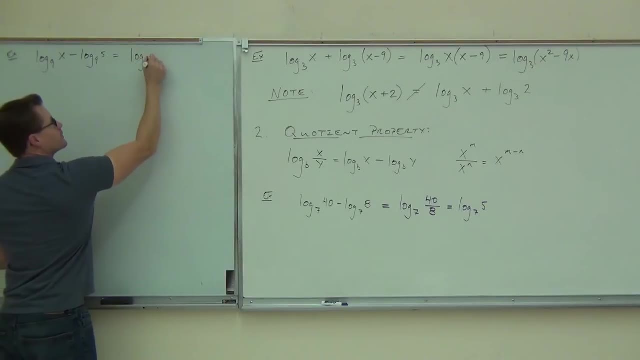 or adding Which one, Dividing, Dividing. Now, is it going to be a log over a log or one log? What do you think? One log, Sure, So we're going to have one log, base 9.. And then we'll have a fraction. 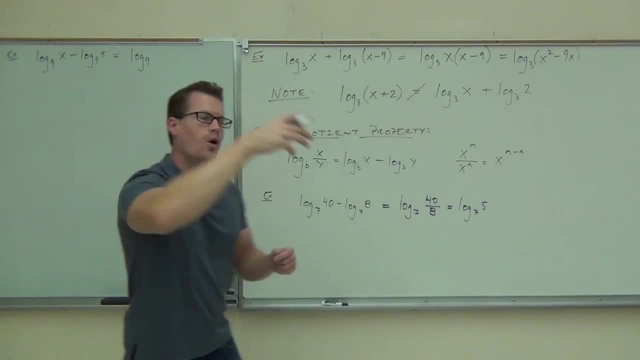 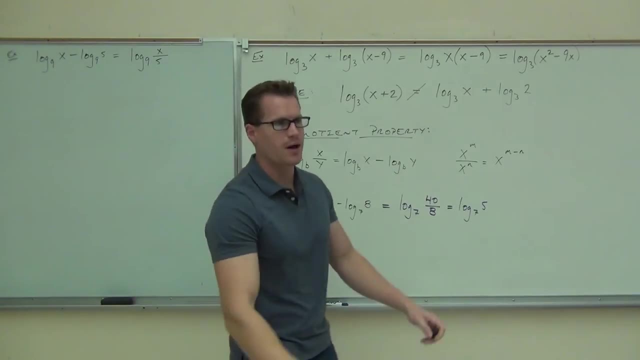 We have our first logarithm on the numerator. whatever the inside of that logarithm is over the second logarithm, which is 5, in this case x over 5.. Now, there's nothing we can do with x over 5.. 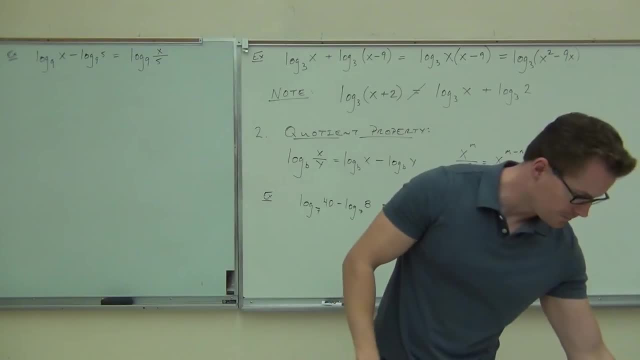 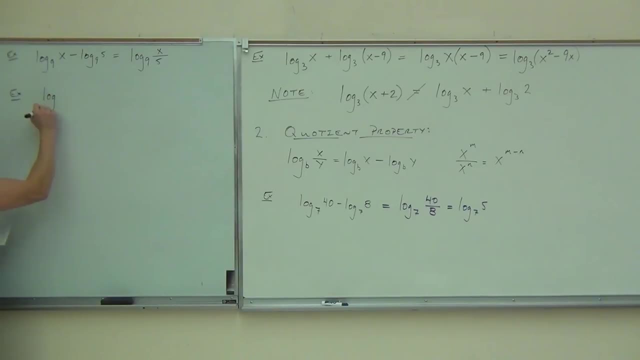 We just leave it. It's one way that we can put logarithms together. OK, Log base 3 of x cubed plus 4.. Notice how I'm putting the x cubed plus 4 in parentheses. that's saying log of that entire thing. 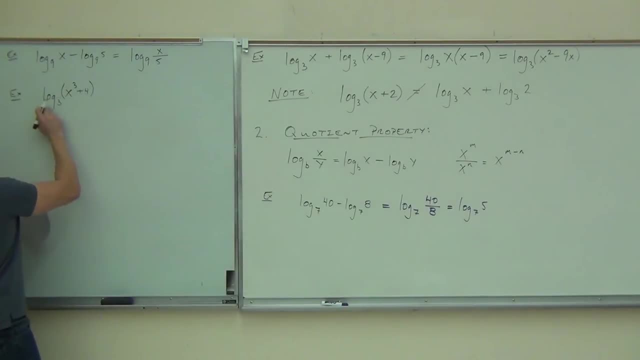 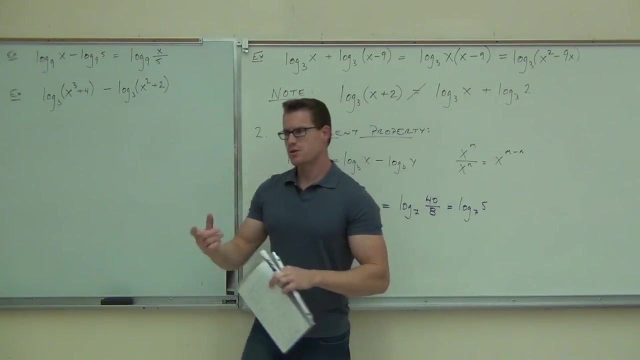 If I didn't do that, it could be misconstrued, just for people to think this and then plus 4 at the end. So we really do need to show those parentheses. Can you put these ones together? Let's go ahead and try that. 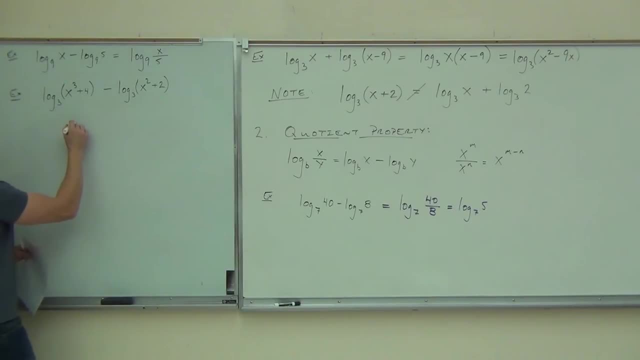 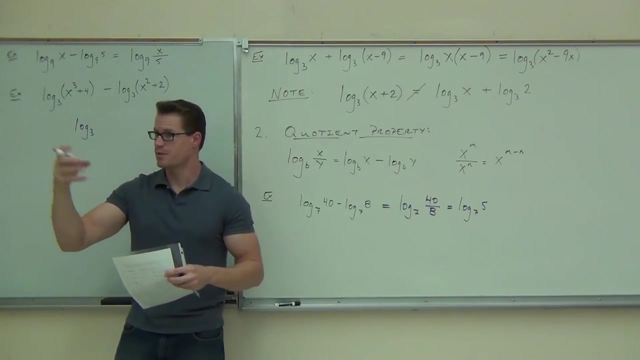 We'll get. what exactly are we going to get? Why don't you tell me Log 3. Log 3,? OK, great, That's the only log I should write right, Because I have those two logarithms. I've combined them to one. 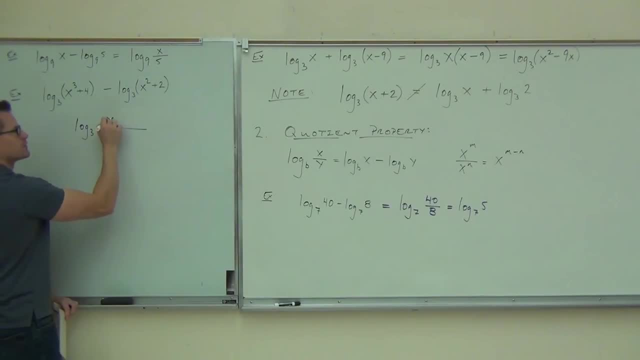 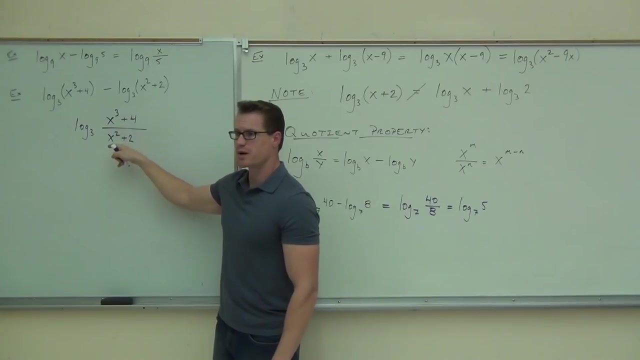 What's going to go on? the numerator of my fraction, x squared- Perfect, And denominator x squared. That's it. You try to simplify it. You can't factor any of this stuff. Can you cross out the x cubed and x squared? 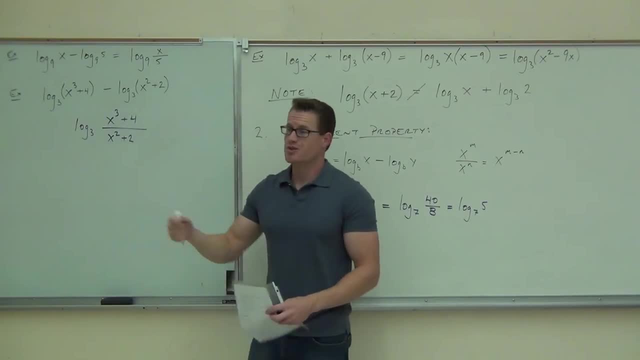 No, No, no, don't do that. No, you can't do that. It's connected by addition, So you're done. That's as far as you can go on that example. Are you guys ready to try some on your own? 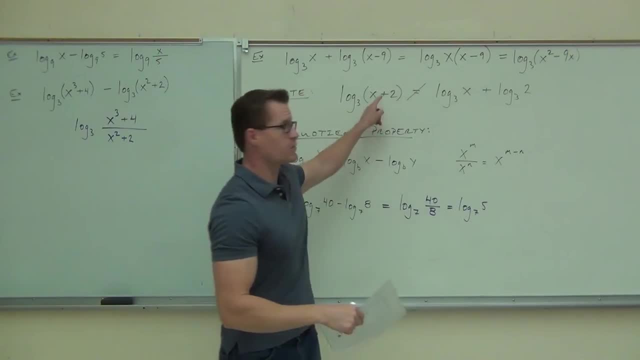 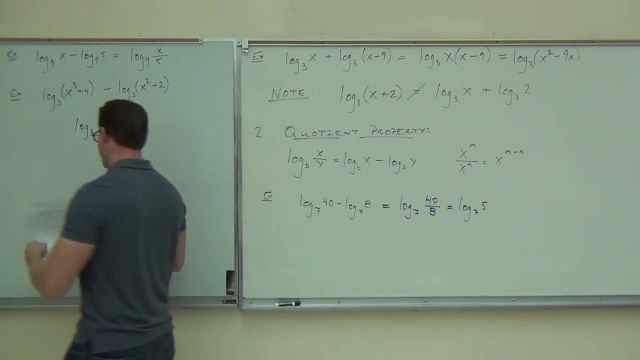 Yeah, Good, all right. Before we do, I want you to write some notes, just like this one. that wasn't true. Write these things out. That way you see some common mistakes that we have on your paper. Look them over. Make sure you're not making these mistakes, all right. 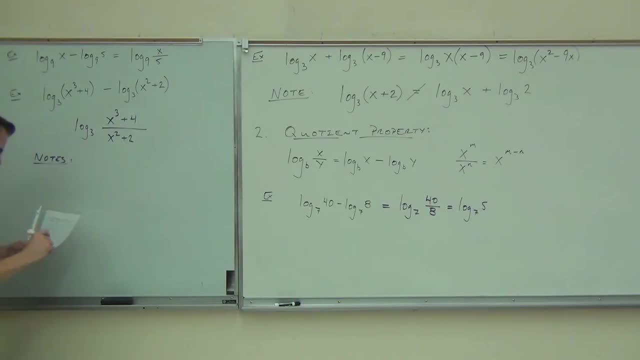 So a couple notes here. First thing: Look back at your product property. Can you combine those? Look back at your product and look very carefully at your product property. Can you combine those? Do they fit? If it doesn't, look, now listen. 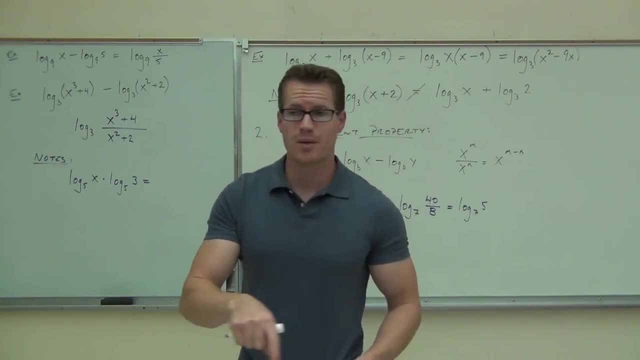 These properties are something where, if it doesn't look exactly like it does on the paper- exactly like the property- you can't do anything with it. If it doesn't look exactly like it does on the paper, you can't do anything with it. 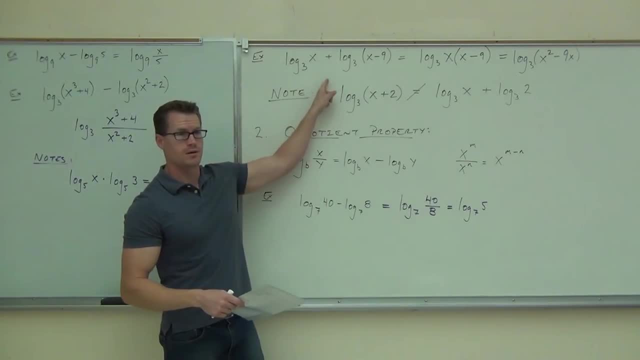 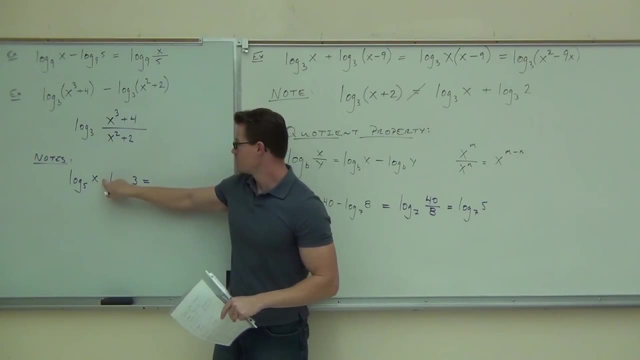 Does this look exactly like this one? No, No, this has two logarithms that are being multiplied together. Multiplied, not added. Could you combine this Absolutely? Can you combine? oh, that messed up. Can you combine that? 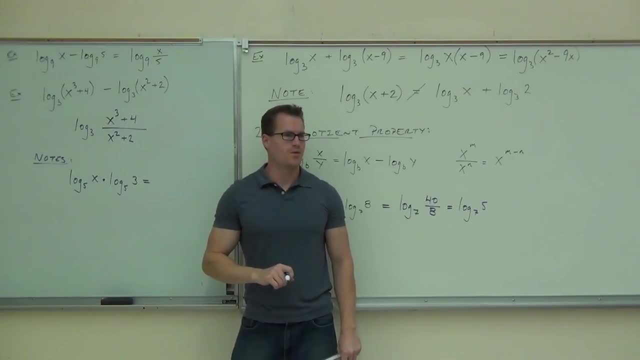 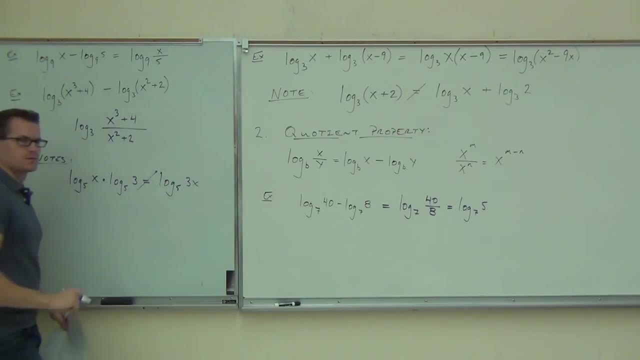 That's hard to do. Can you combine that? No, No, you can't. This in no way equals, this Does not. even If that was a plus, yeah, that would equal, That'd be great. But you cannot combine multiplication, two logarithms. 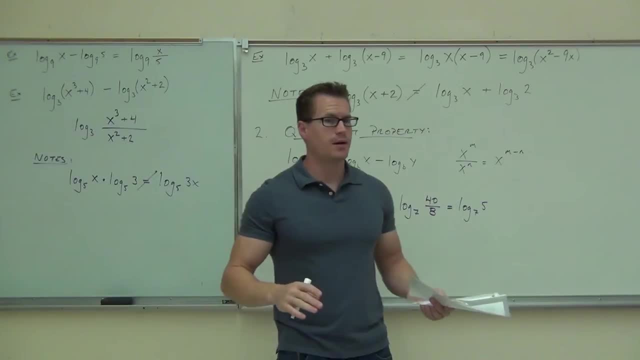 There's nothing you can do with it, You just leave it. You can't do that. Not sure if you're OK with that. So are the rules hard? No, but they're very specific rules and you have to have them exactly down. 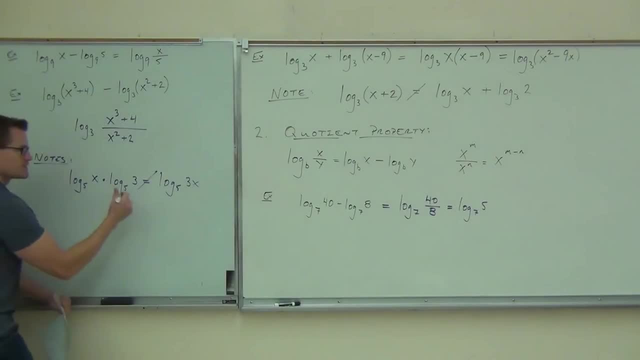 Right, Exactly the way they are. Also, this doesn't equal log base 5 of x plus log base 5 of 3.. That might seem silly to you. Of course. product doesn't just directly equal plus, right? You can't do that either. 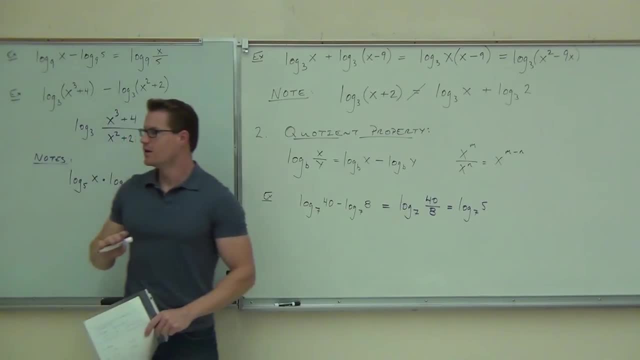 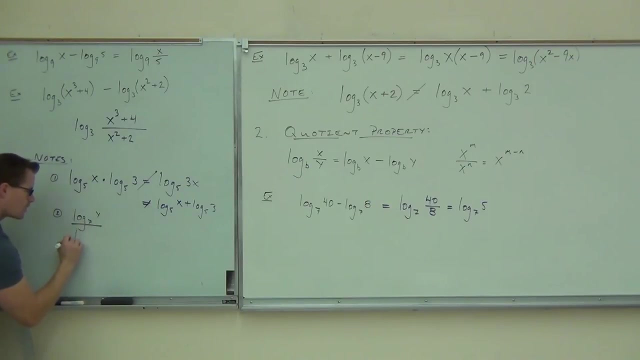 So this is just the way it is. You can't do anything with that Couple other ones. I showed this to you over here, but I want to make sure you really see it. If you ever have a logarithm over a logarithm like that, can you combine those two logarithms? 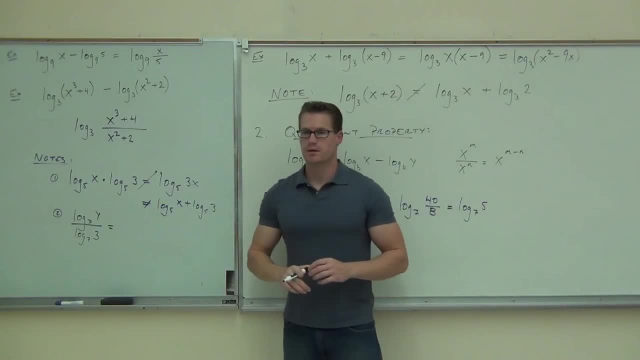 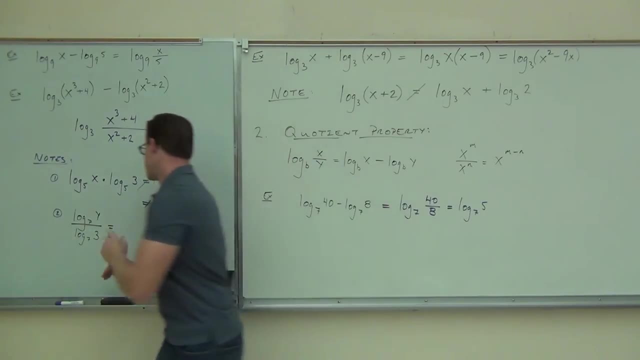 What do you think? Does it look exactly like the property that's on the paper? Does it look exactly like this? No, You can't combine them. This in no way equals this. That does not equal. You can't do that. 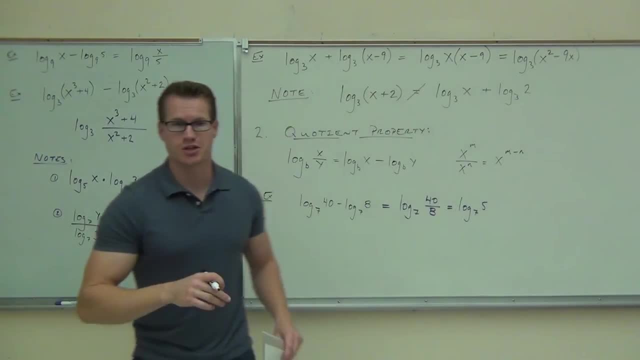 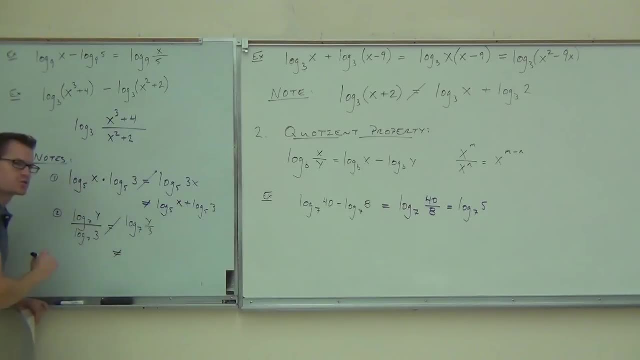 You can't put them together. They literally have to look identical to the properties I just gave you, Otherwise you can't work with them. Also, this doesn't equal subtraction. You can't split this up by subtraction either. You can't do log 7 y minus log 7, 3.. 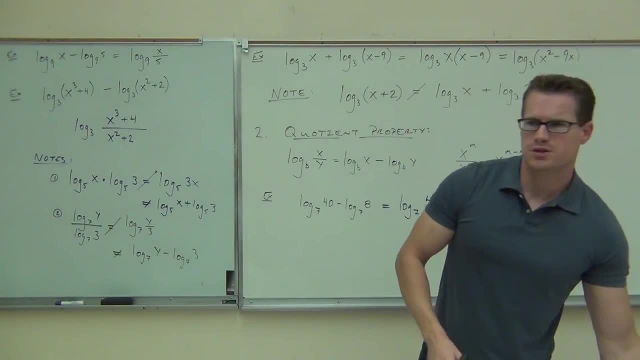 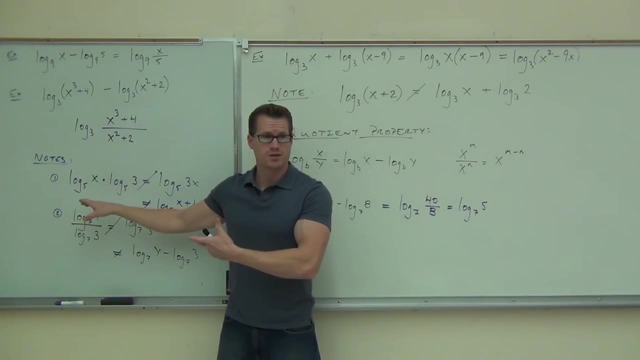 Neither of those things are equal. Those are pretty much the four most common mistakes that I see. I see a lot of this. This one looks like it should be possible, right, Because you think multiplication, multiplication. But here's what that comes down to. 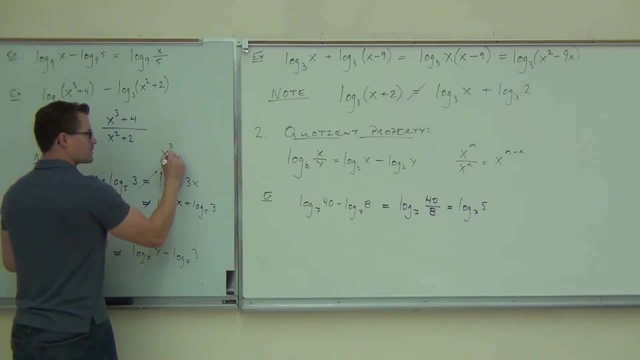 That would be like saying this: X to the third times x to the fourth equals x to the twelfth. Is that a true statement? No, That's x to the seventh, isn't it? It's not the same. It's not the same. 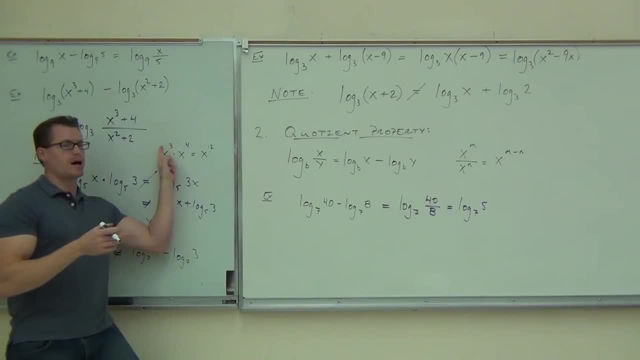 They work like exponent rules, So you can't just multiply your exponents together. That's what this would be doing. That's an exponent, That's an exponent. You don't multiply those things together. It doesn't work, It doesn't compute. 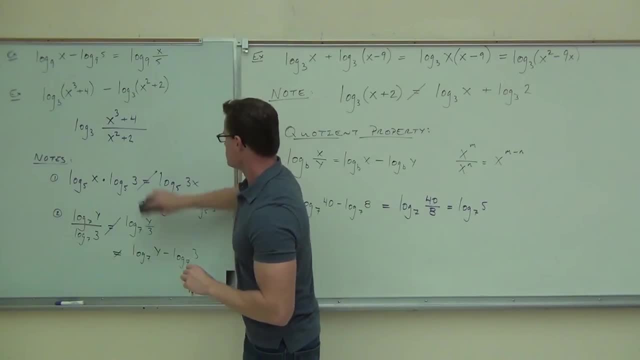 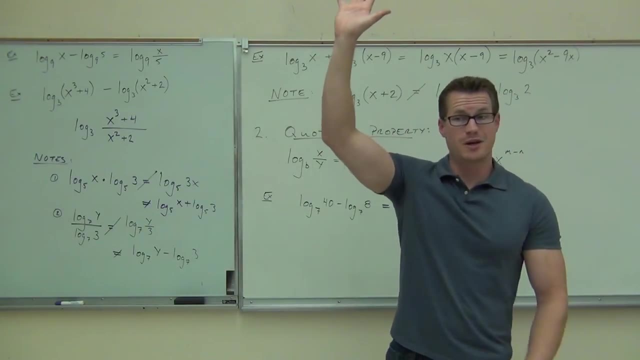 It's similar to that. It's not exactly the same, of course, but it's very similar to that idea. Would you raise your hand if you feel okay with this so far, especially these non-rules that we have over here, the ones that you can't do? 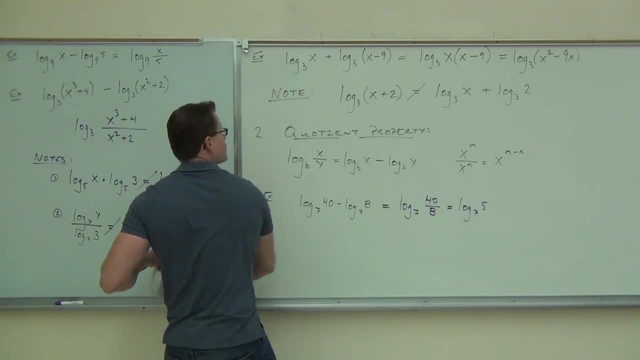 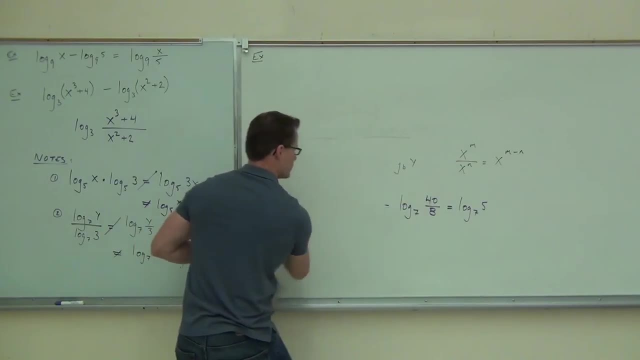 All right, With that in mind, go ahead and give these examples a try. All right, We're going to do this one over here And then we'll move on. Let's do that one. So right now we're just combining. 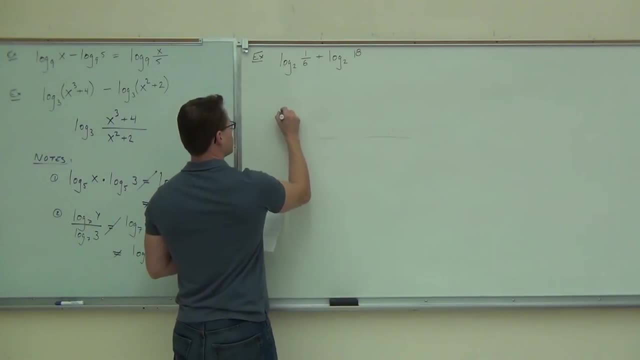 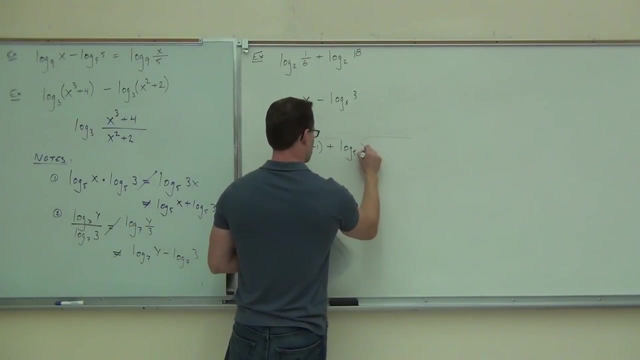 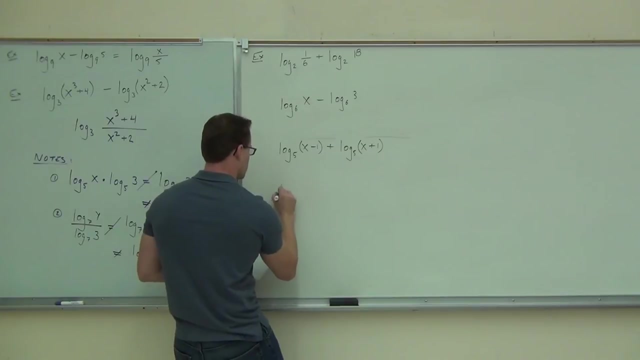 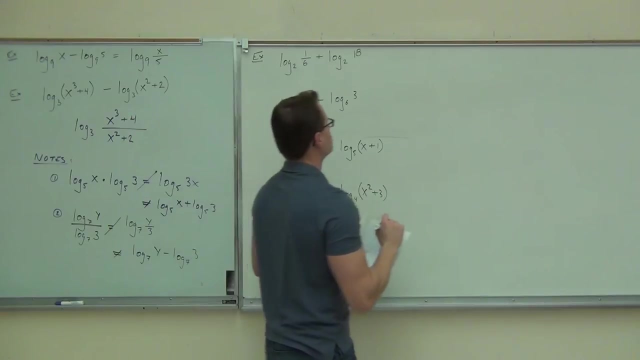 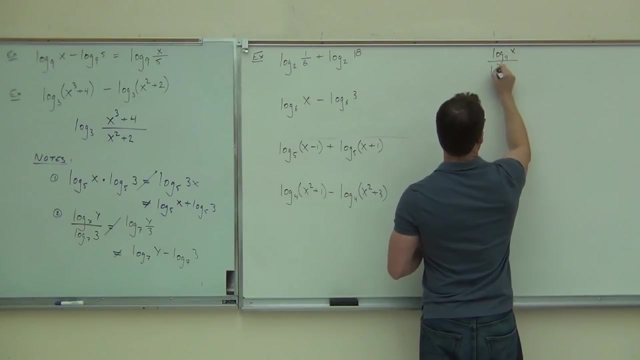 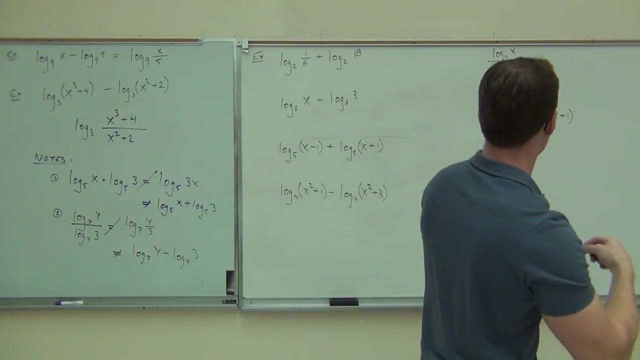 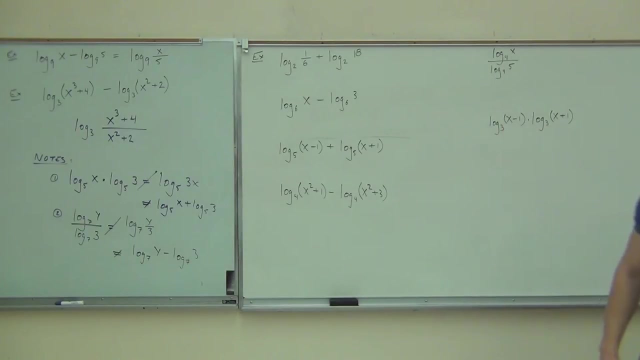 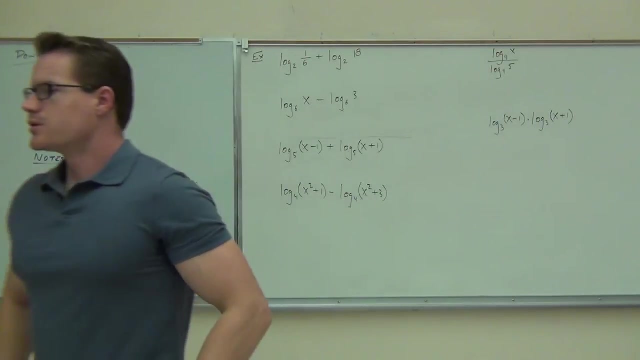 I'll show you expansion in a little while And then we'll move on. Thank you, Thank you. Okay, go ahead and work on those. Remember, we're trying to combine in every case, Thank you, Thank you. So these properties say: if we have two logarithms being added together, 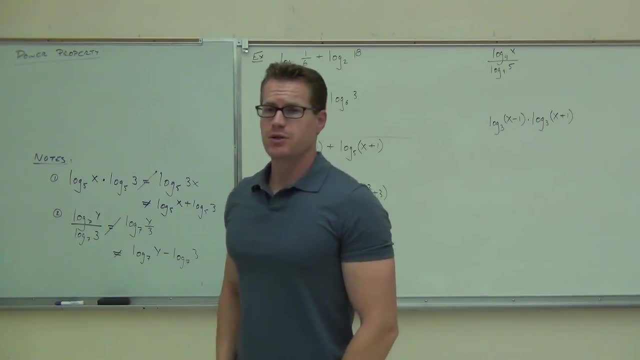 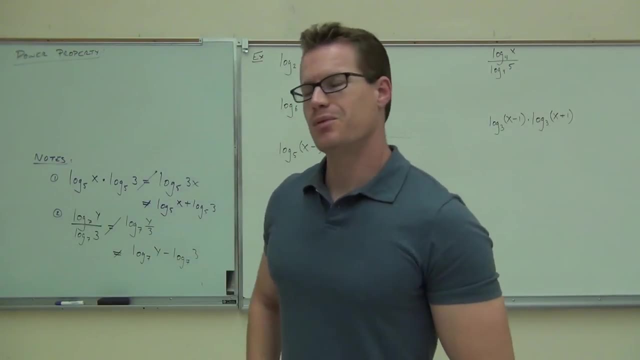 it's a product property, We can combine that by a product. If we have two logarithms being subtracted, that's a quotient property. We combine those with a quotient. If it's not exactly like those things, we can't do anything. 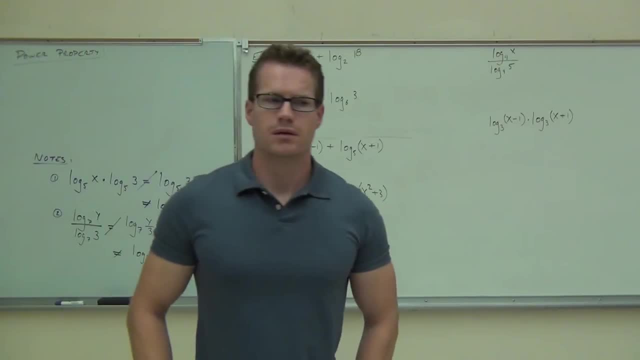 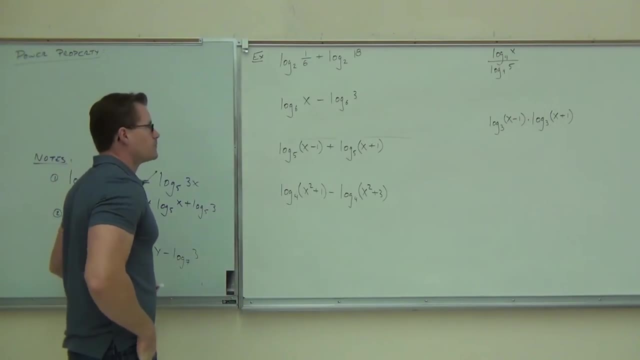 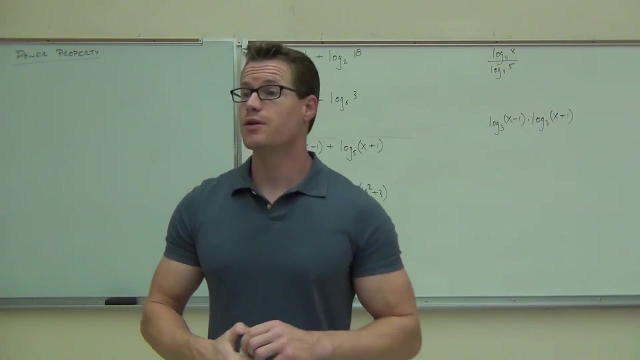 We can't do anything with it. Looks like we're about done up here. Take a couple more seconds, see if you can wrap it up. Okay, let's look at the first one. Is that combinable? Can we do something with that? 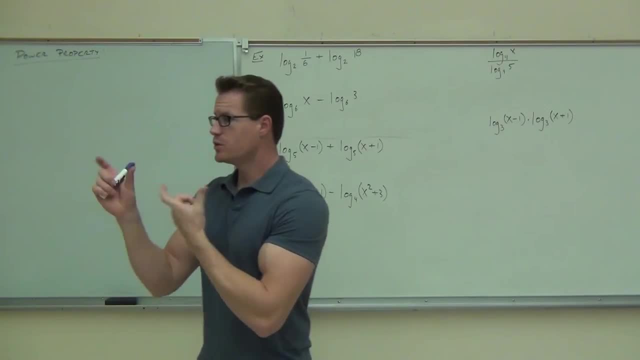 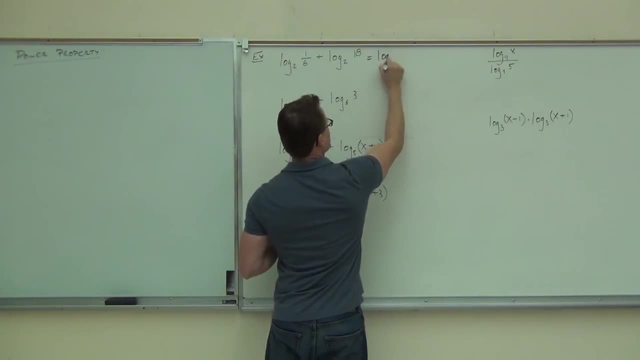 We're going to get one logarithm out of it. It'll have the same base And we're going to what's going to be on the inside: One, sixth, one, sixteenth, Sure, Not plus, Not plus. We can't combine logarithms with a plus. 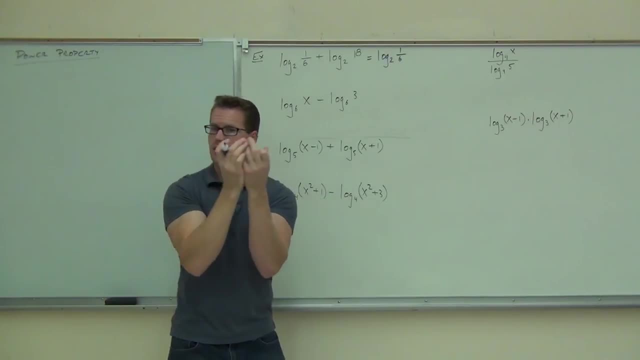 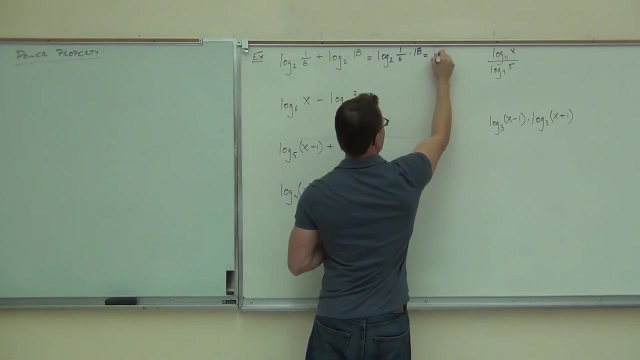 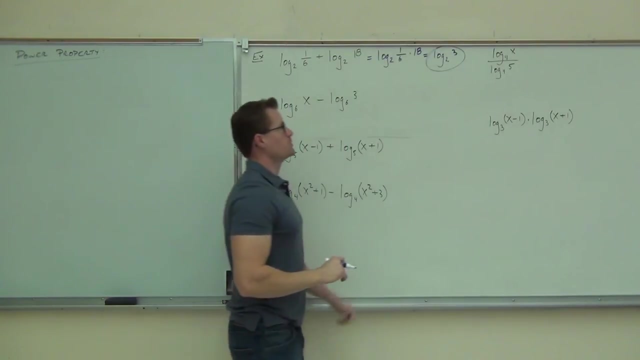 We say if we have two logarithms being added, that's the same thing as a product of the inside of those logarithms. Yeah, That means we'll get log base 2 of 3 is how that's set, Log base 2 of 3.. 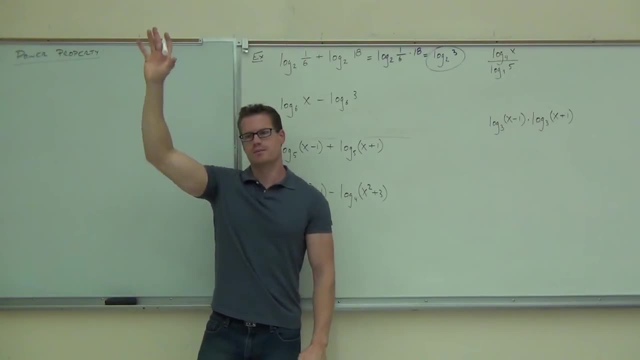 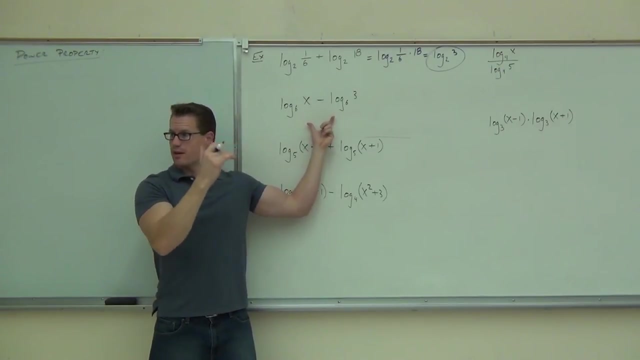 Raise your hand if you've got log base 2 of 3.. That's good, That's great. That's great. Okay, next one. Can you combine these two? Yeah, It's got subtraction in there, right? That's good. 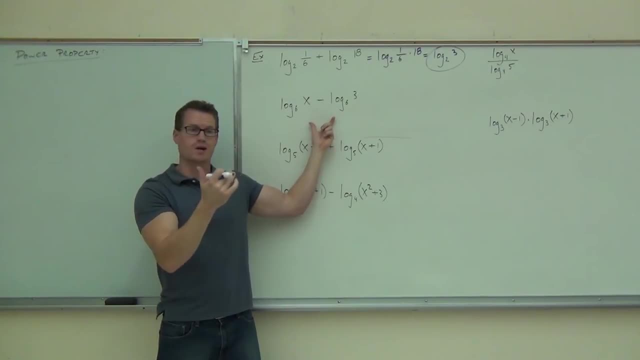 That's part of our quotient property. We've got common bases. That's great. That means we can actually put these things together. So, on the right-hand side, how exactly would you write that Log base? what? first of all, Log base 6.. 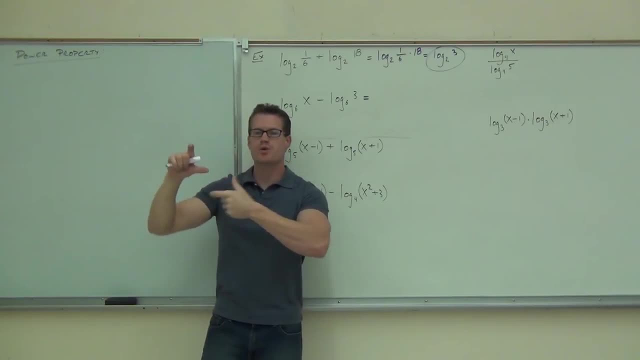 Are you going to have one log base 6 or two log base 6s? Remember, you're combining things. You're trying to change two logarithms into one logarithm. You don't want two anymore, You're trying to make it one. 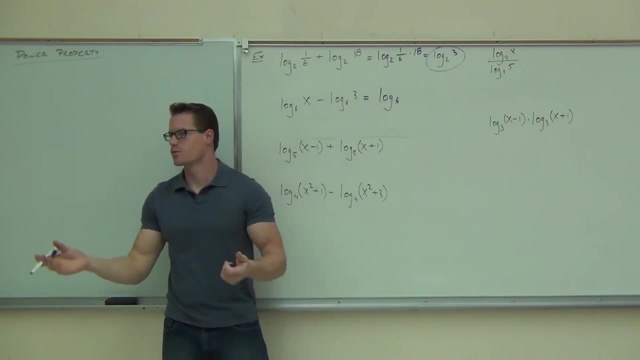 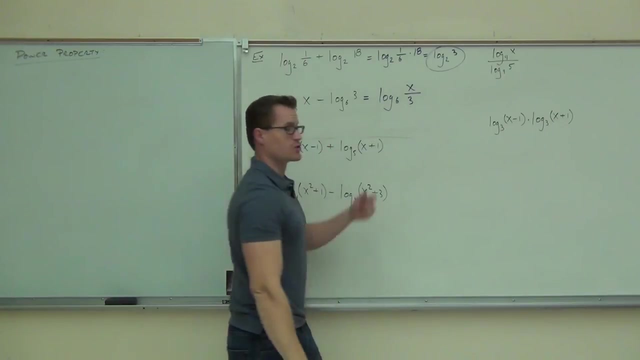 Okay, great. Now what? X over 3.. Good, X over 3.. Because you say: we take the first logarithm, that becomes the numerator of some fraction, and the second logarithm becomes the denominator of that fraction. There's nothing to do with that. 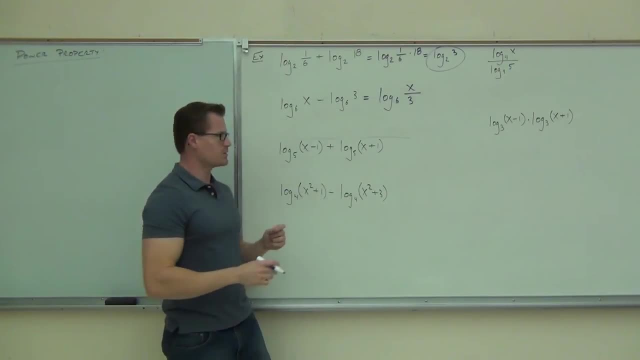 We're done. in that case, Did you make it that far? All right, Good, All right. Next up, how about this one? Can you combine these two? Sure, Yeah, It's plus same bases. That means we're going to have a single log base, 5.. 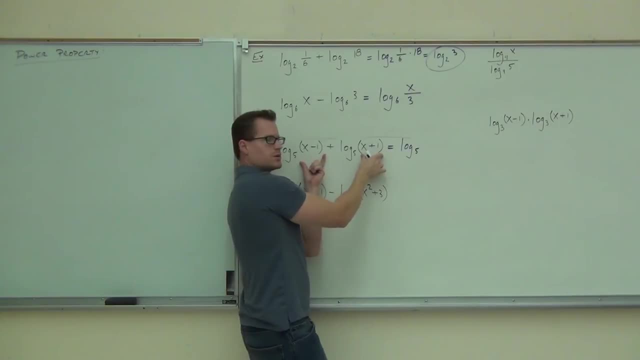 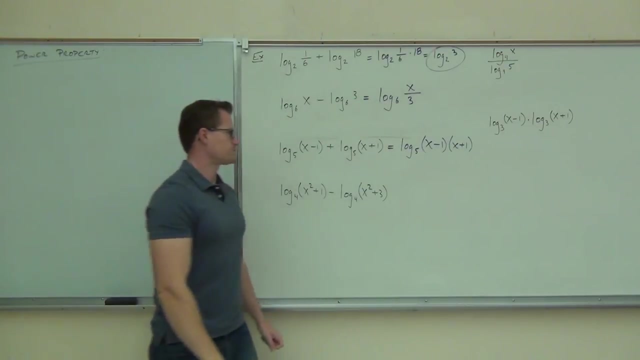 Are we going to add those or multiply those? So you should have X minus 1, X plus 1.. Yes, All right. Could you distribute that? Yeah, Yeah, if you wanted to, You get X squared minus 1.. 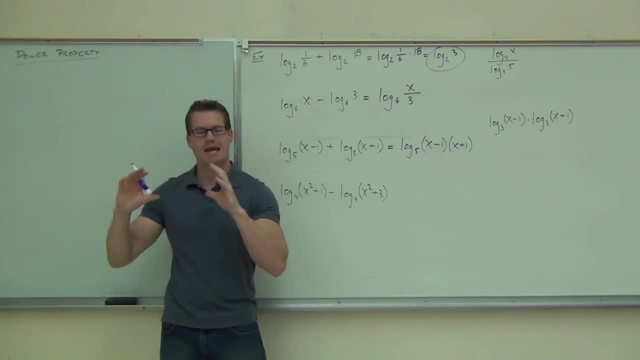 If you distribute, you get X squared minus 1.. Just make sure you have parentheses around it. You can't leave it without parentheses. So if you did this, if you did that, make sure that you go back and you put some parentheses. 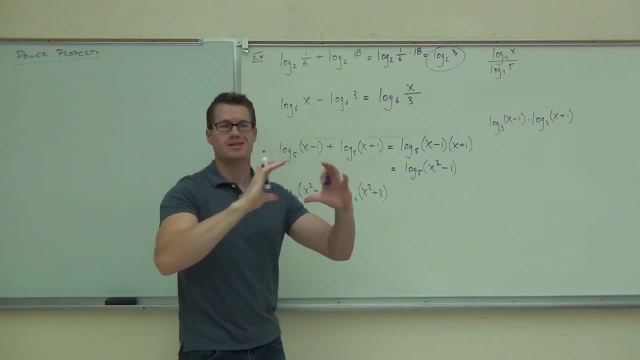 You have to show that it's a logarithm, the same logarithm, the entire thing. It's got to go with it. Okay, next up, can you put these ones together? Yep, Sure, we've got a subtraction, That's great. 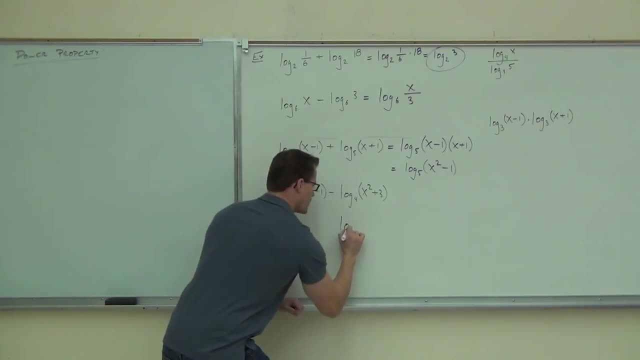 We know that's part of our quotient property. We have the same base. This would be log base 4, a single logarithm, not two logarithms. single logarithm of a fraction, because we know that the subtraction makes a fraction out of it. 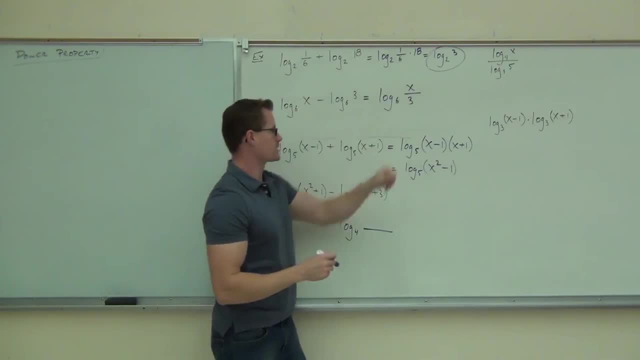 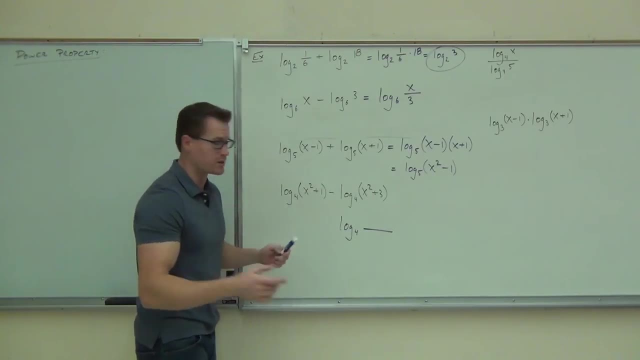 The way I always remember is: the P's go together plus product and the straight lines go together minus quotient. That's how I do it. It flows for me. If that works for you, great, do that. What's going to be on the numerator? 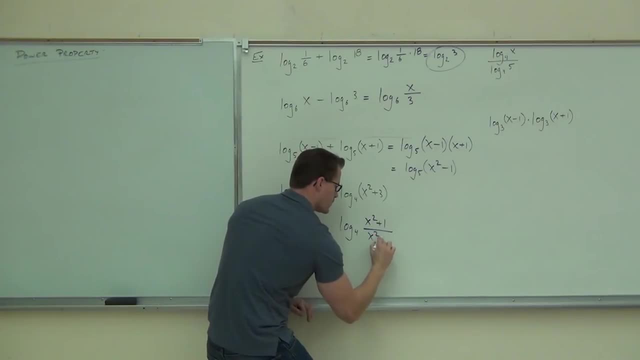 X squared minus 1.. X squared minus 1.. Denominator should be X squared plus 3.. You can't factor it. You can't simplify this one in any way, so this is exactly what you have. That's it, Richard. have you got all four of those? 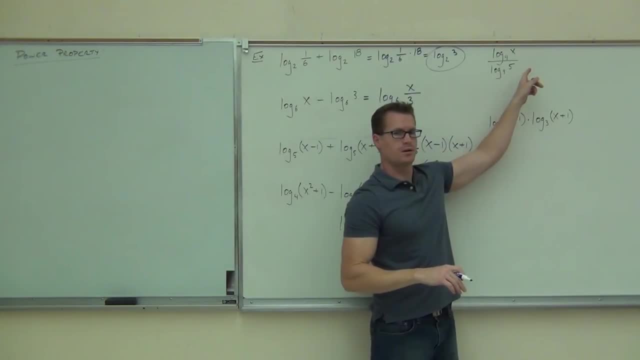 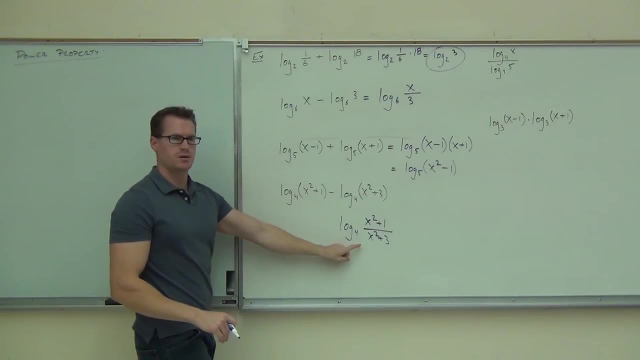 That's great, Okay, Now what can we do with this one? Nothing. Can I split this up by subtraction? No, Oh, Could I have split this one up by subtraction? No, This one, Yeah, This one is this. 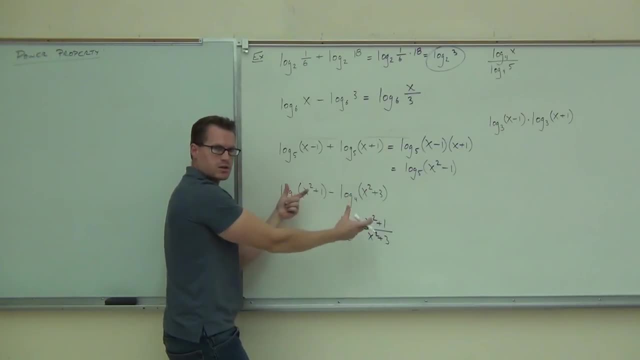 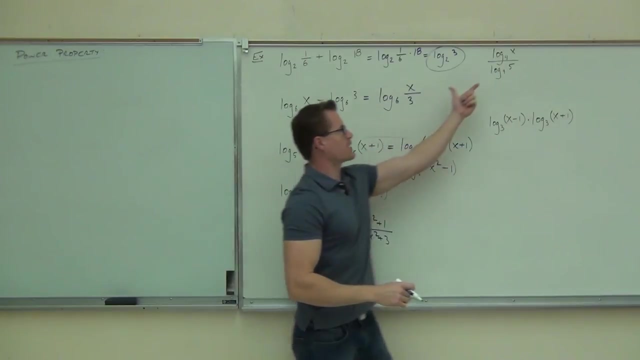 I could have split that up. We're going to be going backwards a little bit. You can do that. I mean, if you put it together by subtraction, you can split up a quotient By subtraction. Can you put? can you split that one up? 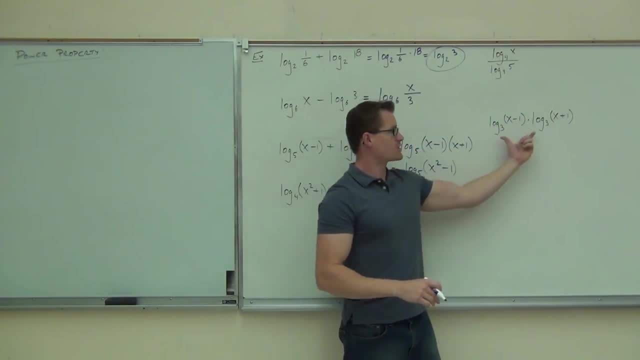 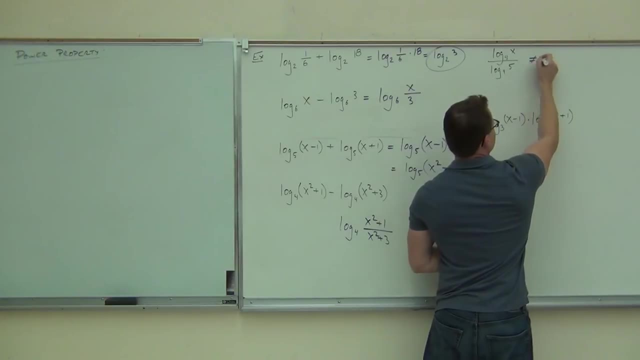 No, It doesn't look exactly the same. Can I put this together? No, No, These are the two mistakes, So we can't split this up by subtraction. Again, this does not equal log base 4 of X minus log base 4. 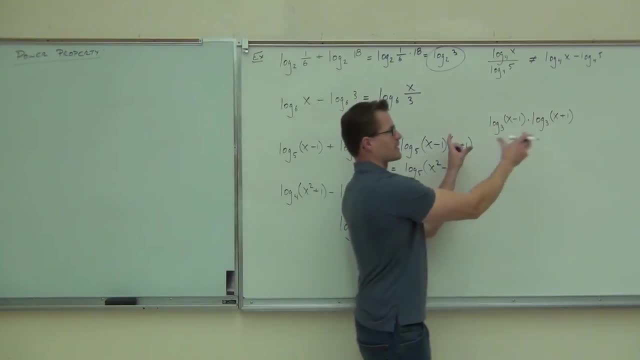 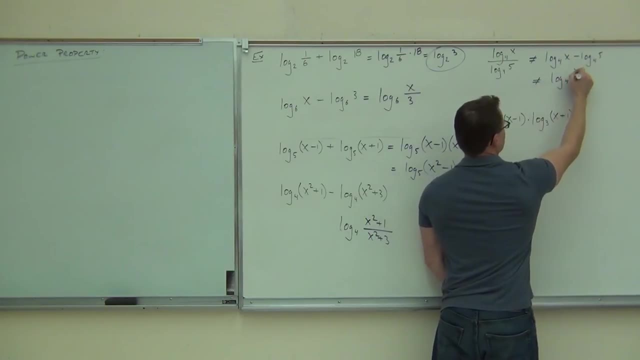 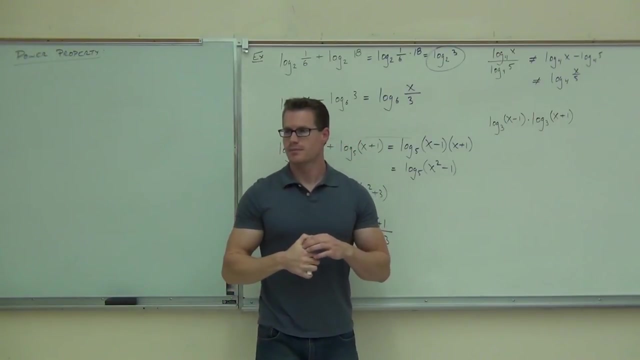 of 5.. It's not the same thing, This one. I cannot combine those either. This also doesn't equal. No, It doesn't equal either of those things. So when you ask that on a test, what do I have to put to answer that? 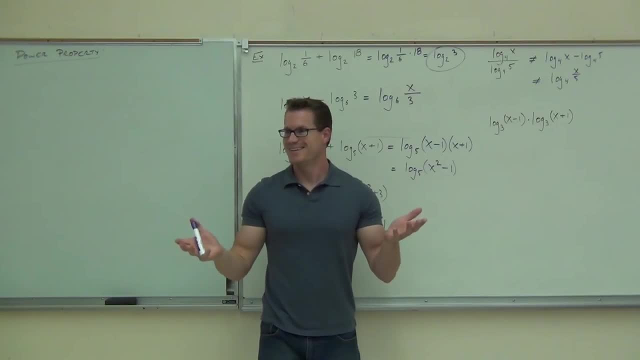 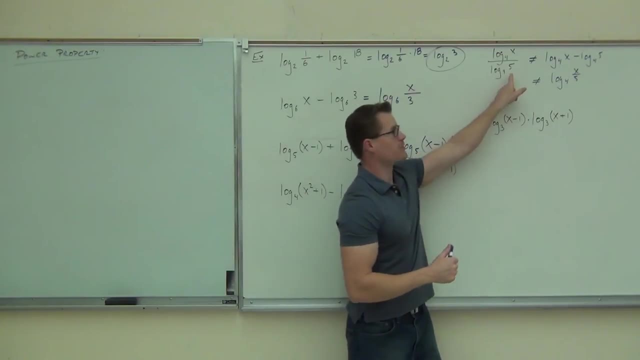 If I ask that on a test you'd go nothing. You'd say: that's as simplified as possible, That's it. You can't go any further on this problem than right there. You wouldn't show this, I mean, you wouldn't do anything about it. 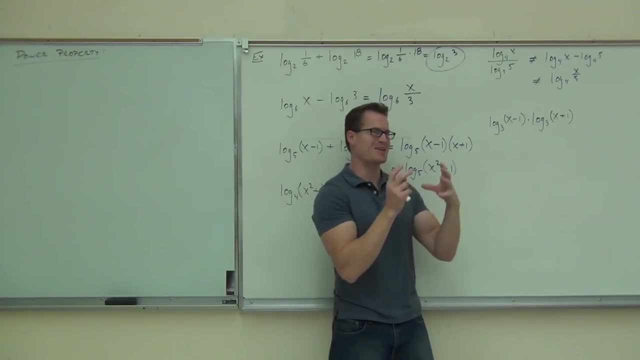 You could if you wanted to. You just want to be smart and go. ha-ha, Mr Leonard, look, I know what not to do, But just make sure you don't have it, You don't have an equal sign, because I'll be like ah-ah-ah. 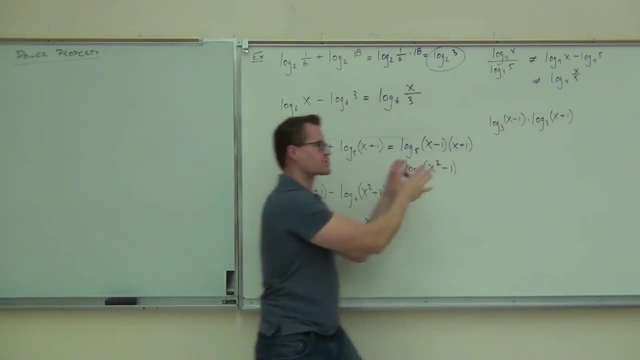 No, you can't do anything with this one. You can't do anything with this one. They don't look the same as these over here. Now there's one more property that we got to talk about Before that. are there any questions on what we just covered? 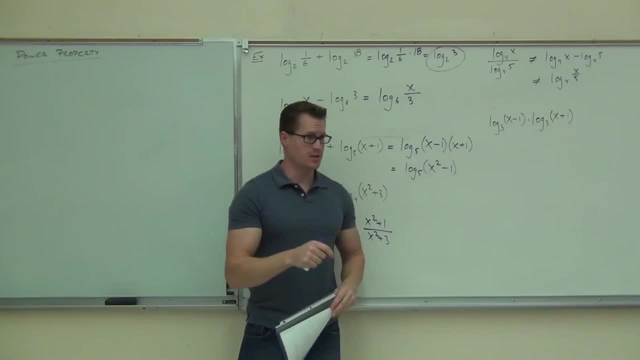 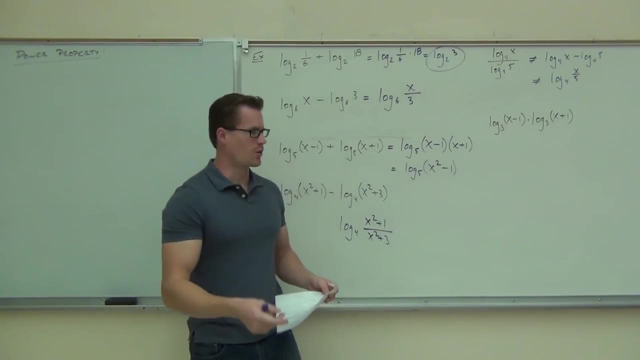 Remember. this is brand new for you. You're going to have to really memorize these properties. Are they really hard? No, No, they're not really hard. You just have to remember what you can and what you cannot do. That's the hardest part. 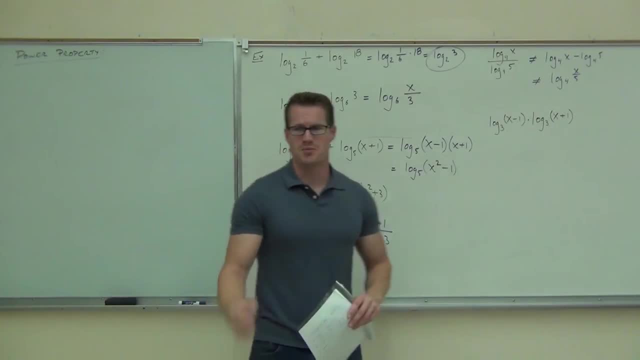 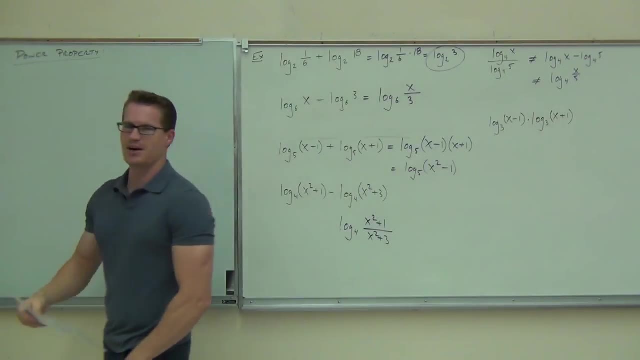 Now, the last property is by far my favorite property because it's the power of the power. I'm sorry, It's the power property, Arr, This is the best one. It's awesome. The power property is great. You're going to find out why. the power? 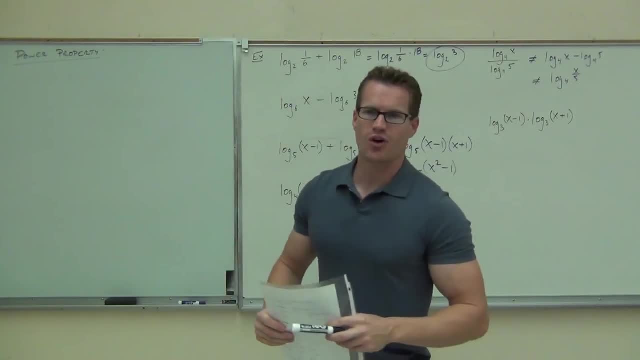 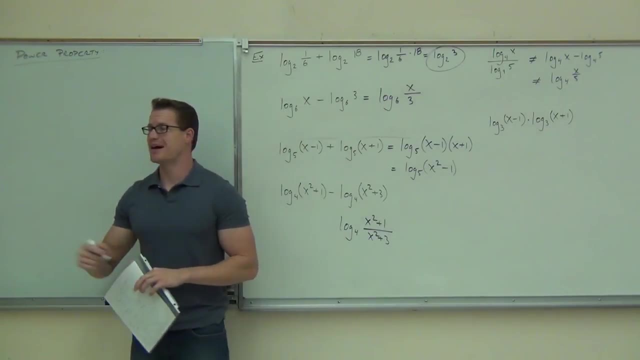 The power property is the only way that you're able to solve exponential equations. You're going to find that out in two more sections. This is the only way it works is with the power property. If you didn't have the power property, it wouldn't be possible. 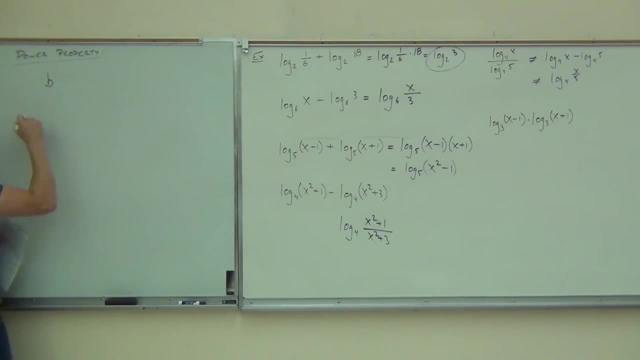 Here's what the power property says. It says: suppose you have a log Of some expression raised to an exponent. We'll call that r Log base b of x to the r. This is the coolest property. Now here's why it's the coolest property. 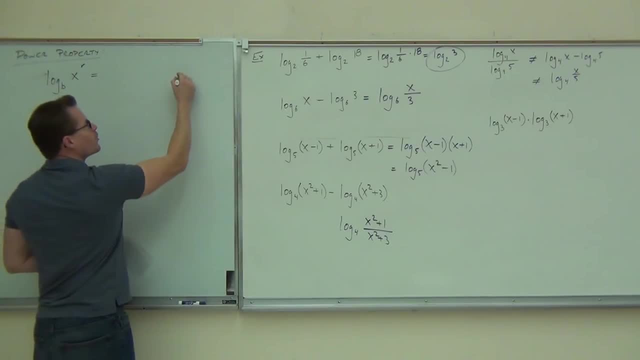 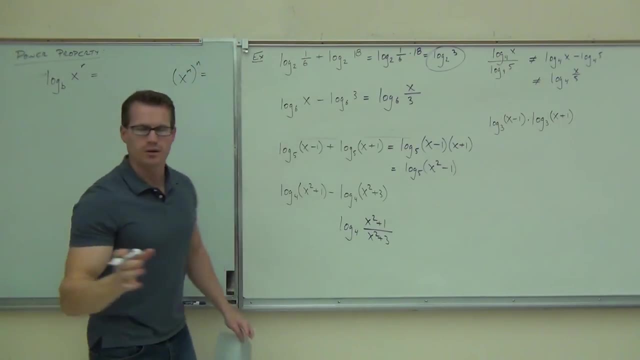 I'll do it over here with one of our rules that we're familiar with. What do you do when you have an exponent raised to an exponent? You multiply, Great. You multiply those exponents together, yes, And you get x to the. 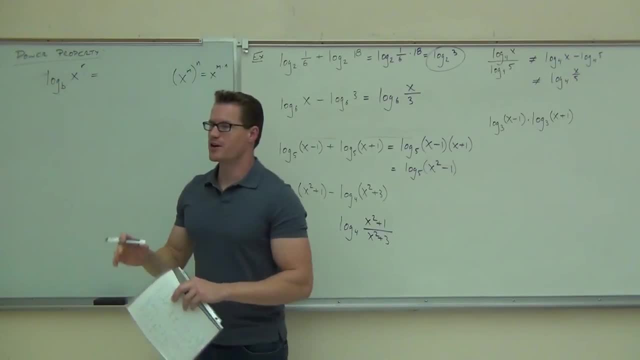 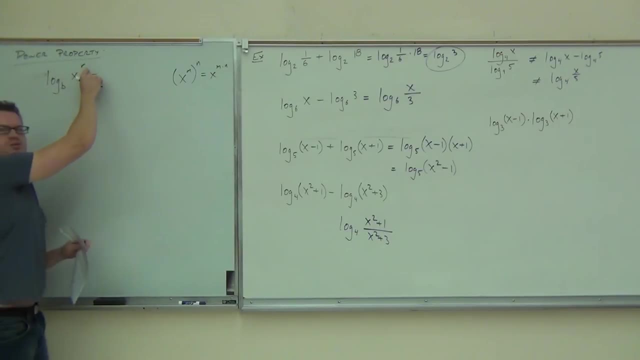 M times n. This one is going to be very similar. This is so cool. Notice how this is pretty much represents an exponent and this is another exponent. You with me on that. You multiply exponents together. Here's what this says. 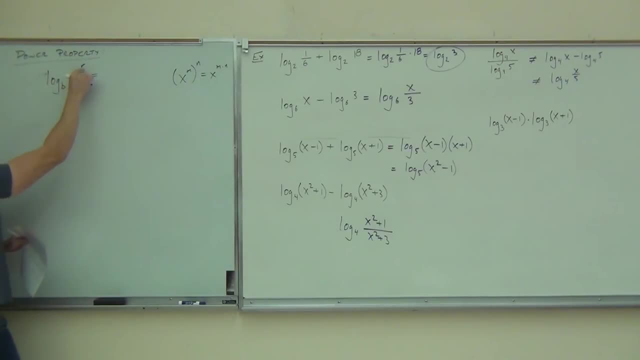 It says: if you multiply these exponents together, you can actually multiply these exponents together. Do you see the similarity? Exponent times an exponent. pretty much an exponent times an exponent. That's what that does. Is it exactly the same? 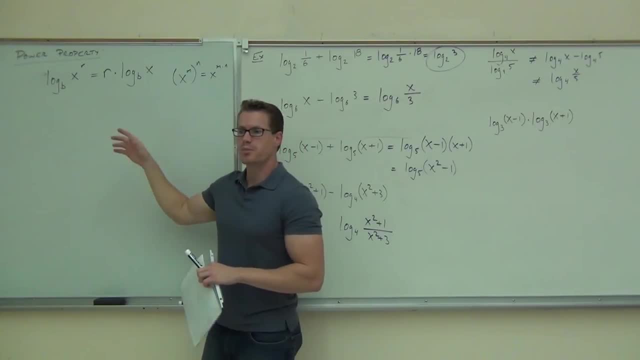 No, it's not exactly the same. Is it close? Yes, very close. You're multiplying exponents together. Remember that a logarithm. this represents an exponent. This would be equal to a value. that is an exponent. This r, that is an exponent. 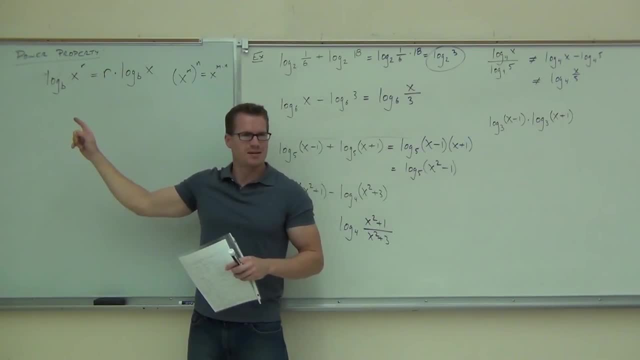 You're actually multiplying exponents together, Do you guys see it? It's kind of neat. Essentially, what it lets you do is take an exponent and move it to the right, Move it to the front of your logarithm. So do you ever have to have an exponent in a logarithm? 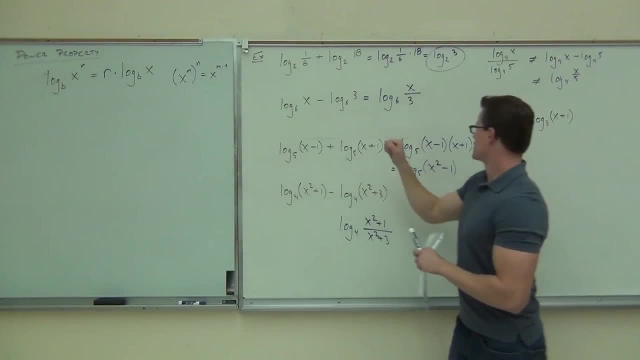 No, No, unless it's being- let's see where is it, Unless it's being added. you can't split that up at all. You're done with this one. You wouldn't be able to move anything on this problem. 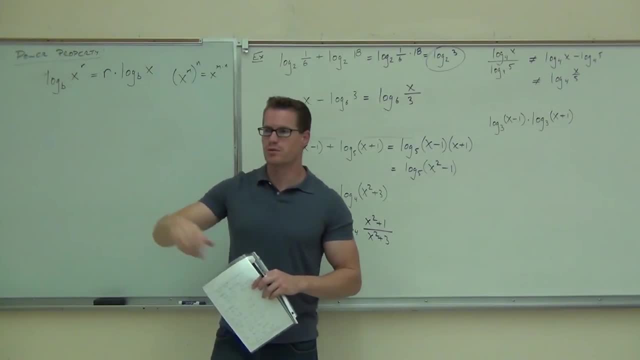 but if you have an exponent here, yeah, you can move it to the front of your fraction or in front of your logarithm. It's kind of neat. You'll see why it's kind of neat. in a couple sections Right now you're like: oh, I don't really care. 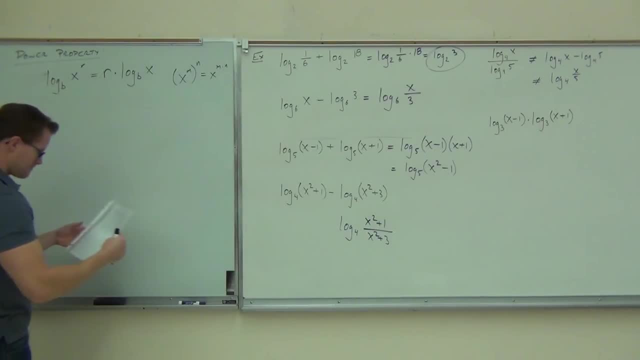 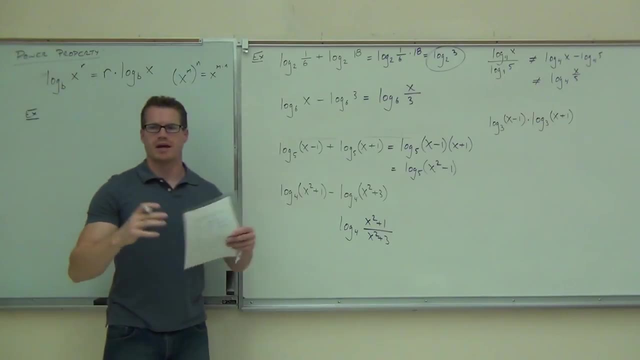 This isn't doing anything for me, But in a couple sections you're going to really care about it. All right, Let's try a few examples here and we'll get on into how to combine and expand some larger expressions. Okay, Log base 3 of x to the 5th. 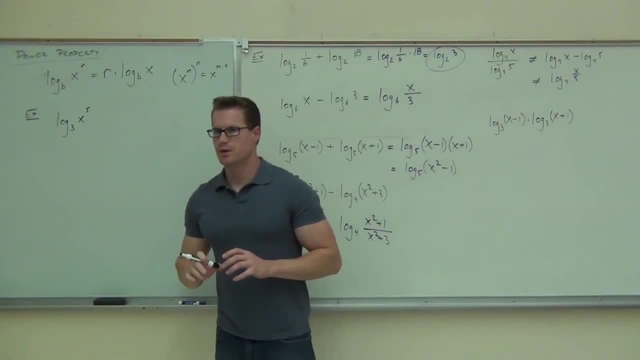 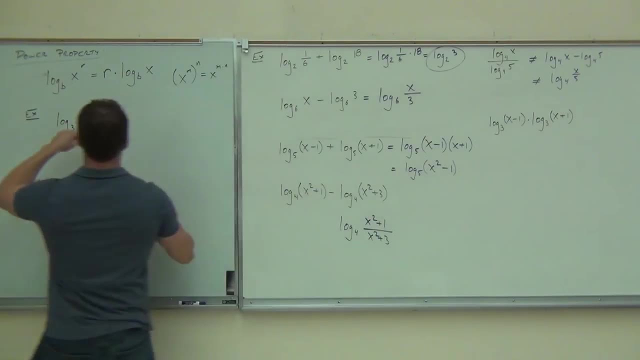 Is there an exponent there that I can move? Does it fit into the power property? Remember, it doesn't fit exactly, You can't do anything with it, but this one fits exactly. This says: I have some expression. I have some expression with an exponent. 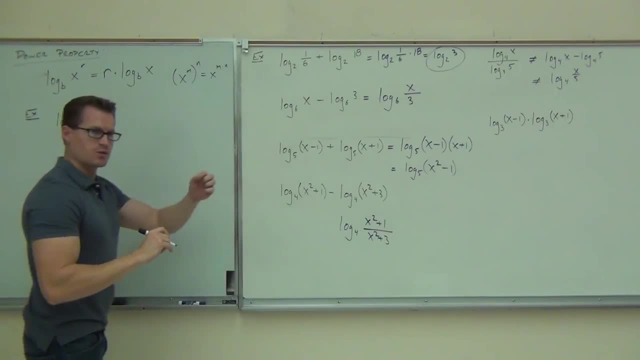 What can I do with that exponent? That's right, That's it. And it's like you're multiplying exponents here. 5 times log base 3 of x. You can put 5 times a little dot. put 5 right next to anything. 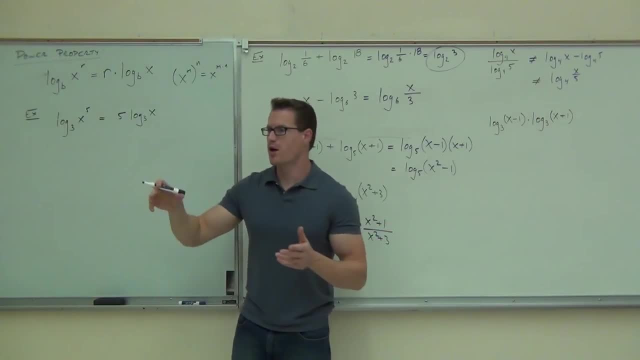 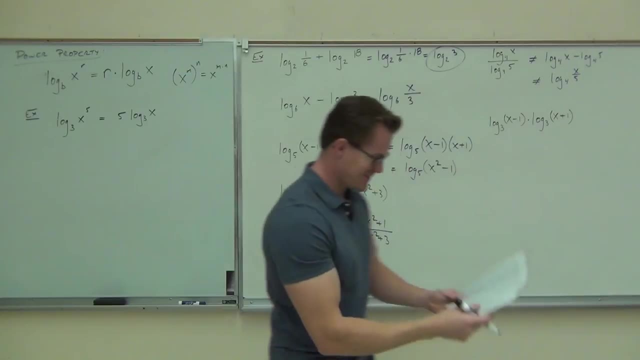 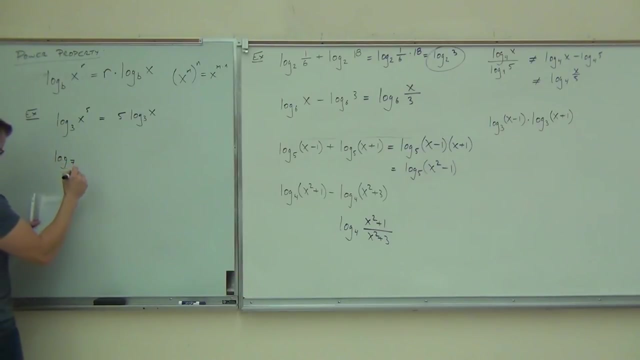 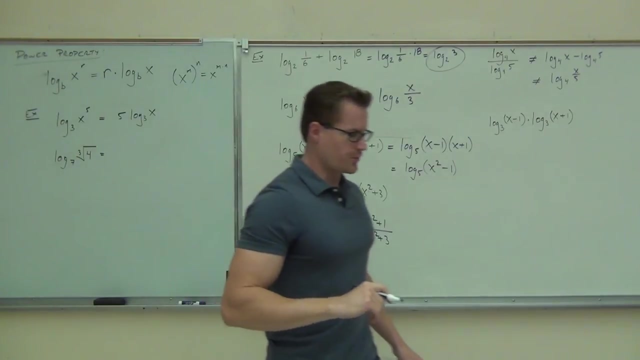 It's typically understood to be multiplication, and it is here as well. So 5 log means 5 times log. base 3 of x. You all right with that one. This is a cool one, Cool, Cool property. Okay, Log base 7 of the cube root of 4.. 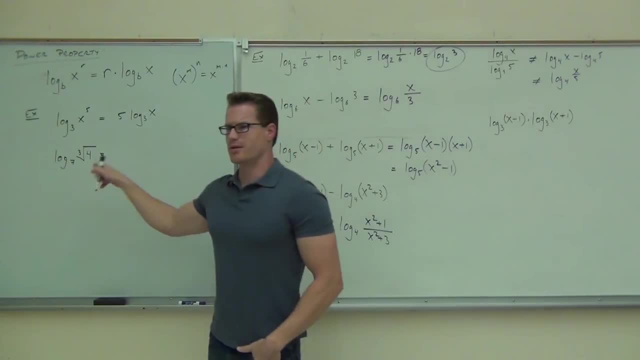 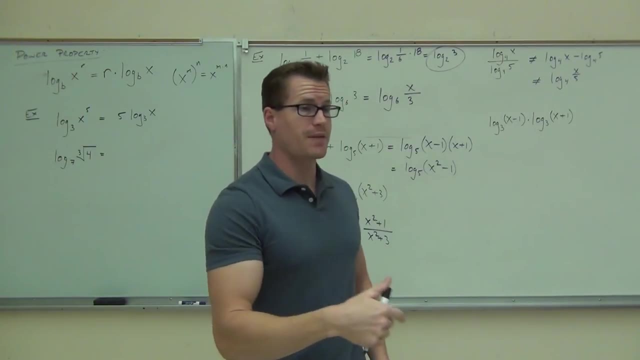 Well, now wait a second. Do I have an exponent here? Yes, sir, Oh, I do. I do have an exponent there, So a cube root. we need to go back to that chapter 10 material and we need to understand that that cube root is actually a rational. 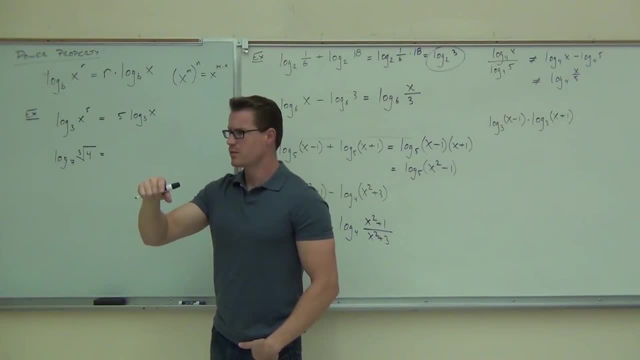 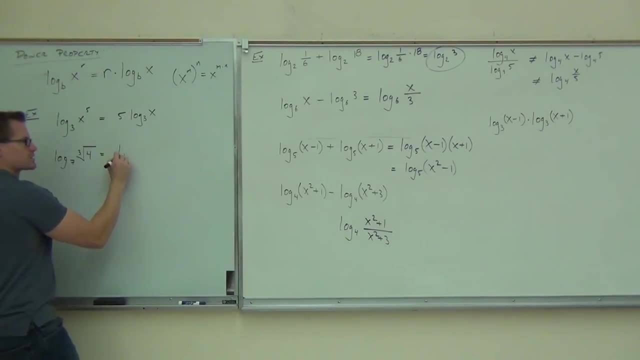 or a fractional exponent. Was it 3?? Was it 1?? It was 1- 3rd. So we need to know that log base 7 of the cube root of 4 is log base 7 of 4 to the 1- 3rd power. 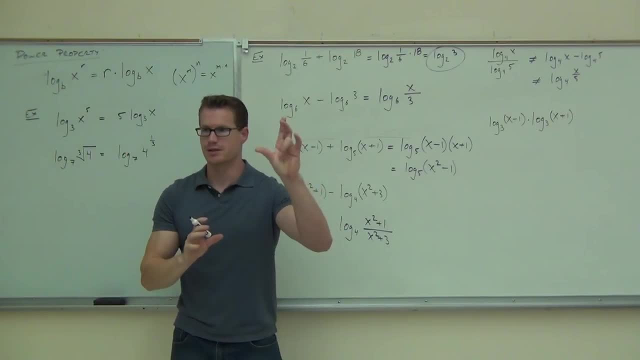 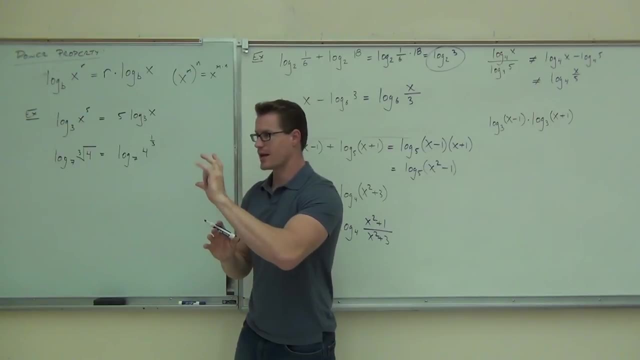 A cube root of 1: 3rd with the same exact idea when you have that 1 3rd as an exponent. Not sure if you're okay with that Now, can I still move that fraction, that exponent, to the front? 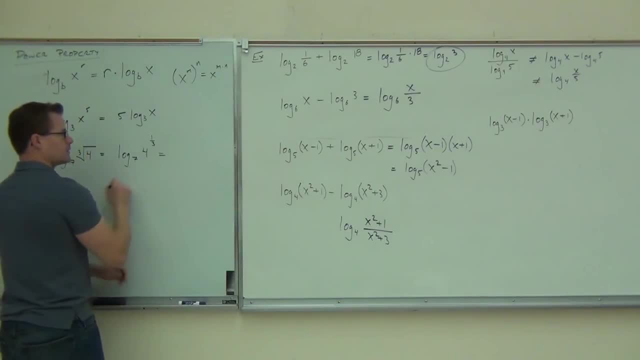 Sure, Absolutely. That's an exponent. I didn't say anything about r. It can be anything that you want. So we have 1, 3rd times log base 7 of 4.. I actually don't even need that multiplication. 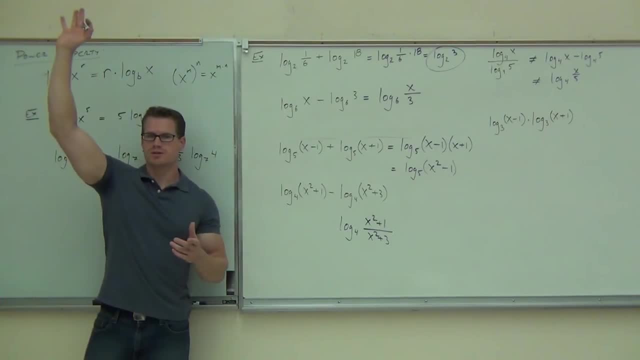 That's your answer. 1, 3rd times that logarithm. How many people feel okay with this? so far, Good deal. Now there's one more thing. This is kind of interesting here. Hope you don't get confused by this. 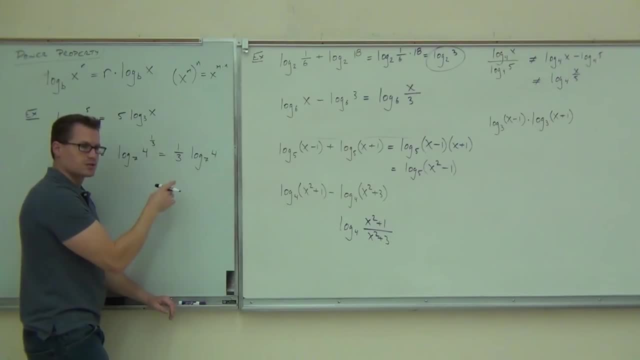 but you could occasionally write this a little different. Let's say you have 1 3rd times that expression. That's the same Same thing as log base 7 of 4 all over 3, not 4 3rds, not 4 3rds. 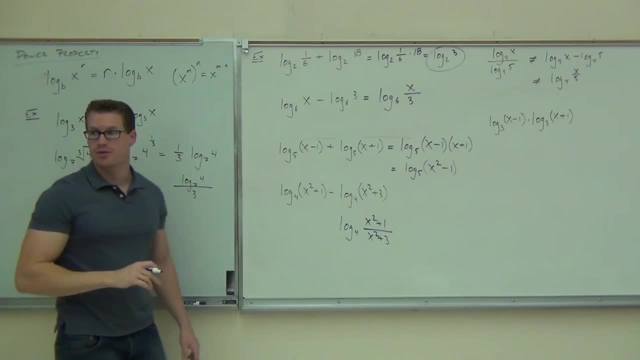 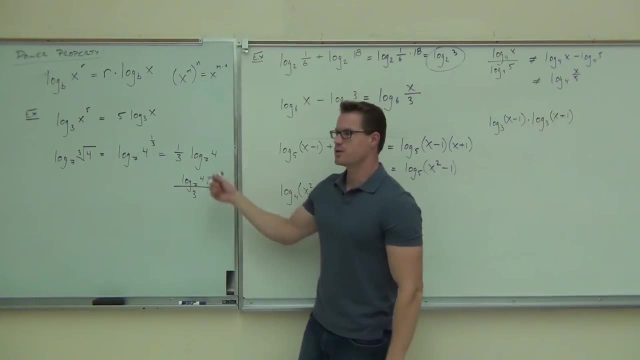 You can't just divide the 4 by 3, but the whole logarithm divided by 3, that is appropriate. That is 1- 3rd. Are you okay with that one? It's a little bit of fraction work. Typically you'll see it written like that: 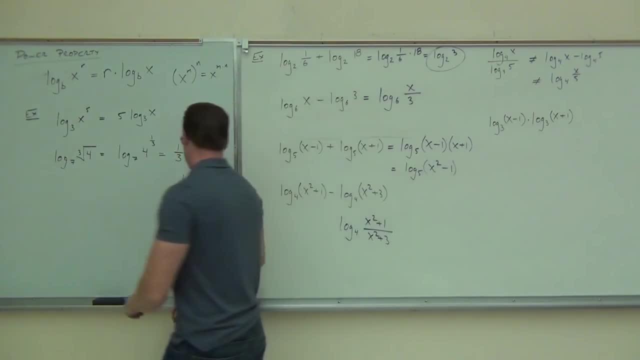 Okay, Typically this will work. Okay, Try a couple of these on your own. Let's do. let's see That one and that one There. 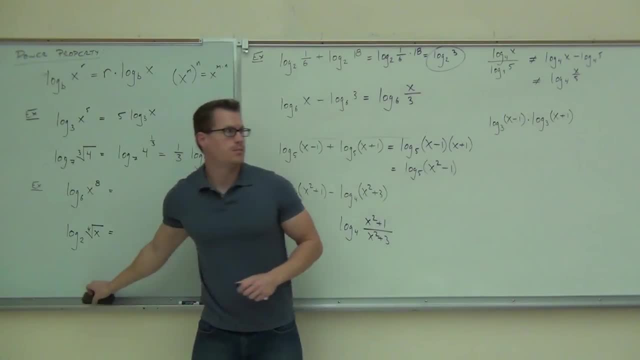 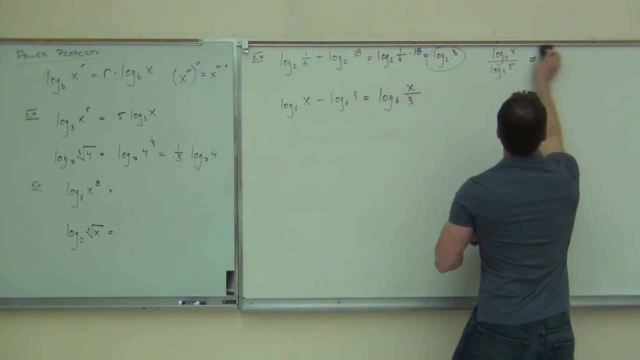 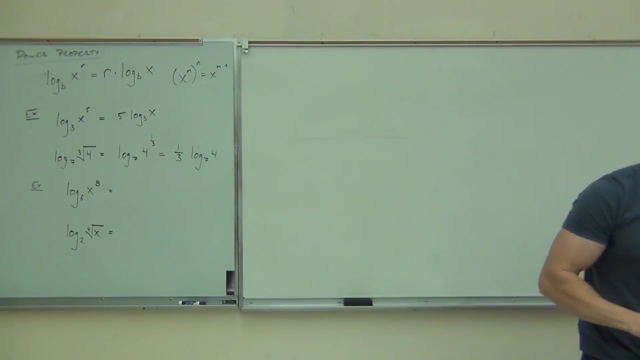 I just don't know what I want to say. Okay. 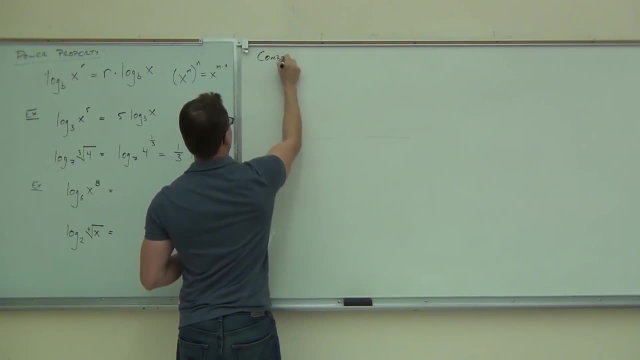 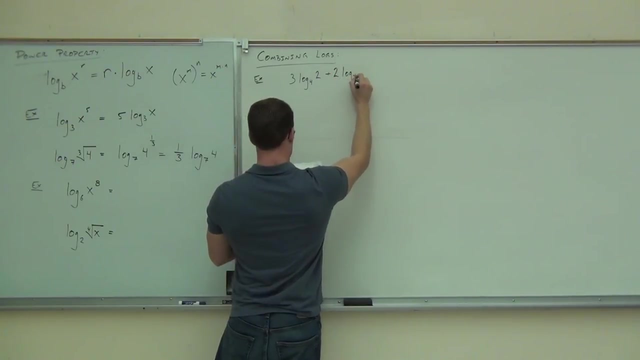 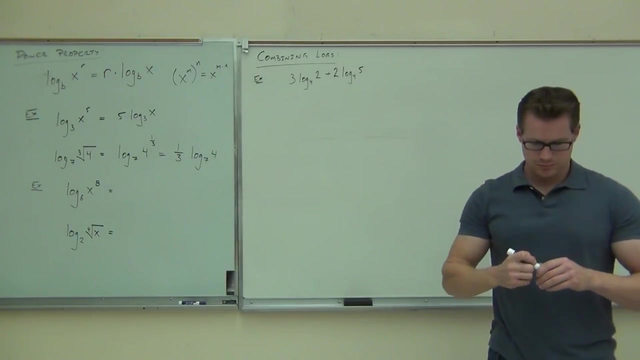 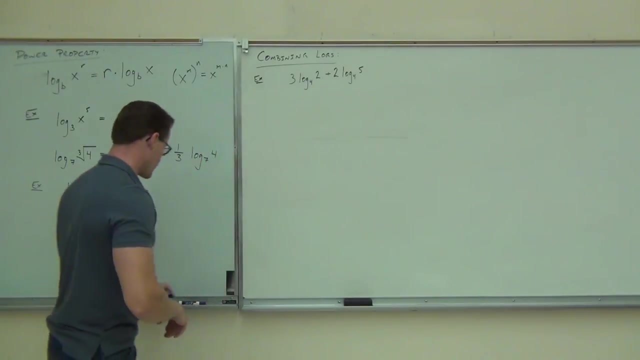 And, of course, right, Yeah, Okay, Okay, Are you done? Mm-hmm, All right, Good, They're pretty quick. these power properties, Since we have an exponent here, we know that our power property says any exponent can be. 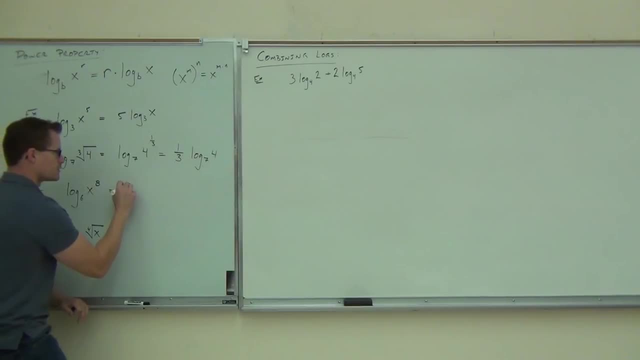 moved to the front of our logarithm and be multiplied, so we'll have 8.. Log base 6 of x: Here we do need to change that to an exponent before we do any more work. so we do need to know absolutely that this is really log base 2 of x to the one-fourth power. 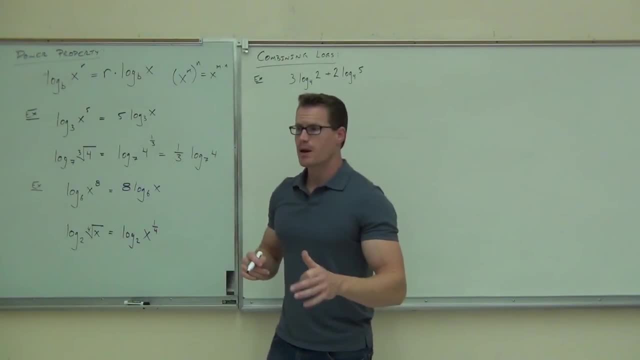 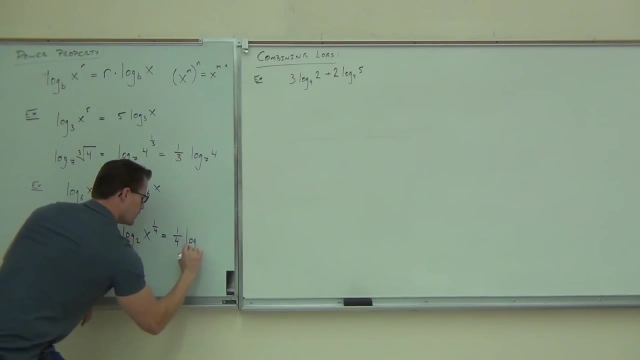 Did you translate that appropriately as well? to the one-fourth power? Yes, Then since we have the exponent, we can move it to the front of our logarithm. You'll get one-fourth log base 2 of x. Could you write this whole thing as over 4?? 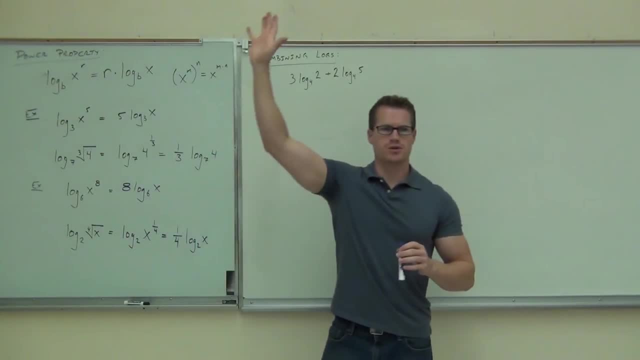 Yeah, that would be appropriate as well. Raise your hand if you got both those correct. Do you feel okay? on the power property, the product property and the quotient property, That's it. That's the only three we have. That's the only thing you can do with logarithms: to expand them or combine them. 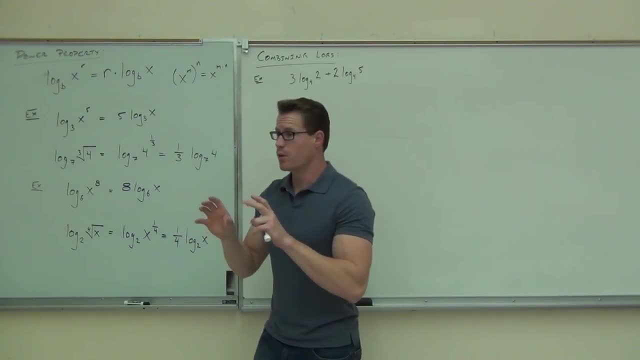 If you master those three properties, if you know that the only thing you can do is do things that look exactly like those three properties, you're done. This whole section is just manipulating them. now Let's go back and let's look at some of these examples. 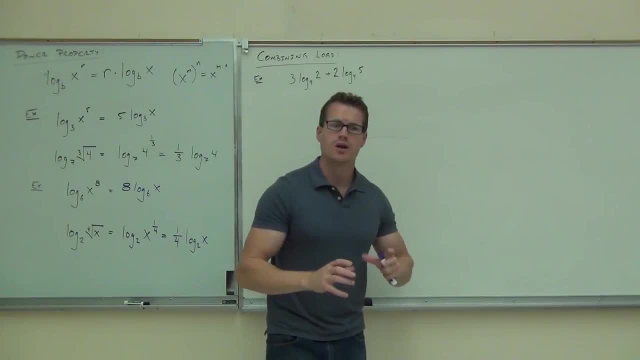 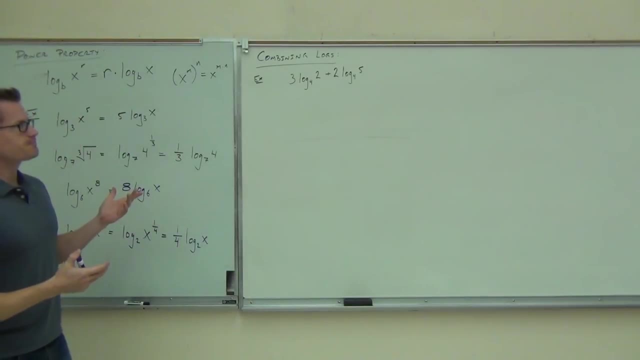 Let's see if we can use some of these properties in conjunction with each other to put together some logarithms or to expand some logarithms. We'll talk about combining them first. Now, when we're looking at that, do you see any exponents or some numbers that could be exponents? 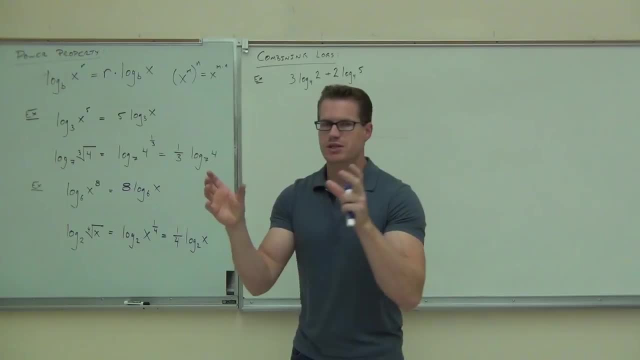 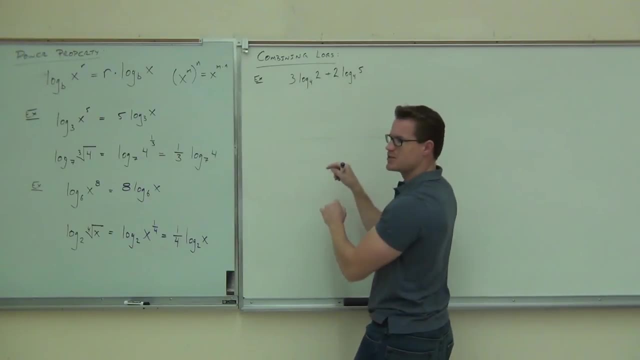 Before we start combining logarithms, like our products and our quotients, we've got to take care of any numbers in front of our logarithms. You see, we can't just directly combine these by multiplication yet, because we don't have. if you look right at your properties, on your product property it said a log plus a log. 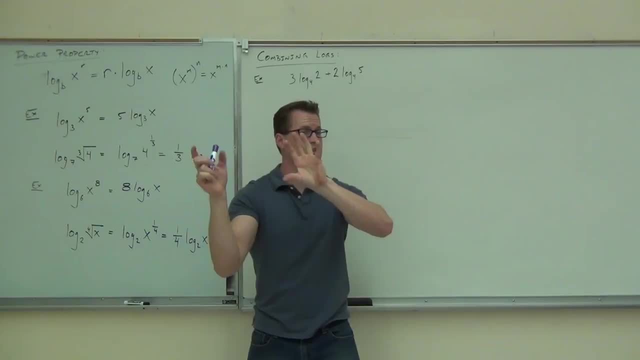 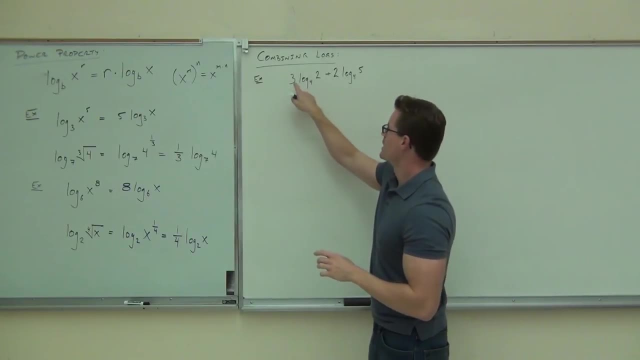 right, Not a number in front of a log. That didn't compute. You've got to change those to be a log plus a log in order to combine them first. Take care of those numbers first. First thing we're going to look at is do something with the three and do something with the two. 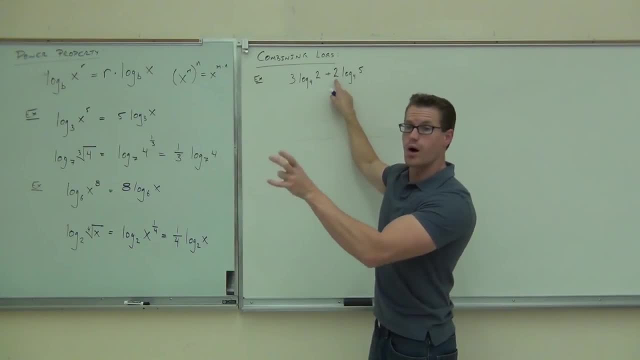 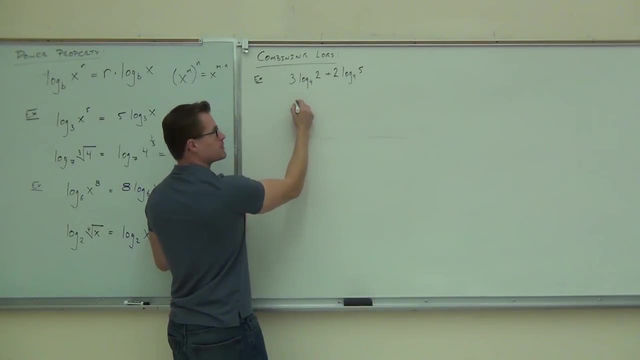 here. Make them so that you have a log plus a log or a log minus a log. if you're going to use the quotient rule In our case right now, we could make this: what please? Log base four: okay, two to the what now? 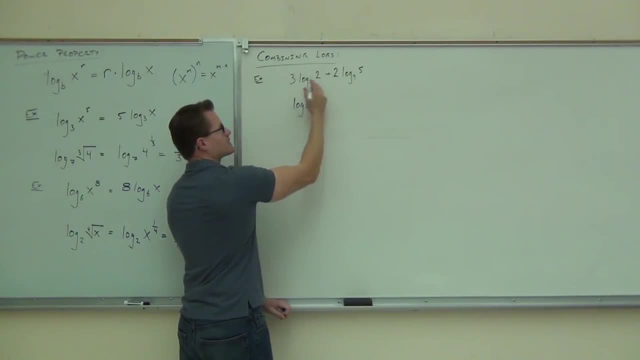 Two to the third, that's right, So that three, that is an exponent. Any number in front of a logarithm is automatically an exponent. It's kind of weird, right, You look over here, but that's what that says. 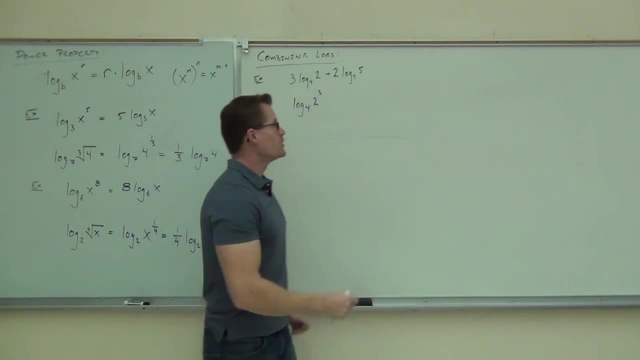 It says r is an exponent. It's kind of cool. You can move it and make it an exponent Plus, because we have a plus, We'll also move that two log base four of five to the second. You see what that does is it makes it so I have a logarithm plus a logarithm. and now 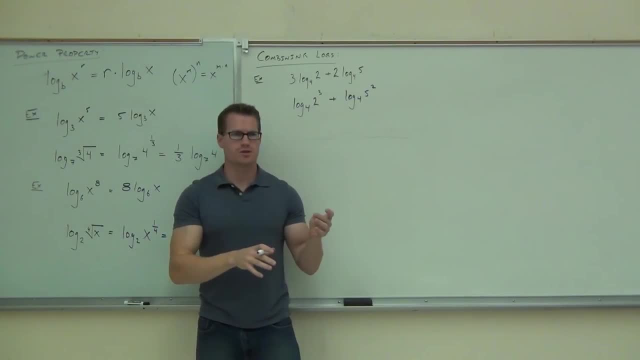 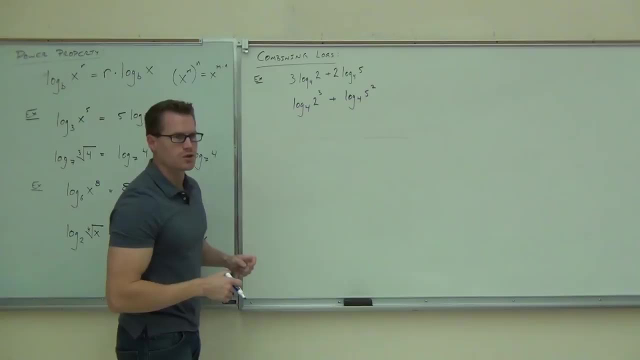 that does fit into another property that we have. You guys all right with this so far. So when you're combining, your exponents come first, just like order of operations. Then you look for anything else that you can do Now. could you make that into an eight and that into a 25?? 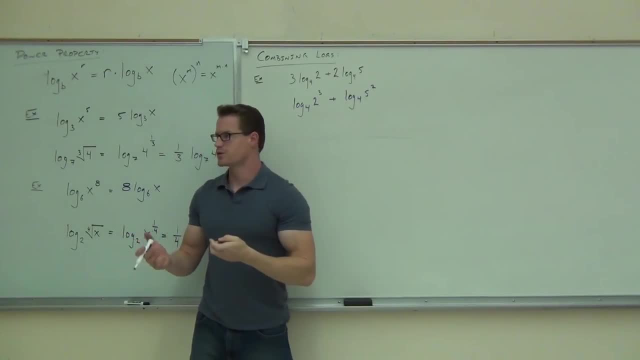 Absolutely you could. Don't forget that. two to the third power, that's always eight, That is okay, and five squared is 25.. I'm going to leave them just so you see where those numbers are going, but on your paper, 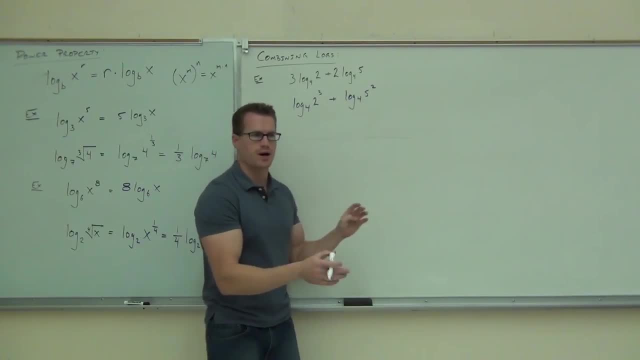 you could put, like on your test or something, eight over 25 on your homework, eight over 25.. Now can I combine these? Do they have the same base? Sure, They're being added. Can I combine addition of two logarithms. 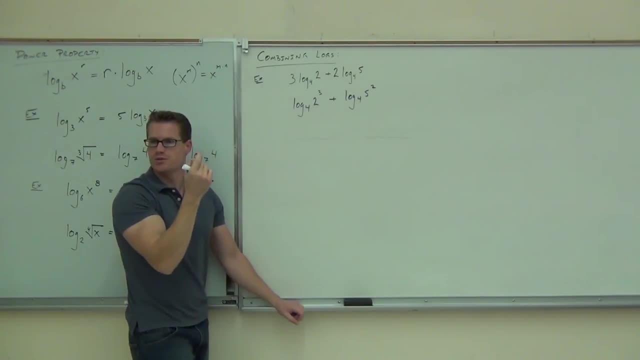 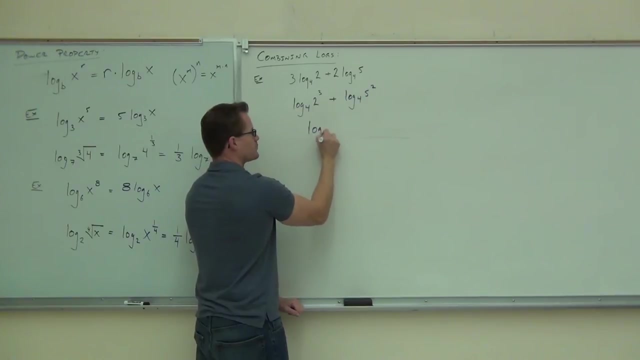 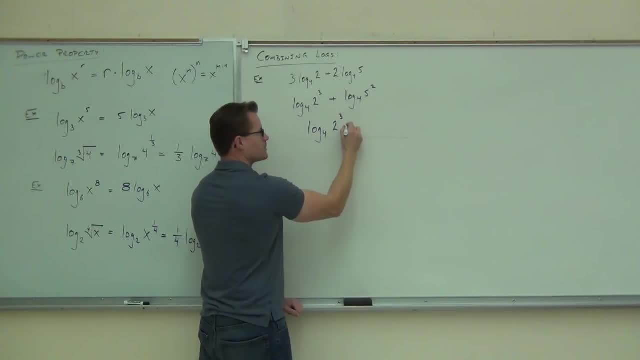 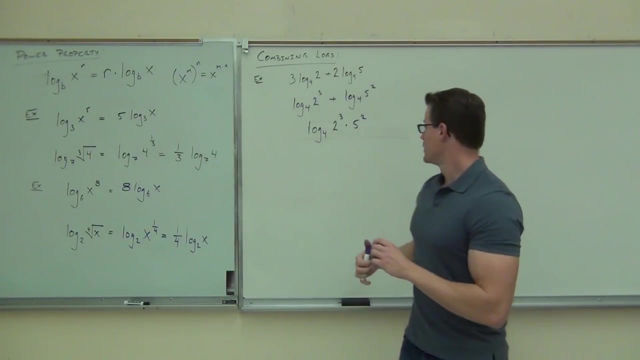 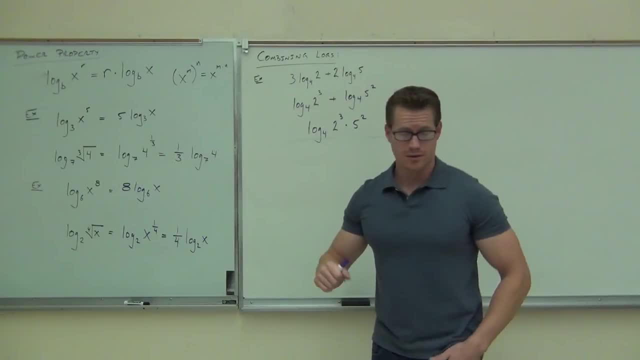 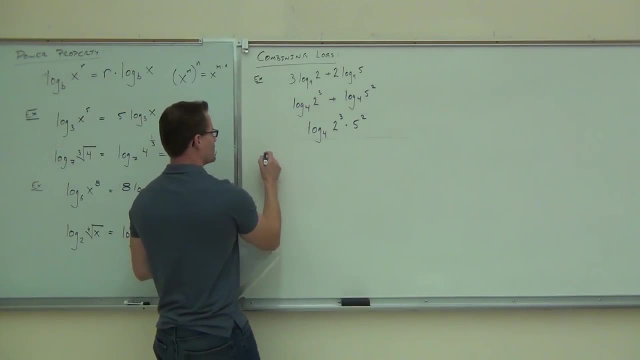 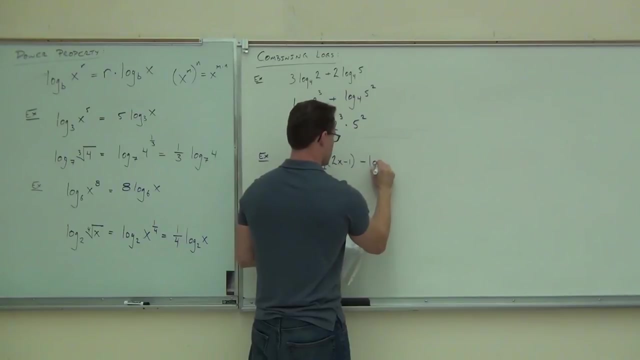 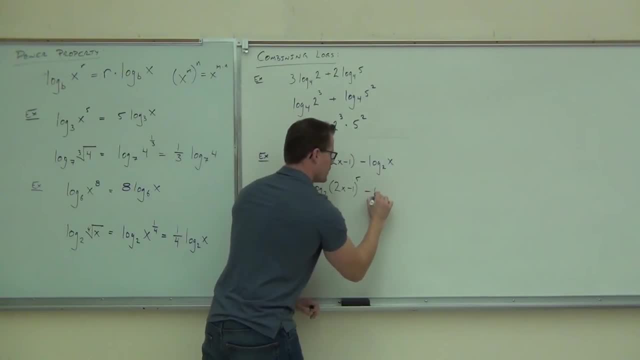 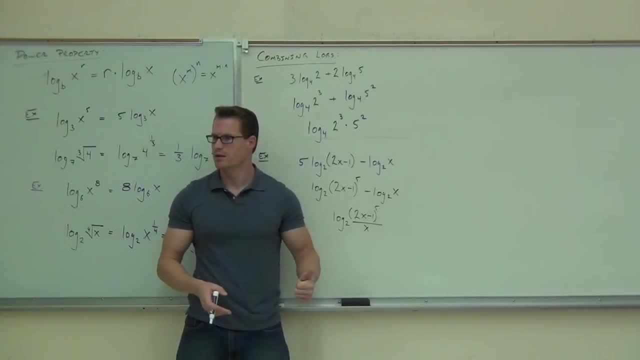 That's it. That's as far as you can go. You're definitely not going to want to distribute that right. You don't want to. that'd be horrible, really, really nasty. Let's try one more. I'll give you a couple. do one on your own. 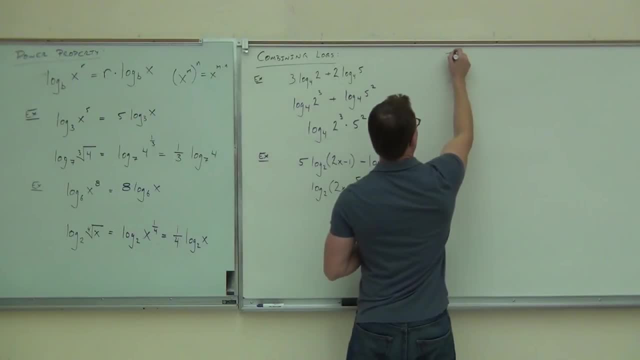 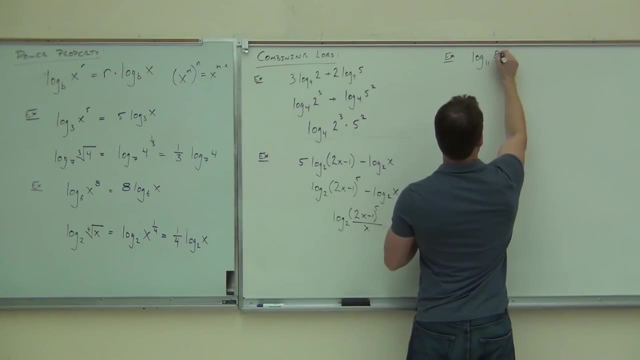 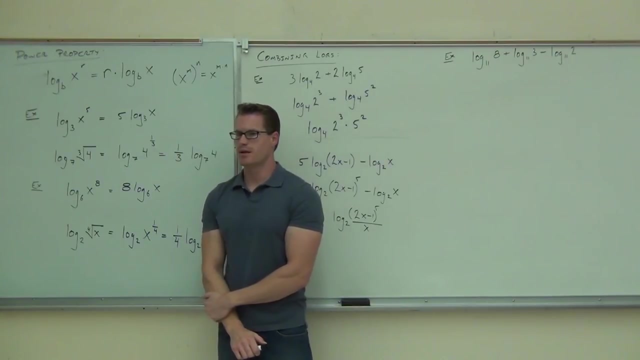 We'll talk about expansion and then we'll be done. Do I have any exponents to deal with in this problem? Well, it's kind of nice. I don't have that little deal that I got to do. That's not bad. 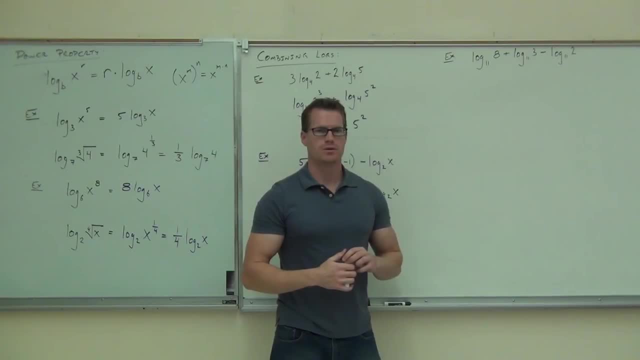 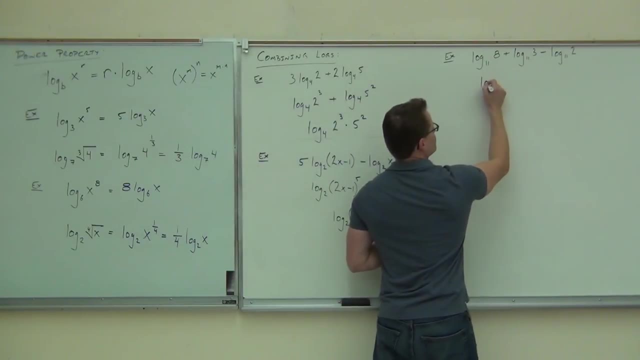 What can I do? Sure, The addition one gets combined as what. So the first two? I could do log base 11 of 8 times 3.. All over 2.. All over 2,. great, because now I have log base 11,. 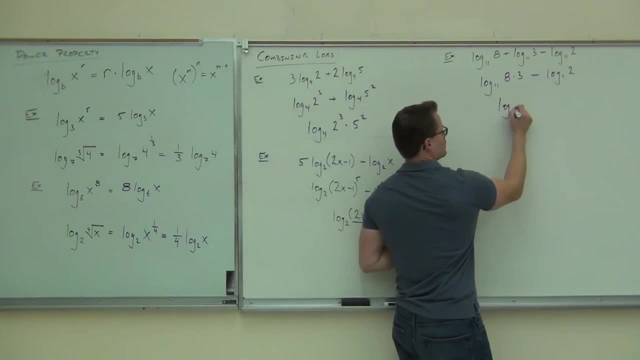 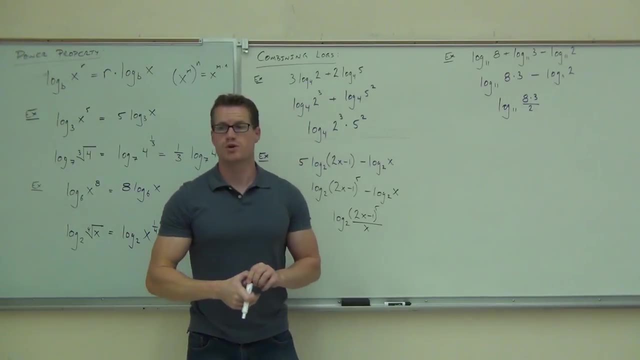 log base 11 to be subtracted: Log base 11 of 8 times 3 over 2.. Of course, could you do the math on that. Sure, you're going to get what? 12? 12. You're going to get 12 out of that. 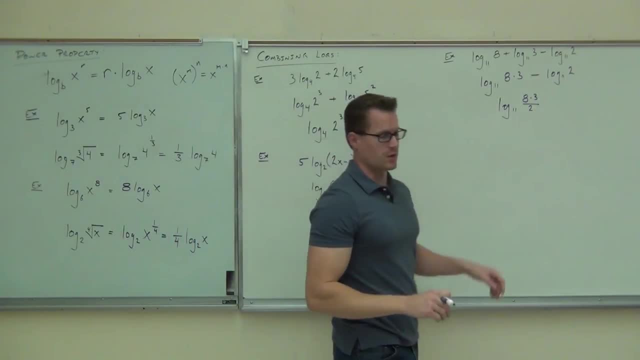 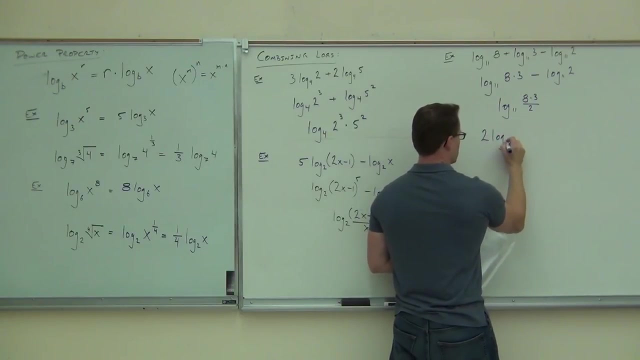 Log base 11 of 12.. You can show that if you'd like. This is combining. Why don't you try a couple of these on your own? Let's do 2 log base 5 of 4 plus 5 log base 5 of 2.. 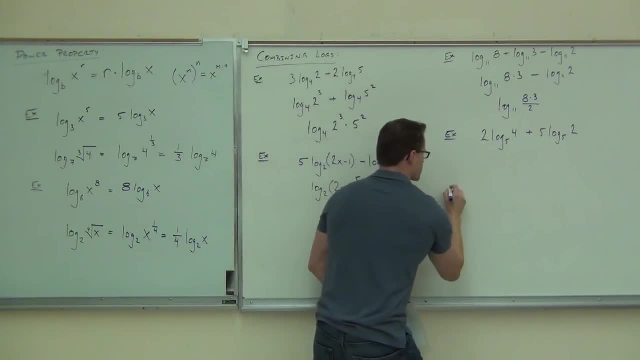 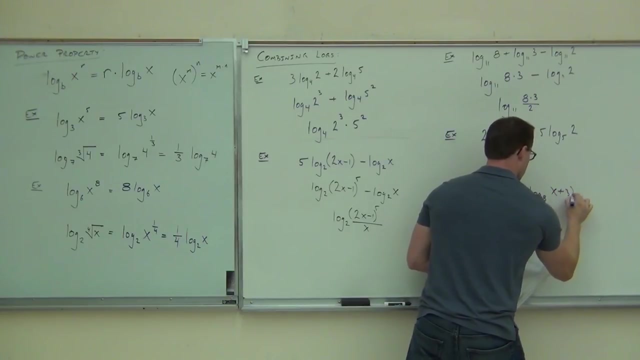 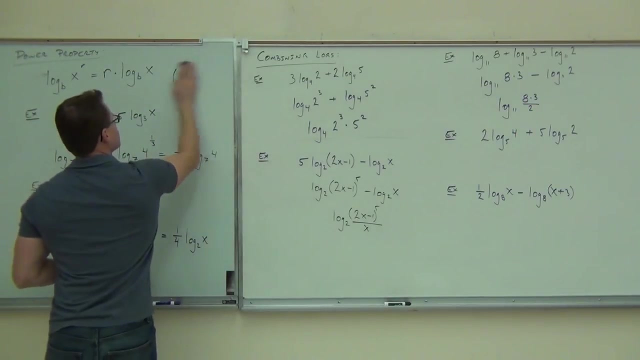 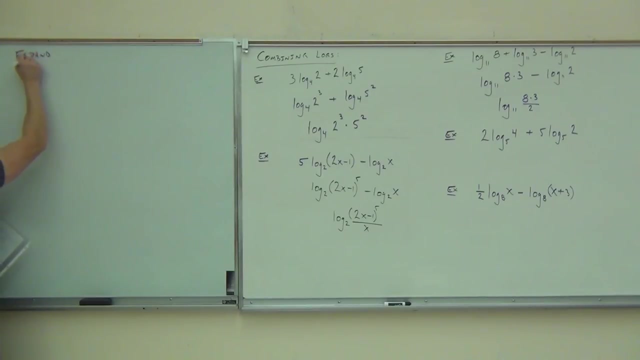 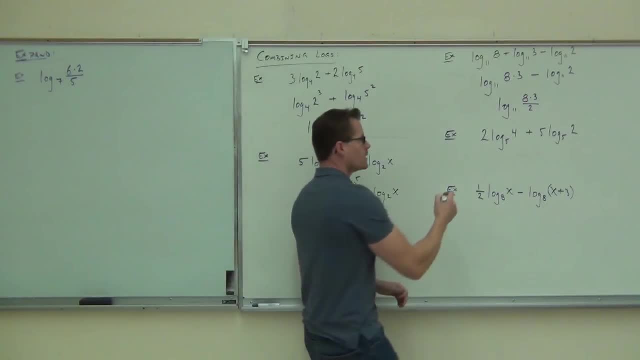 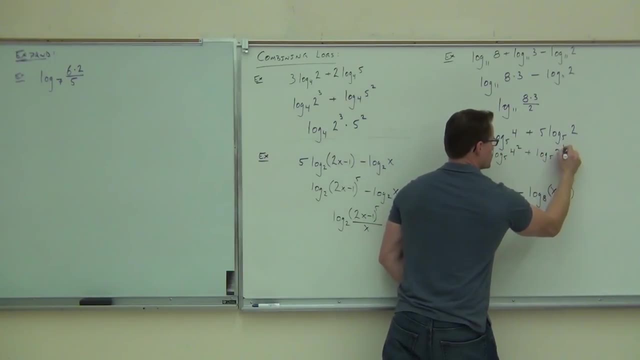 You cannot combine logs. if there are numbers in front of your logs, You can't do it. So here we have to do first log base 5 of 4 squared plus log base 5 of 2 to the 5th. 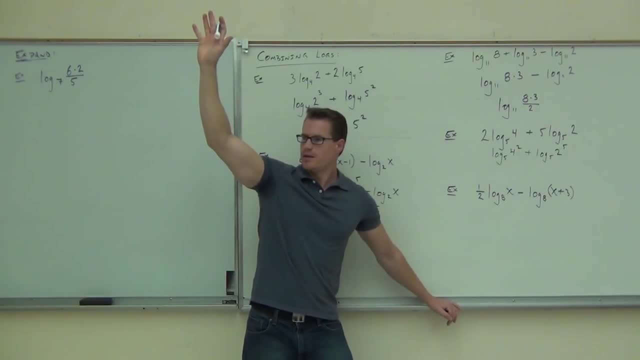 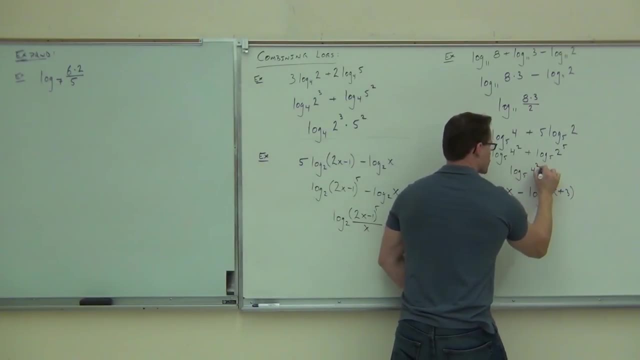 Raise your hand if you made it that far. Good deal, You did that first. Now we have a log plus a log with the same base. We can also combine that by multiplication. That will be log base 5 of 4 squared times 2 to the 5th. 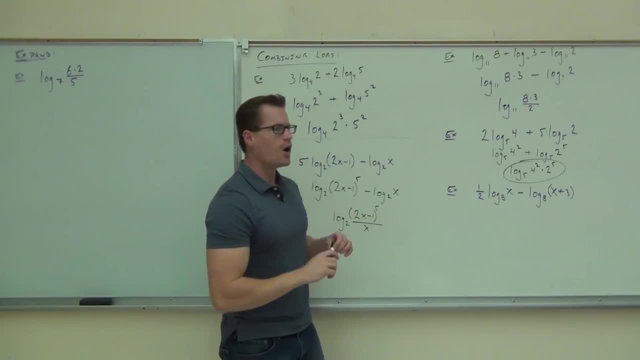 Log base: 5 of 4 squared times 2 to the 5th On your paper. you can actually do the work and get. what is that? 16 times 32, whatever that happens to be on your paper. Okay so far. 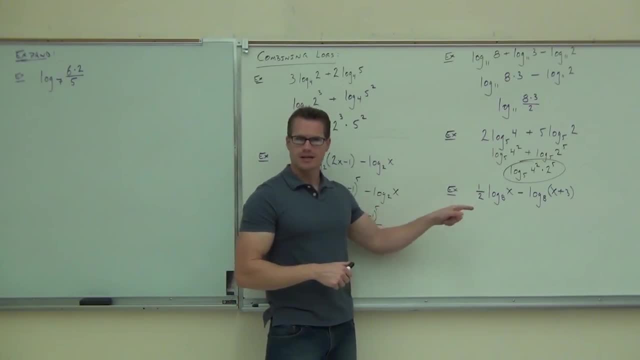 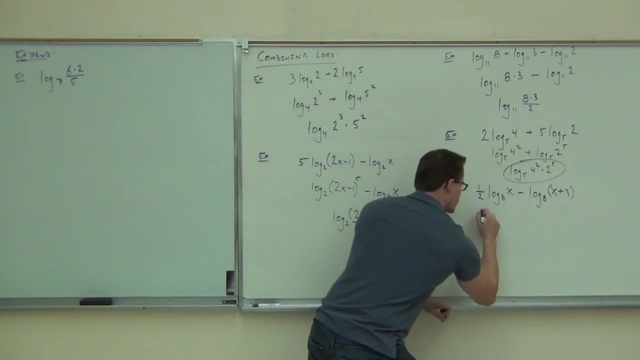 Okay, next up. What about the 1 half? Is that still an exponent Square root? Yeah, that's actually a square root. You can change it to a square root if you wanted. You see, when you move that as your exponent. 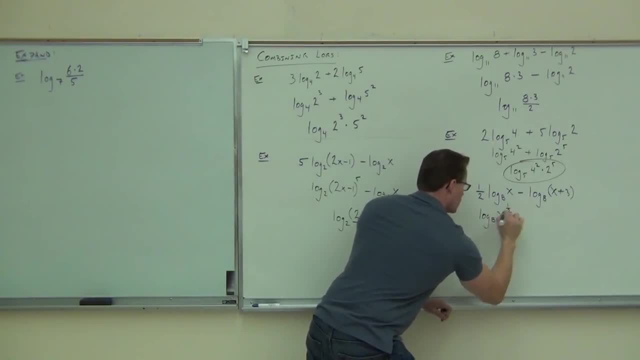 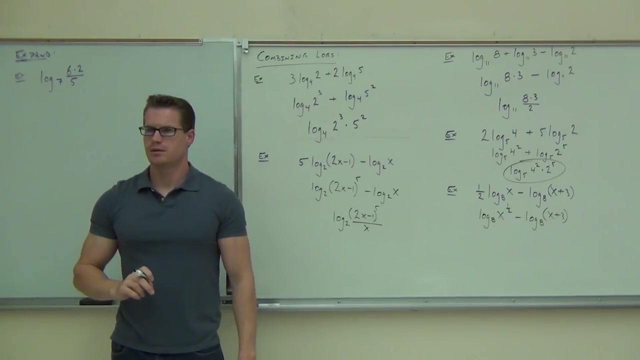 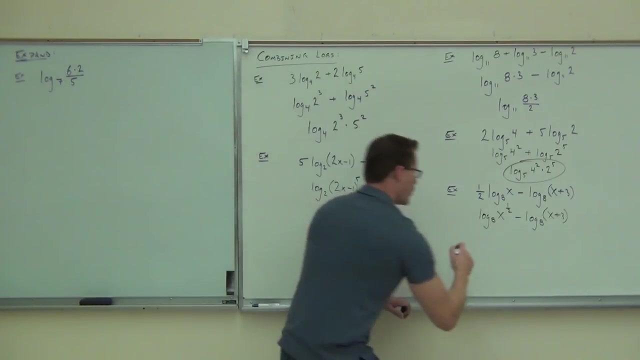 you'll have log base 8 of x to the 1 half. Those fractions can still move up as exponents. Is there anything else we can do on that? Sure, Is it going to be a product or a quotient, So we should have one logarithm. 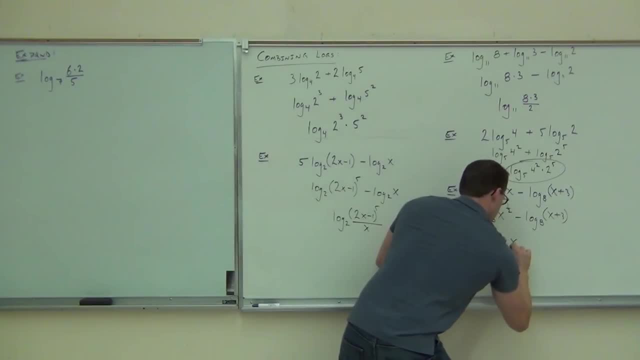 What's going to be on the top of our logarithms? Square root of x. Sure, x to the 1 half. or you could write square root of x. That's fine, because x to the 1 half is a square root of x. 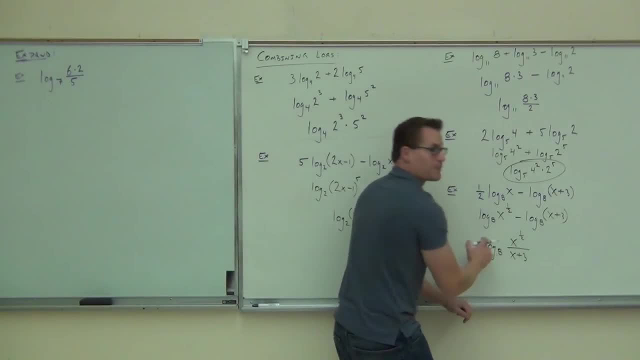 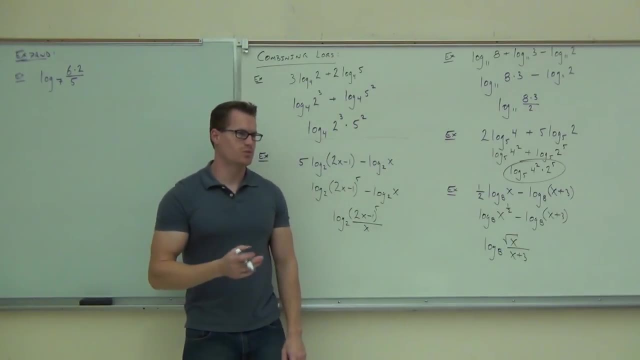 Just like that. So either the 1 half right there, or, if you want to be fancy about it, let's say, hey, look, Now it looks cooler. You can do that too, because that 1 half power is a square root. 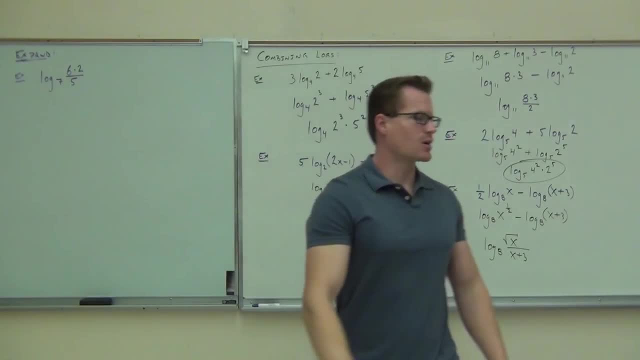 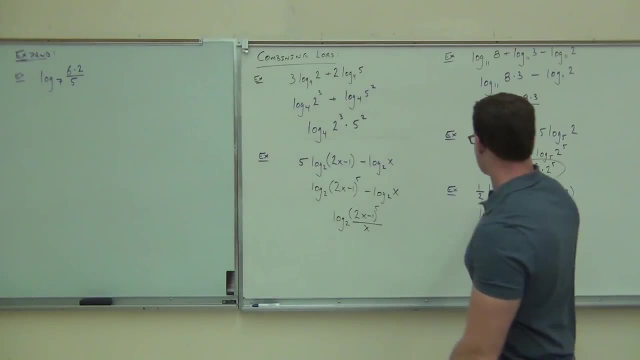 Richard, do you feel okay with this combining of logarithms? Now? the last thing we're going to talk about is expanding logarithms. You also need to go backwards, Be able to take these things and make them into those. Be able to take this and make it look like that. 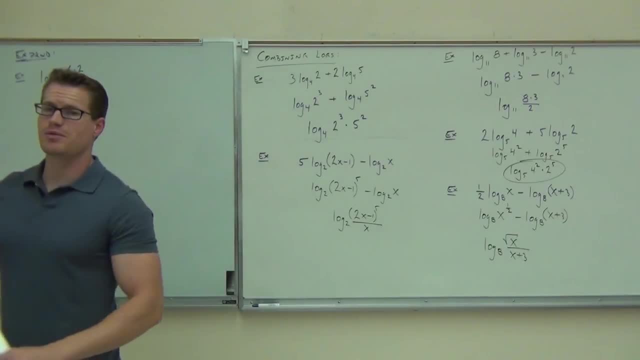 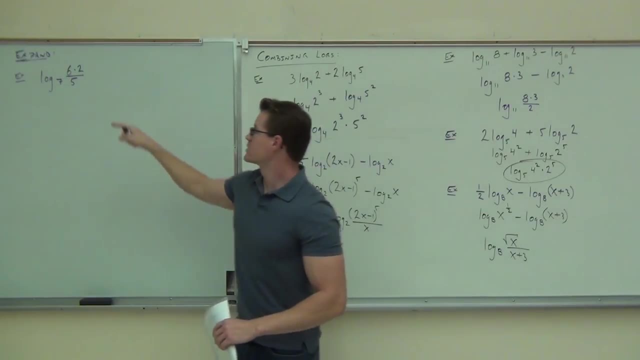 Expand it as much as possible. Let's practice that here. Do you see some things that we can expand? Do you see some things that we can expand? Can you expand a quotient Work from the outside in? Okay, work from the outside in. 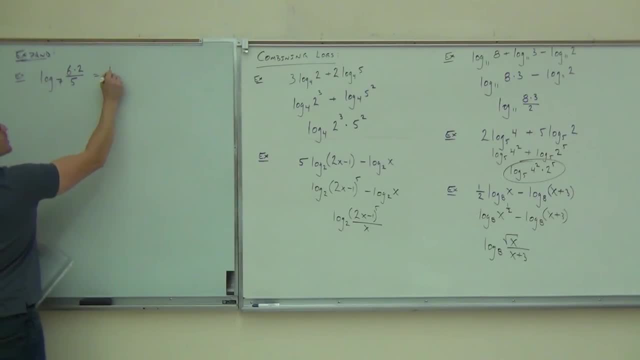 So the first thing I'm seeing here is a quotient. So I know that this is going to be log base 7 of 6. So log base 7 of 6 times 2. Is it going to be over log base 7 of 5 or minus? 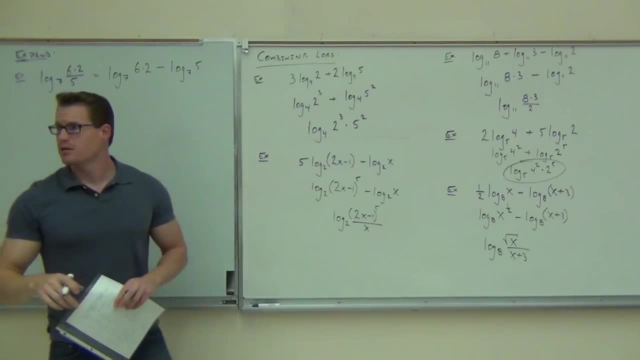 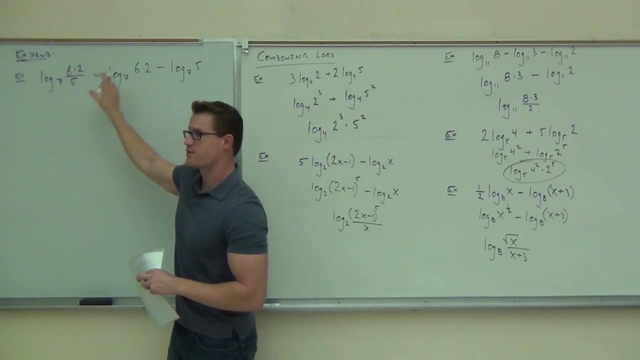 Very good, That's how you put it together right? That's how we did that example right over there. We put it together as log base 7 of 6 times 2 over 5, so that's how we split up by that subtraction. 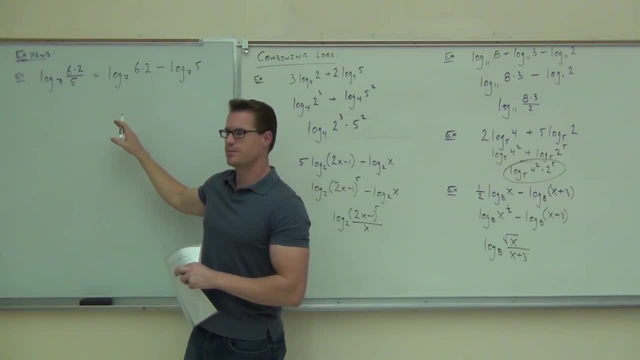 Are you guys okay with that so far? Now, is there anything else we can do? Yeah, so 6 times 2.. You definitely can do that. So, all in all, this is going to be log base 7 of 6 times 2,. 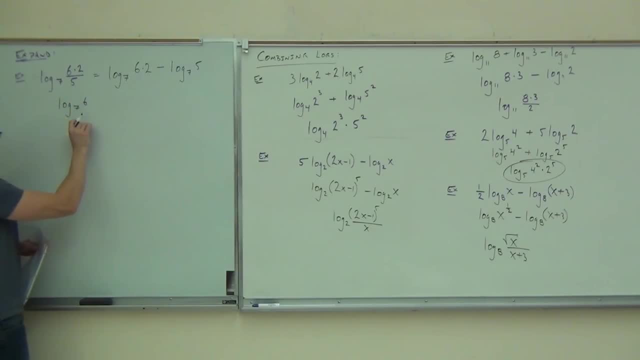 and you can do that. So all-in-all this is going to be log base 7 of 6 times 2 over 5, so that's how we split up by that subtraction. Are you guys okay with that? so far, That's as far as you could go. 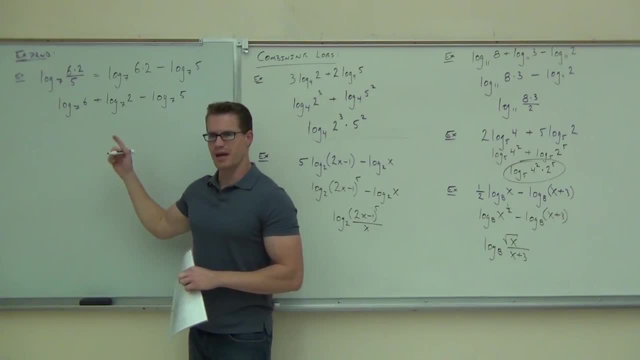 You got it right with that. Now, at this point, you'd be checking for any exponents you could move forward. Notice that you don't move exponents forward until you get down to this step: Expand all your product rule, your quotient rule and then your exponents. 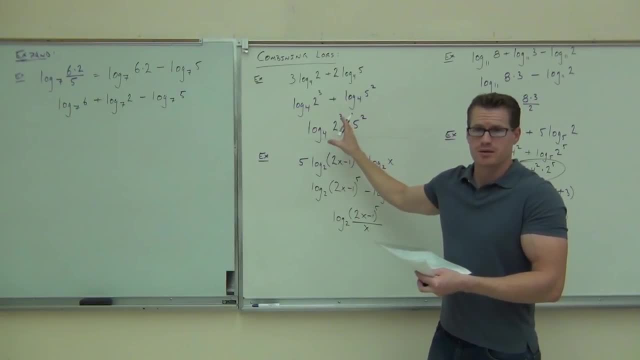 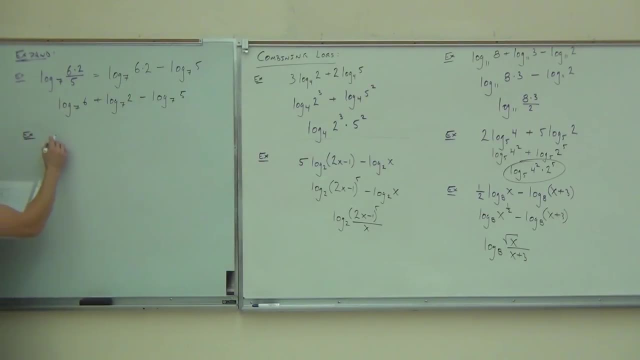 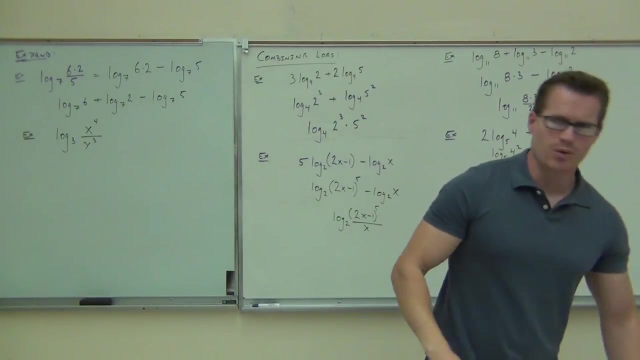 You're going backwards of combining. The first thing you did here was exponents, right, It means the last thing you're going to do over here is exponents. So we're kind of working from the outside in First things first. could you move your exponents forward? 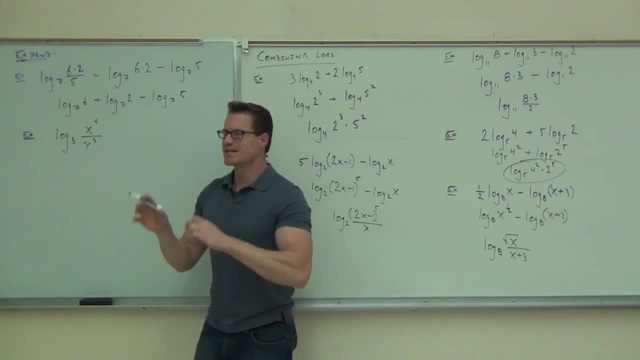 Is that appropriate to do At this particular step? Not until it looks exactly like those properties I gave you. and it doesn't look like that right now. Right now it looks just like a quotient. So the first thing you'd have to do here is break up that quotient. 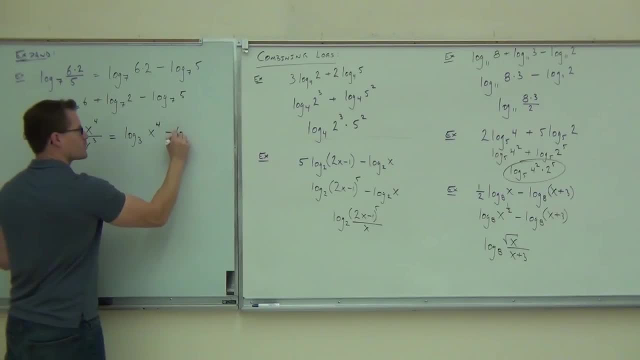 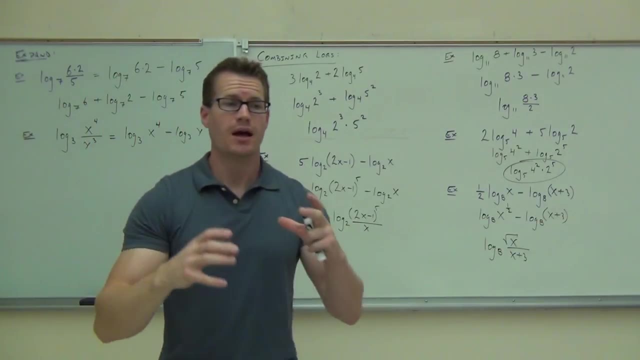 That's log base 3 of x to the fourth, minus log base 3 of y to the third. That's the first thing you have to do: work from the outside in. Now each one looks like one of those power properties. Now it looks okay. 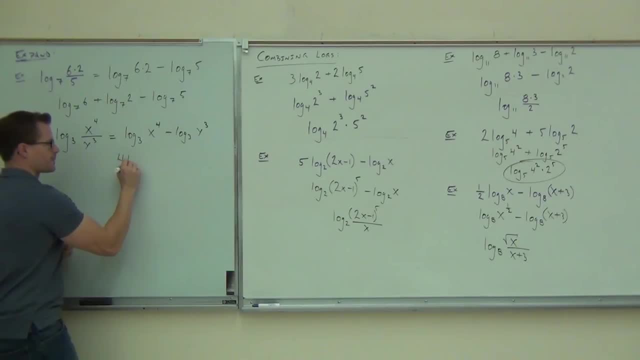 Now we move our exponents to the front, We'll get 4. log base 3 of x minus 3 log base 3 of y. I should give these a try, Very, very similar Try, that one and this one. 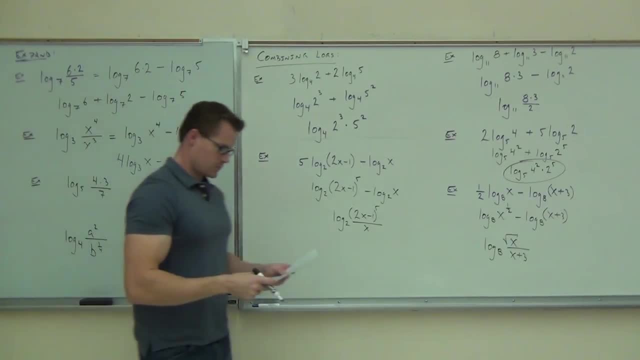 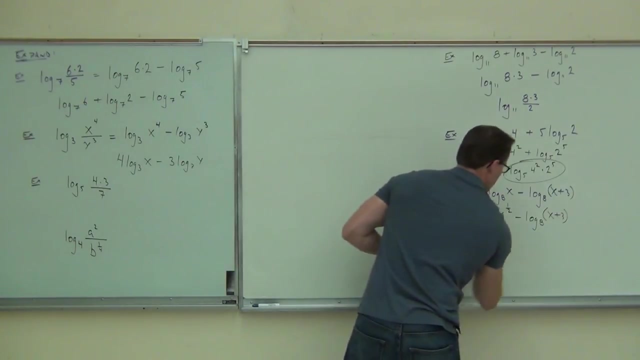 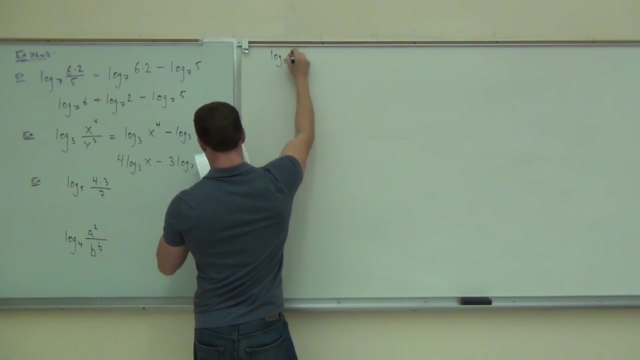 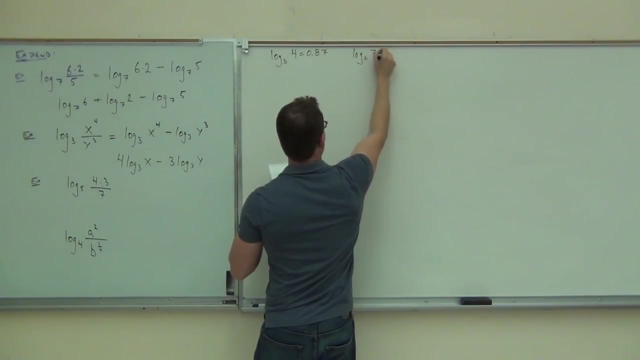 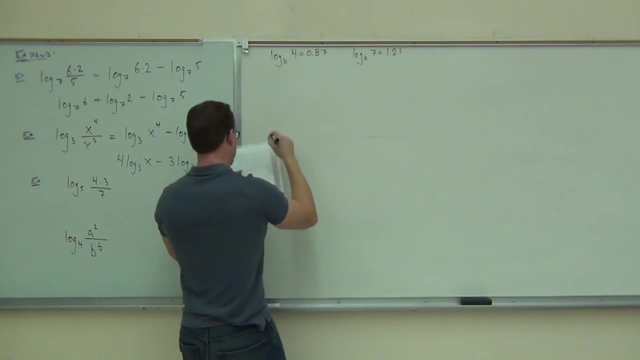 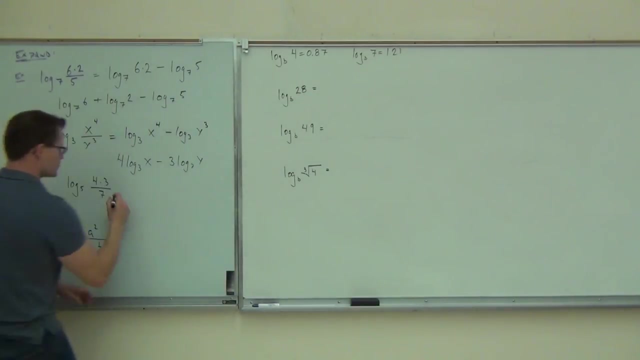 All right, All right, All right. Okay, We're running out of time here, so I've got to just do these for you. Log base 5 of 4 times 3 over 7, you split up your subtraction first. 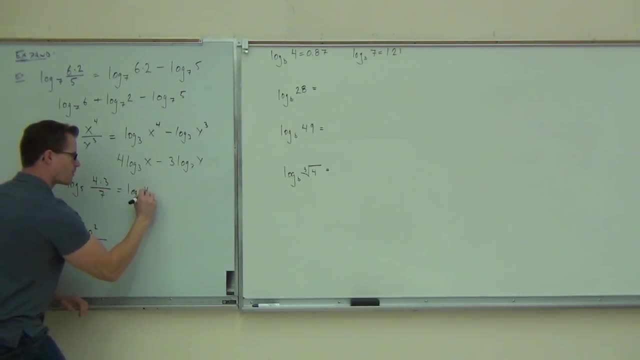 and you split up your addition, This answer is log base 5 of 4 plus log base 5 of 3, minus log base 5 of 7.. Did you get that one as well? Yeah, Okay, Next one: Okay. 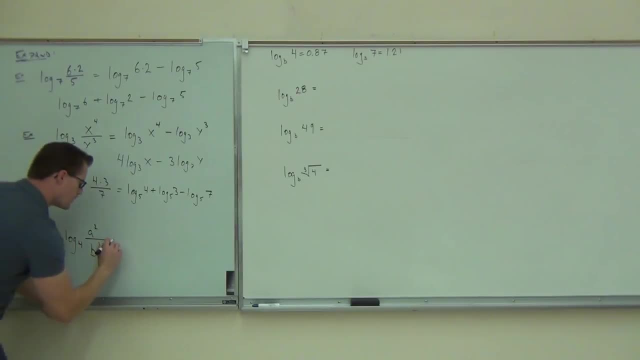 So we first have to split up our subtraction and then move our exponents forward. This is going to be 2 log base 4 of a minus 1 to the 4th log base 4 of b. That's as far as you can go on those ones. 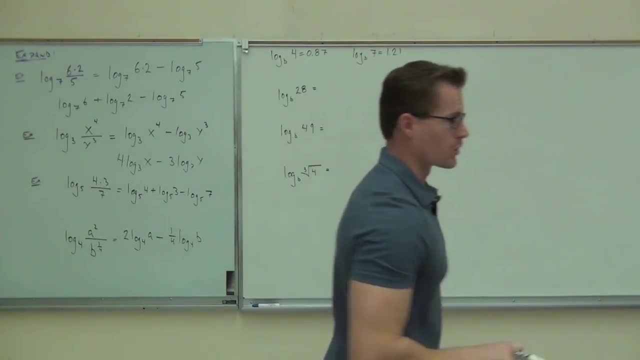 How many of you got those two? Okay, Last thing that's going to really help you out in your homework. This is it. I know we're about a minute over right now. Let's suppose that you only know two logarithms in the world. 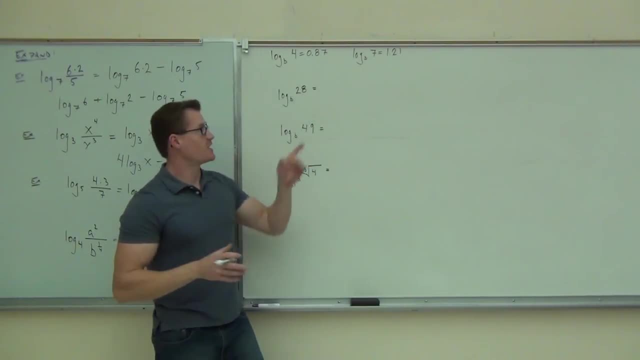 These are it? What the idea of these problems is is, if you don't know the base, you have to know what these. are These values equal? So it's given that to you, The idea is write these as some combination of those logarithms. 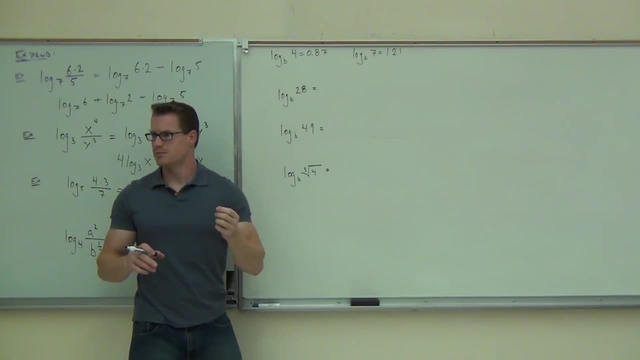 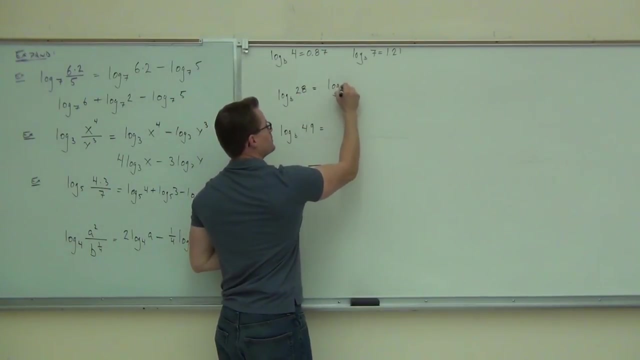 For instance, 28 is 4 times 7.. Do you get me? Why am I thinking 4 times 7,, not 12 times 2?? Well, all I know is 4 and 7.. So this would be log base b of 4 times 7.. 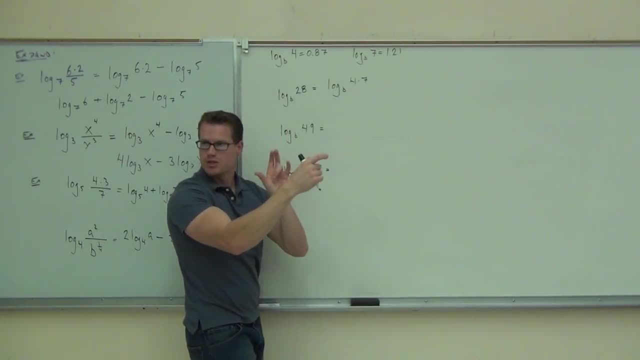 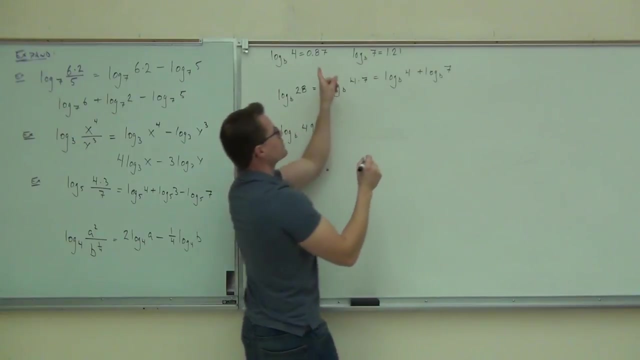 True, That's 28.. You can split up that multiplication now. This is log base b of 4 plus log base b of 7.. And then you can substitute those numbers in. Are you with me on that? Yes, no. 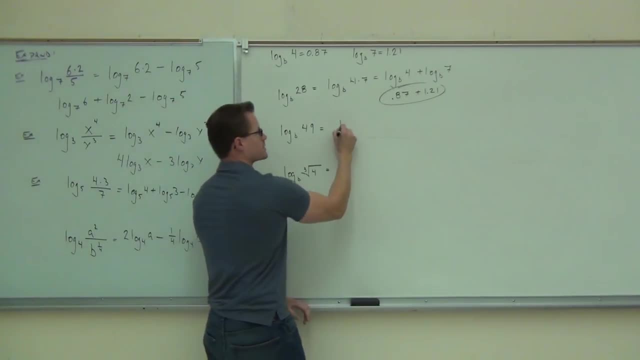 And then add those. Same thing for this one. This is log base b of 7 squared. Write 49 as 7 squared. Write them as one of these things. That's an exponent. It can move to the front. 2 log base b of 7.. 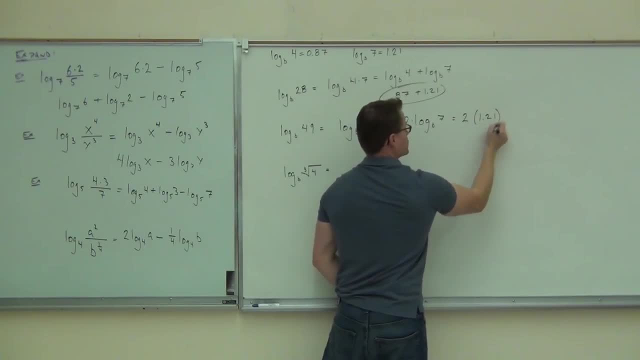 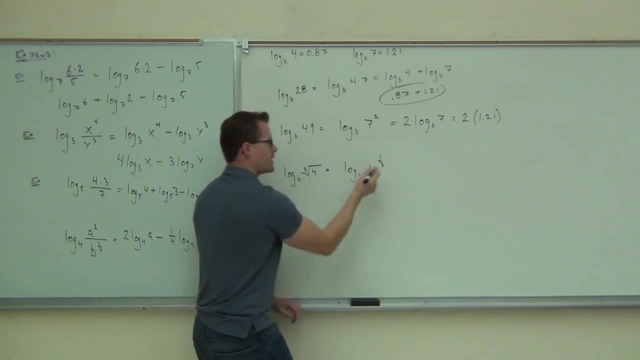 Or that would be 2. 2 times 1.21.. Last, one log base b of 4 to the 1 third. That's an exponent. It can move to the front. 1 third log base b of 4.. 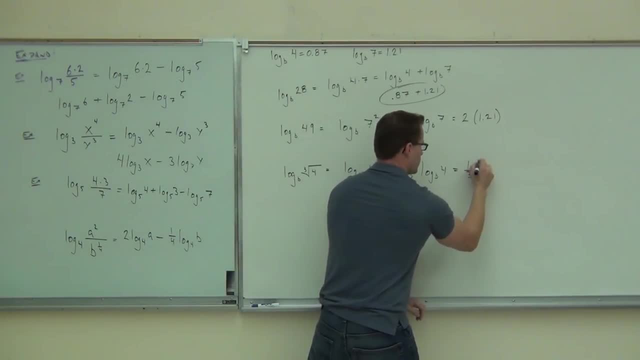 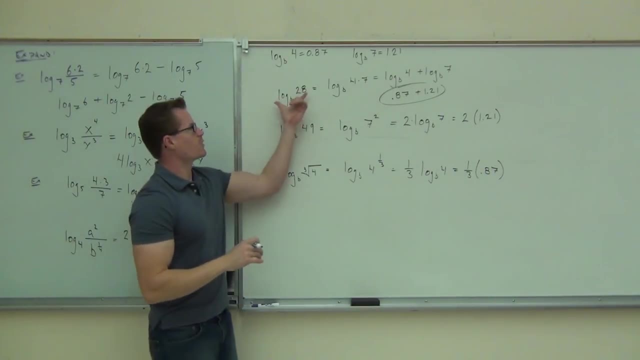 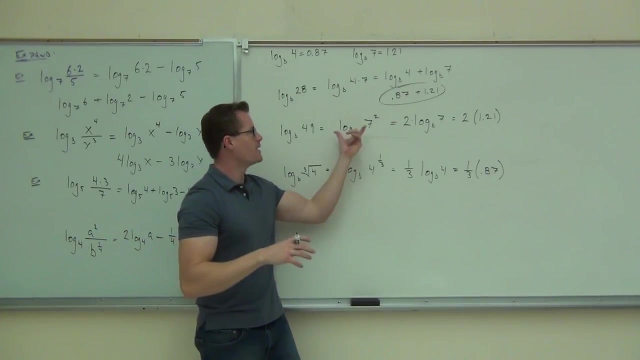 Log base b of 4 is 0.87.. That's the idea. So when you get down to the last few problems, try to write whatever these are as the two logarithms that are given to you, Some combination of those, Then use the expansion properties to write them. 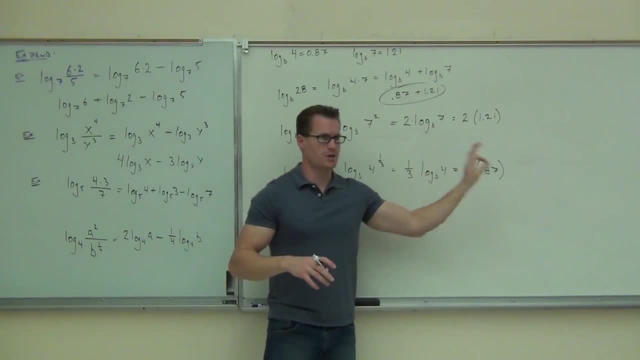 until you get them into an individual form and then substitute in those values.